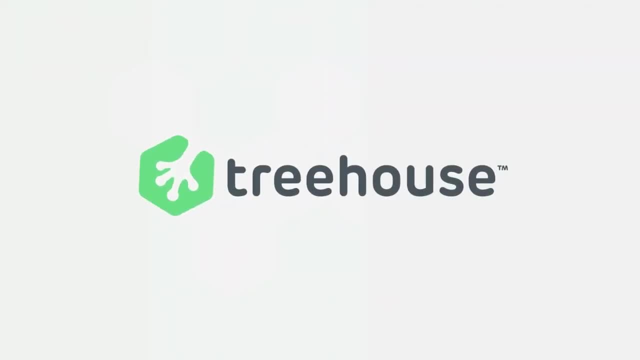 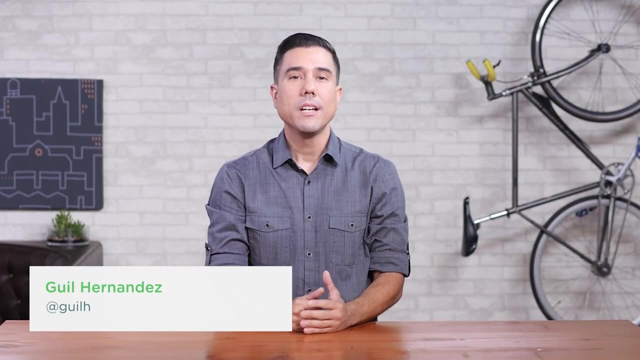 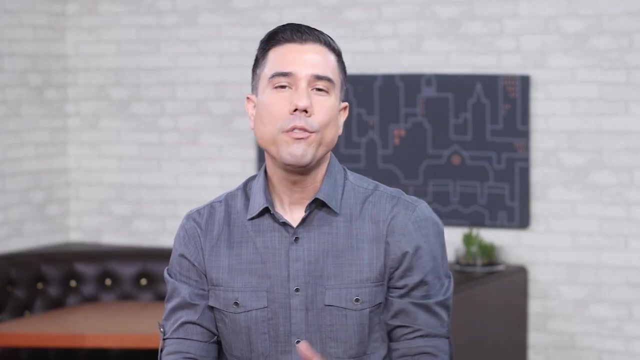 Hi everyone. Gil here, a developer and JavaScript instructor at Treehouse, I'm happy that you've joined me here to continue your JavaScript learning journey. So far, you've explored many of the key concepts and features of the JavaScript language. You're getting more familiar. 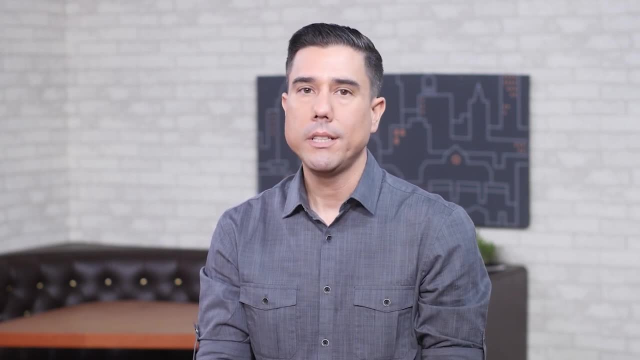 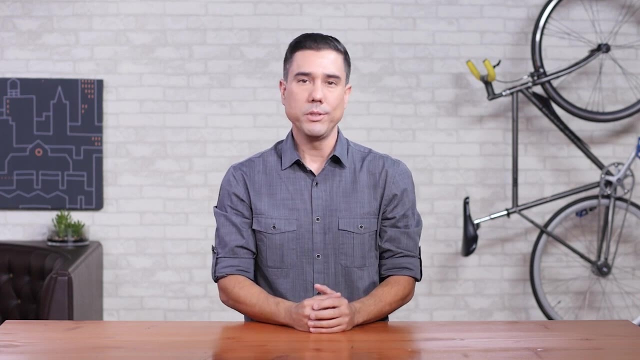 with the syntax, as well as working with variables, built-in data types and objects and conditional statements. In this course, you'll continue to build your JavaScript skills by learning another fundamental building block in JavaScript: functions. Functions are at the heart of how 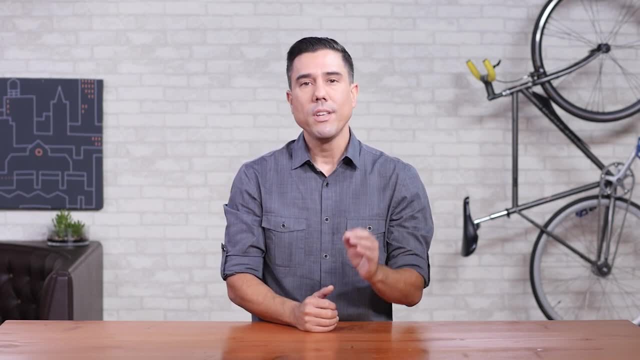 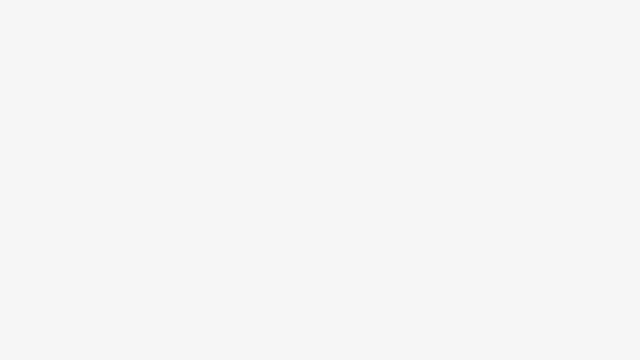 JavaScript or any programming language works At its simplest. a function is a set of instructions that you want to run over and over again. For example, imagine that one magical morning an assistant showed up to take care of some of the tasks that take up extra time in your 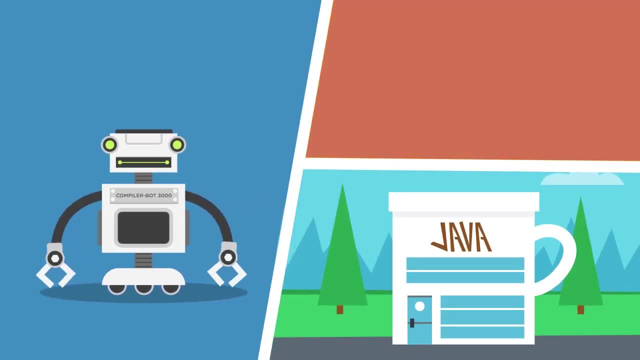 day. One of those tasks is getting coffee from your favorite coffee shop that's a few blocks away. It's your assistant's first day, so you provide them detailed instructions on how to get to the coffee shop and what drink to order. Keep in mind that your assistant 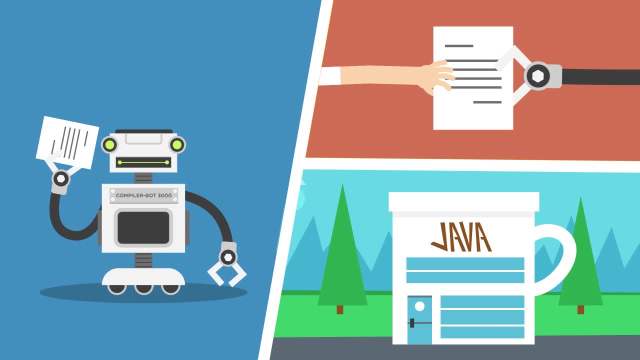 doesn't actually get you anything yet, they just keep the instructions in memory. A little bit later in the day, at around the time you usually go out to get coffee, you say to your assistant: go to the coffee shop and your assistant very kindly goes off to get you. 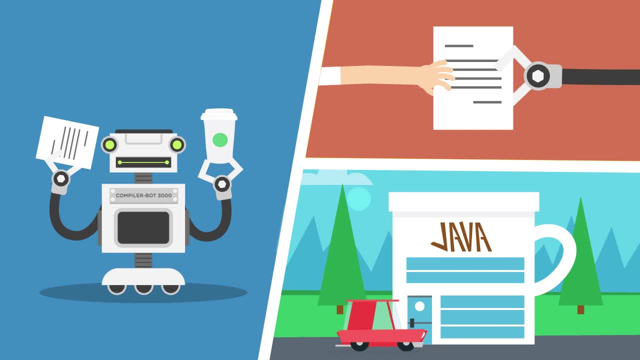 your coffee. Since you already gave your assistant instructions earlier, you don't have to tell them how to get to the coffee shop or even what to order. From then on, anytime you want coffee, you can just say: go to the coffee shop and your assistant returns with your. 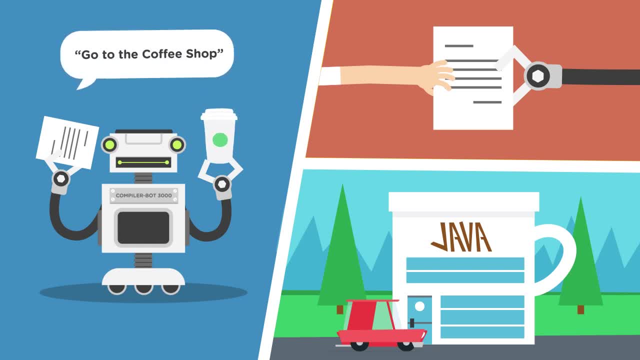 drink. In fact, you can say, go to the coffee shop over and over again and each time you'll get a new cup of coffee Later that day. you might even provide your assistant different sets of instructions for, say, doing the laundry, washing dishes or feeding the cat To get. 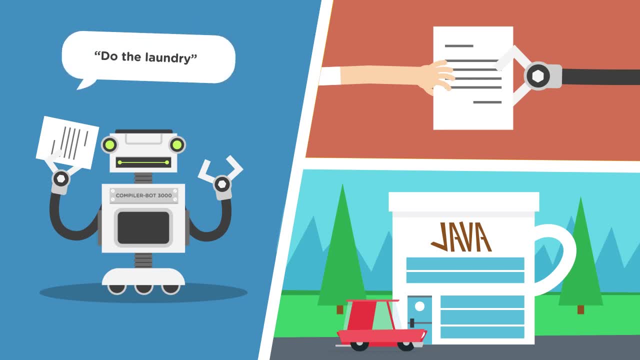 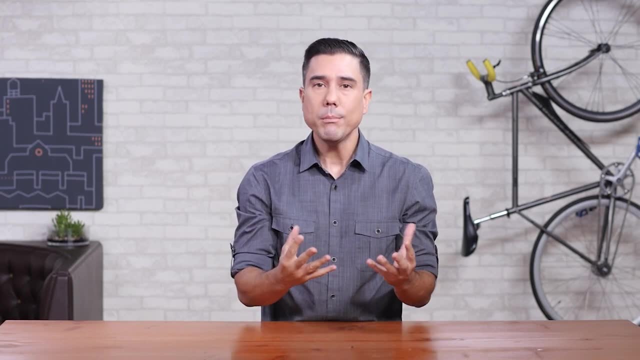 a task done. you just call out a command like: do the laundry. Okay, now let's get back to reality. Functions work in much the same way. They let you group a series of statements or instructions together to perform a specific task needed by the program. Let's get into how they work. 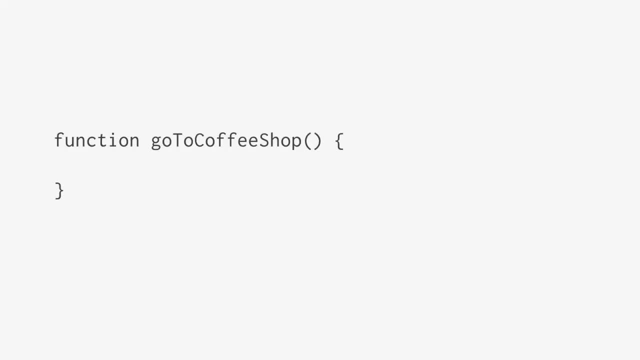 You start by declaring the function. That's like you providing instructions to your assistant. In JavaScript, you use the function keyword, followed by a name for the function, a pair of parentheses and a pair of curly braces. You can name your functions whatever you'd. 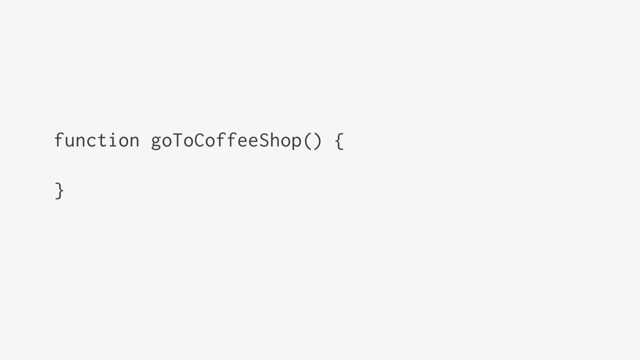 like, as long as you follow the same rules for naming variables. For example, if you call function, names can only be made up of letters, numbers, the underscore and dollar sign characters, But they can't start with a number and you can't use spaces or other. 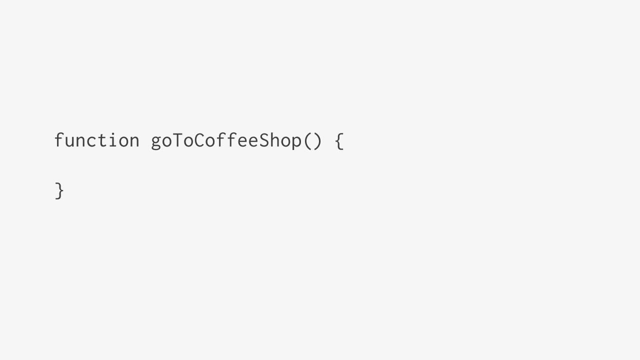 punctuation in the name. Following the name, you place a set of parentheses. This is one way you can identify functions. Whenever you see parentheses following a name, you know you're dealing with a function. After the parentheses comes a pair of curly braces. 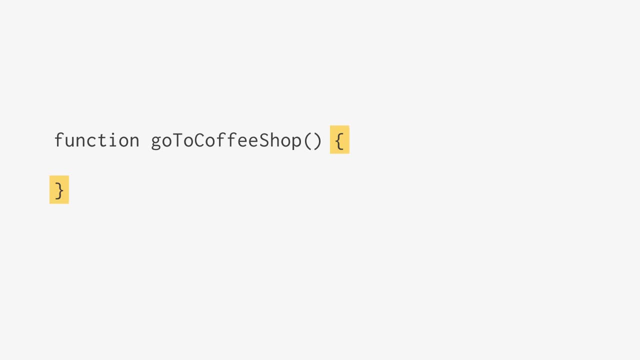 which form a code block. You learn about code blocks in an earlier course when you wrote conditional statements, For instance. if you wrote conditional statements, you'd have to write a conditional statement. In a conditional statement, you'd use curly braces to create. 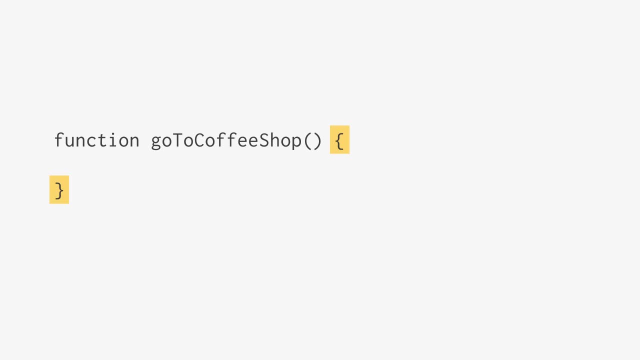 a block of code that runs when a condition is true, Also like a conditional statement. there's no semicolon after the final brace. Don't worry about the details, Just remember to leave off a semicolon after the final brace In a function. the JavaScript you place inside the curly braces runs whenever the program. 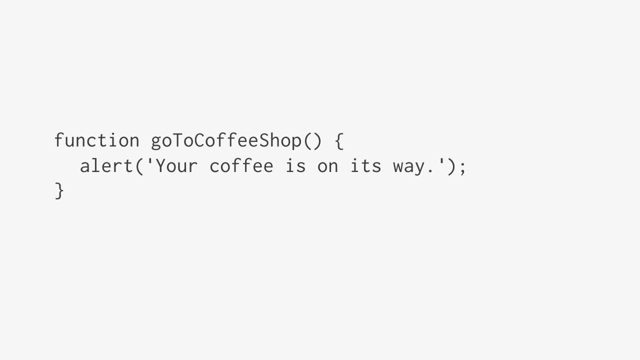 activates the function. To activate the programming inside a function, you call the function, which is just like you saying: go to the coffee shop, to your assistant, To call a function and run the code inside of it. you write the name of the function. 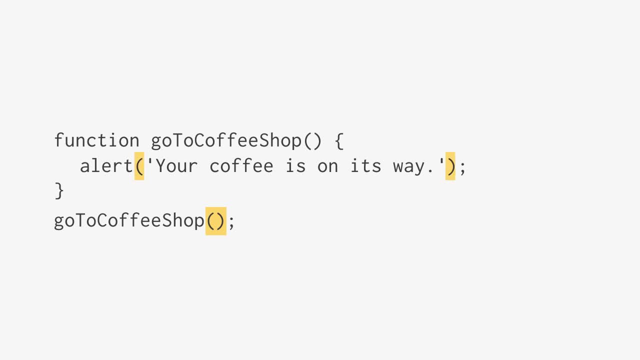 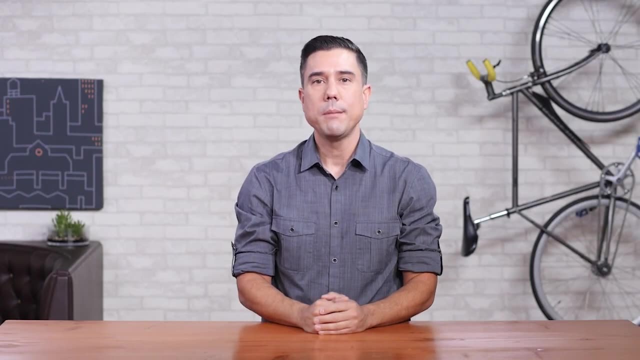 followed by a set of parentheses. The parentheses are important. They call the function and activate its programming. When programming, you'll often need to perform the same tasks in different places of the program. For example, check if a user correctly filled out a form. 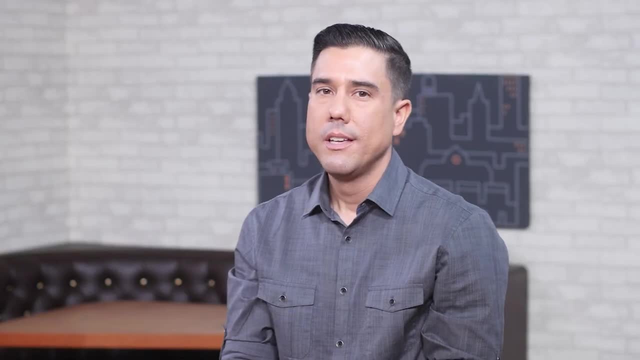 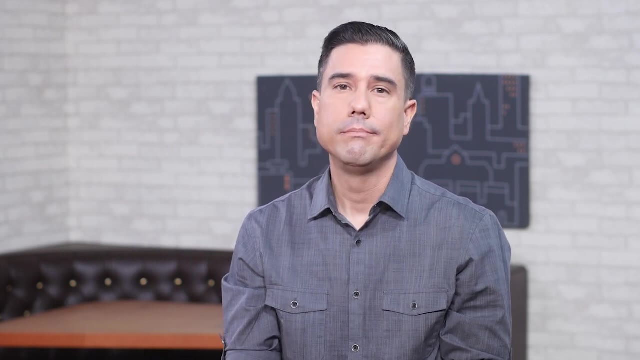 field or display a specific message to the user. Imagine having to repeat or re-type the instructions for a task everywhere you needed them. That would make your code messy and unwieldy. Functions provide a way to efficiently execute code that you want to. 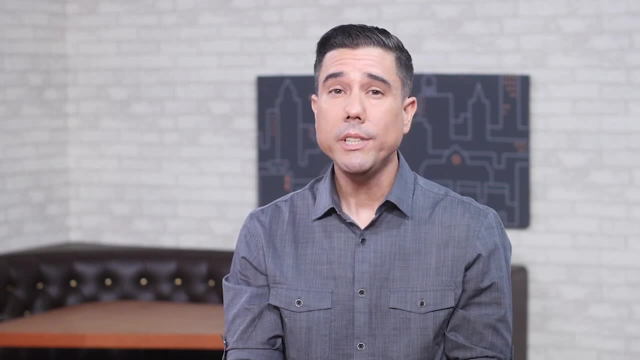 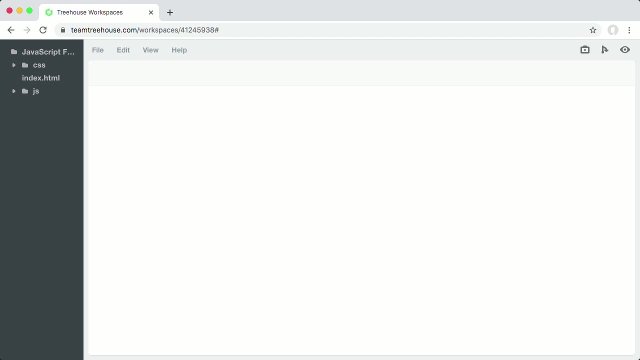 repeat again and again. Then you can call that code whenever you need it using a single short command. Now that you've learned the basics of functions, it's time to create a function You can code along with me. by launching the workspace with this video: Open the file named. 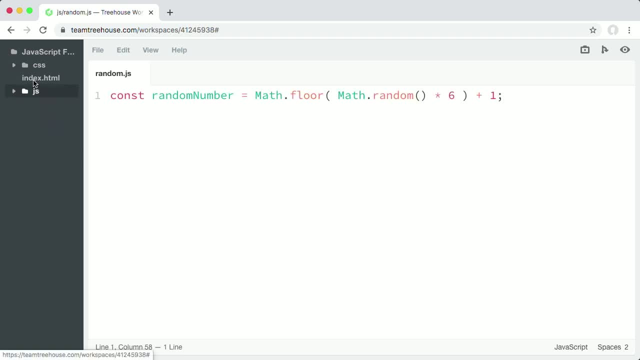 randomjs located inside the js folder. This file is already linked to indexhtml. You'll see that the file already has a single line of code. You've seen this code before in a previous course on JavaScript numbers. This code creates a random number from one to six and stores it in a variable. 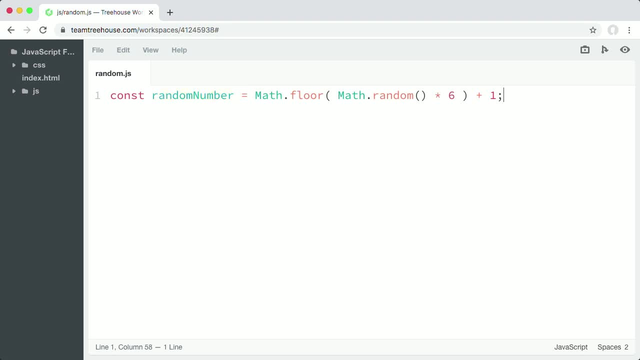 named random number. Functions are just about everywhere in JavaScript. In fact, we've used lots of functions so far. For instance, notice the parentheses after mathfloor and mathrandom. Mathfloor and mathrandom are also functions. They're functions that are built into the 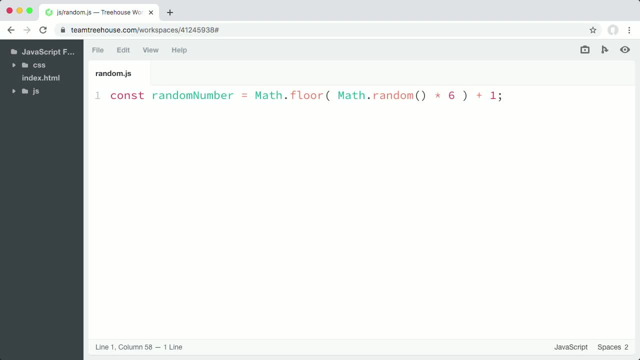 JavaScript language. They're not just functions that are built into the JavaScript language. You can also create your own functions to perform just about any task you want. In this case, let's create a function that displays an alert dialog box with a new random number in it each. 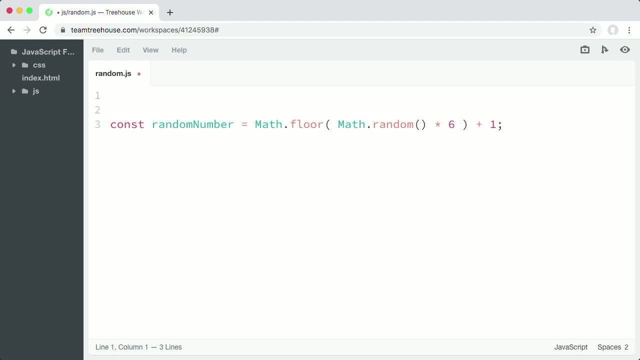 time it's called. First, create a function named alertrandom with function alertrandom, followed by a set of parentheses and a set of curly braces. I'm writing the function at the top of a file. Remember, the code in the function does not run immediately. JavaScript creates a. 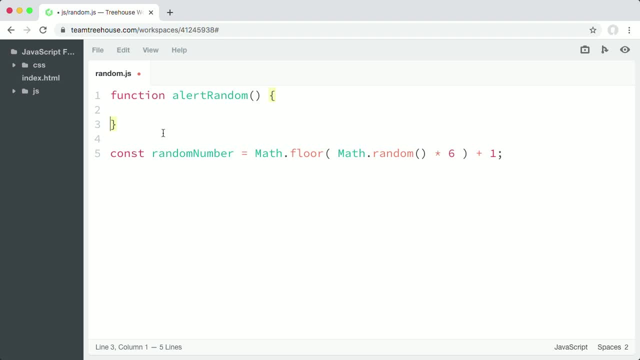 space in memory to save the function definition and assign it to the name alertrandom. similar to the assistant memorizing the directions to the coffee shop, I want to create a new random number each time I call this function, So next I'll move the random number generating code into the 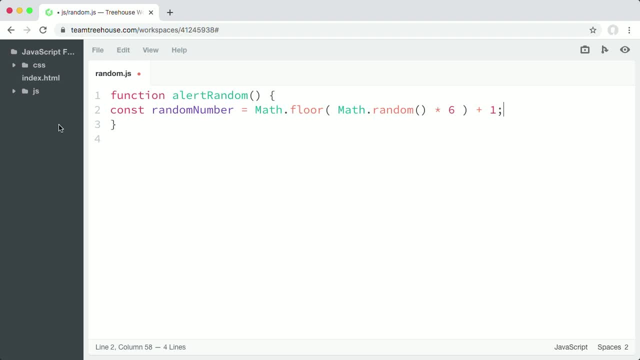 function And, just as with conditional statements, you should indent any code inside your function. This makes it easier to see that the code belongs to the function. Lastly, I'll display the random number using the alert method And look more parentheses. which means that alert is also a. 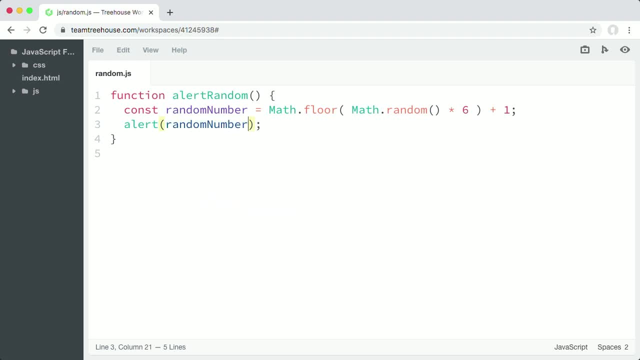 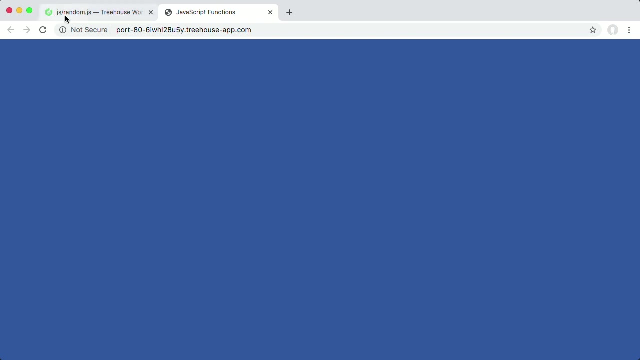 built-in JavaScript function. So now I have a small collection of code that does something. It has a function. I'll save this file and preview the workspace in the browser. Notice that nothing happens yet, But something did happen behind the scenes. The browser read the function into memory and it's now prepared to act on its instructions as 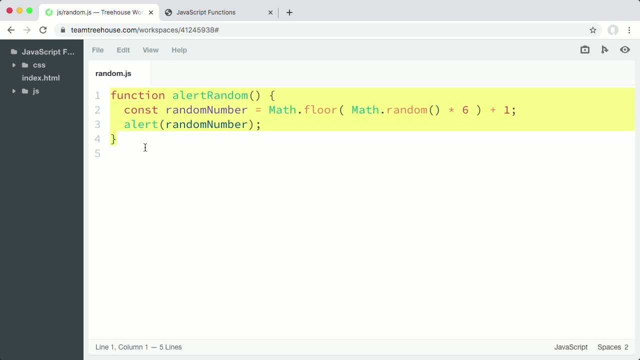 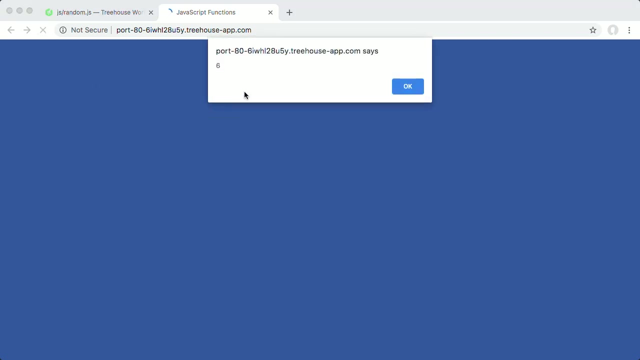 soon as it's called. It isn't until you call the function that its code runs. So in my JavaScript file I'll call the alert random function just below the function definition, like this: I'll save the file And when I refresh the browser a random number pops up. 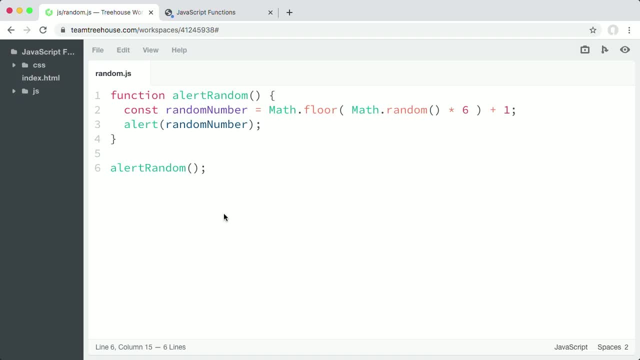 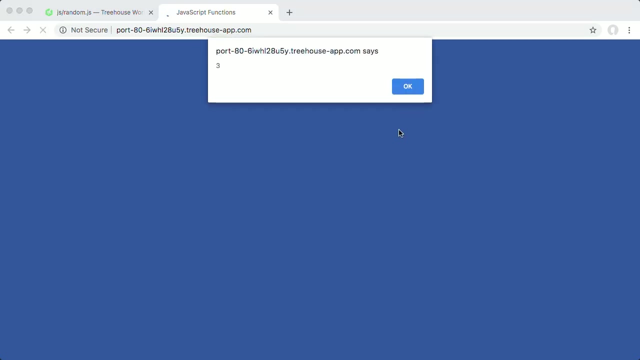 What's great about a function is that you can use it over and over and over again To run the function. call it. For example, I'll call alert random three more times In the browser. I get one random number, two random numbers, three random numbers. 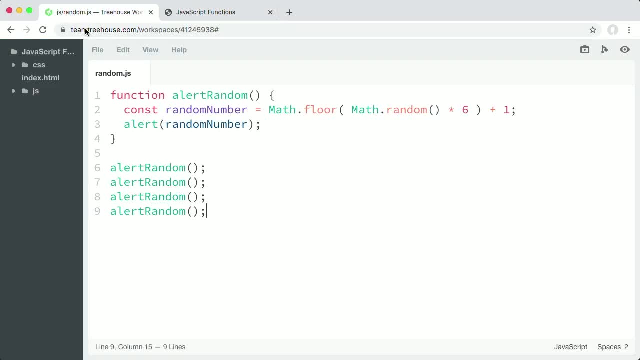 and four random numbers. So just one short line of code where I call the function triggers the browser to run multiple lines of code. Now imagine that you have a function with 50 lines of JavaScript. Calling that function using a single short command. 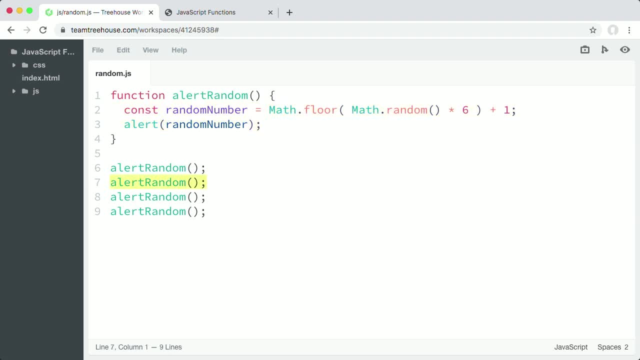 will run 50 lines of JavaScript. JavaScript functions are an invaluable tool in your programming toolkit, As you've learned. they let you run two, 10,, a dozen or hundreds of lines of programming by typing a single line of code. You'll use them constantly in JavaScript. 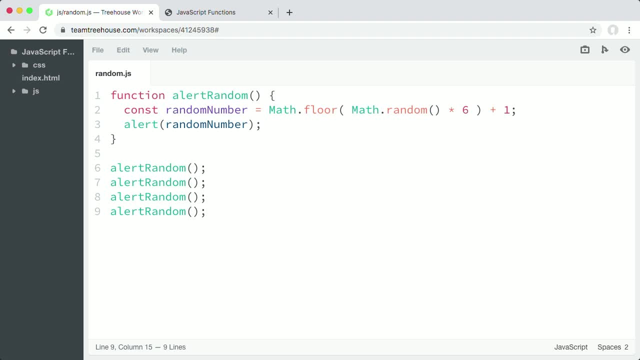 to make your programs more modular and easier to update. Functions also change the flow of your programs. For example, the JavaScript programs you've written so far start at the top of a file and run line by line. You learned in an earlier course that conditional statements can change the flow by doing some. 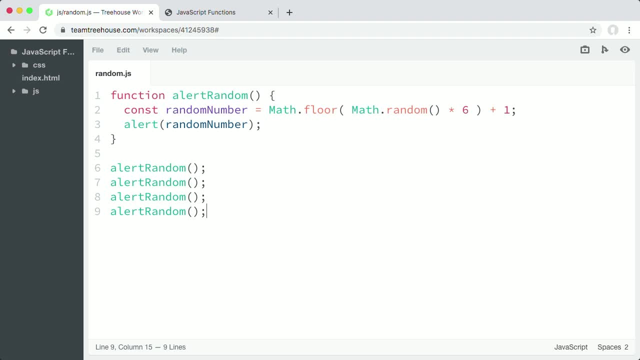 things based on one condition or other things based on another condition, But even then the program still ran from the top to the bottom of the file. It's just that the flow was sometimes diverted to different paths. Functions, however, break that top to bottom flow, For example. 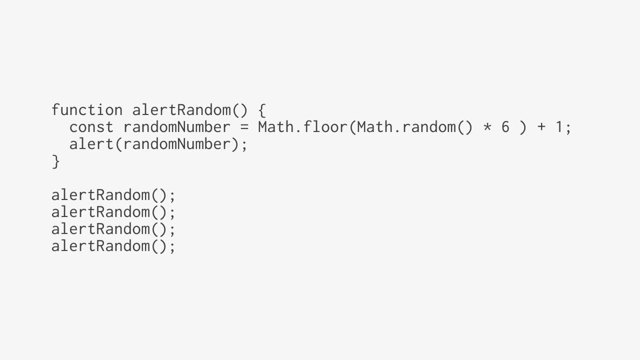 if you look at how the alert random function operates, you'll see that the JavaScript engine constantly jumps around. Each time you call the function, it's always running the same function. The JavaScript engine jumps into the function, runs the function's code then. 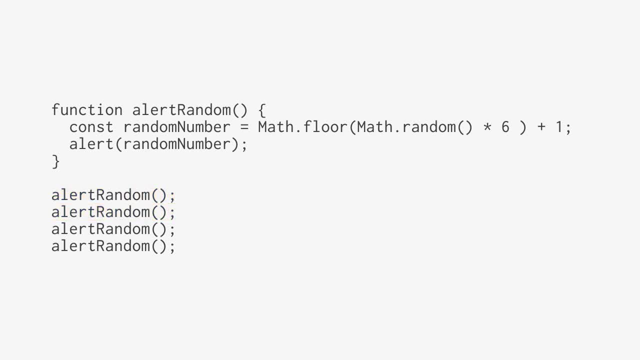 returns to the spot in the program where the function was called. In fact, in this code there are built-in JavaScript functions at work- mathfloor, mathrandom and alert- So when each of those are called, the JavaScript engine has to jump into them and execute their. 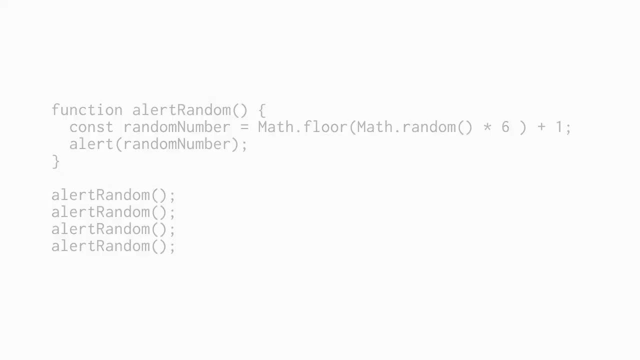 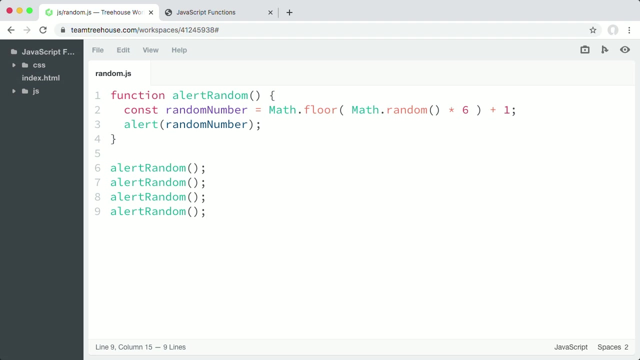 code then return to the spot it left off within the alert random function. You'll often need to perform a similar action in many places in your program. As you become a more advanced programmer, you'll need to perform a similar action in many places in your program. 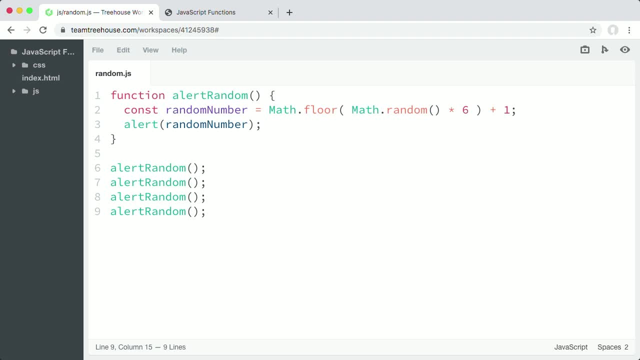 You'll write lots of functions to efficiently run code that you want to repeat again and again without having to type the same code multiple times. Up next we'll dig deeper into how to write and use functions. You're learning that functions are a way to run several lines of. 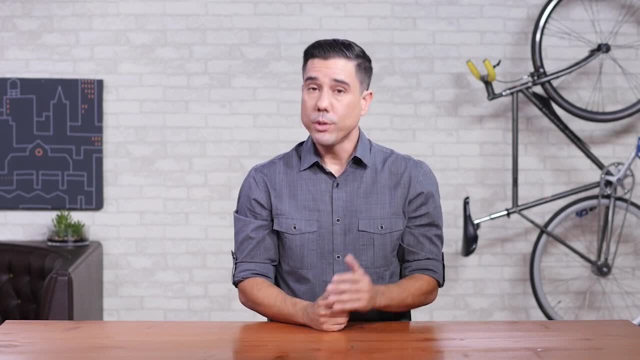 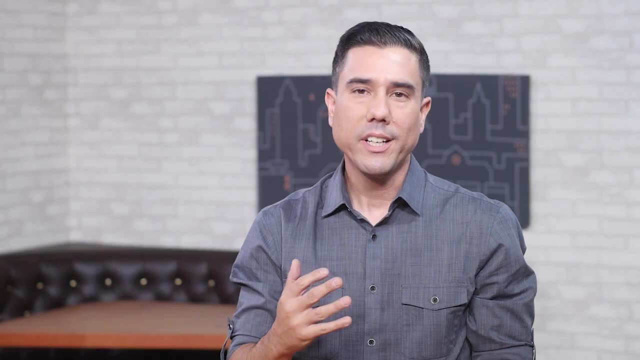 JavaScript code by issuing just a single command. When you call a function, you tell the JavaScript engine to jump to that function and run the code inside it. Remember back when you said, go to the coffee shop to your assistant. They dashed off to the coffee shop. 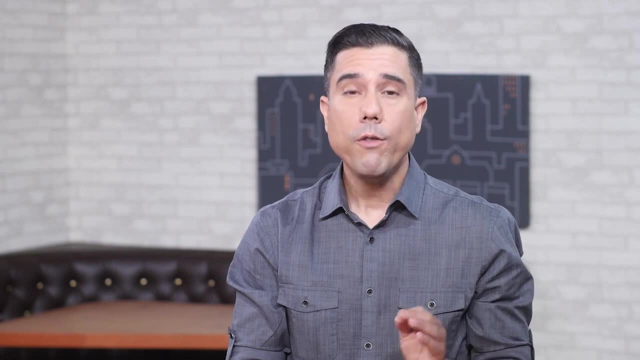 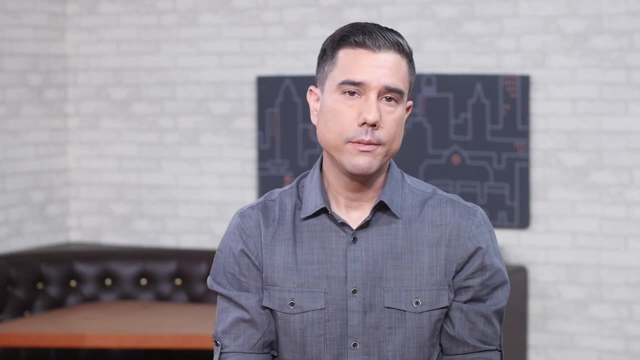 When your assistant returned, they handed you coffee. Well, functions can also give something back when they finish. This is called returning a value, and it's common when working with functions. For example, let's say you needed a way to get the current time so that you can display it on a 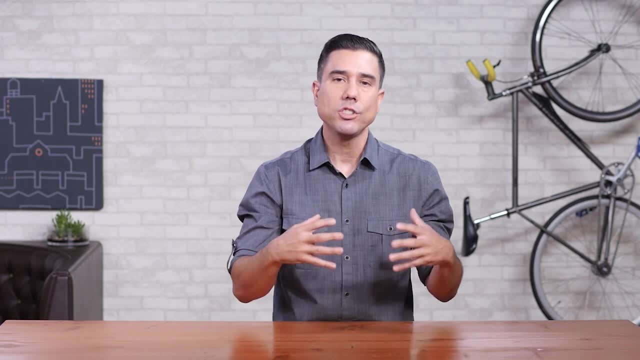 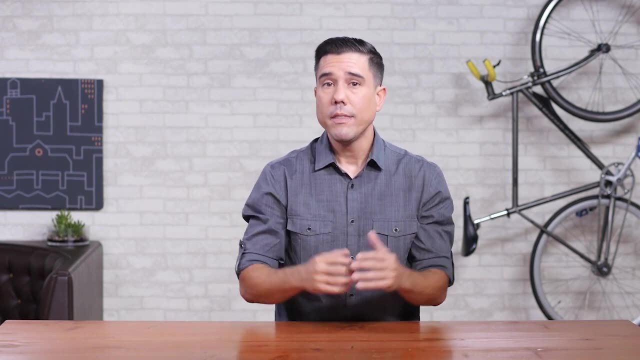 web page. You could create a function that gets the current time and actually writes it to the page. Better yet, you could create a function that just gets the time and gives it back to you. That way, you can not only write the return value to the page. 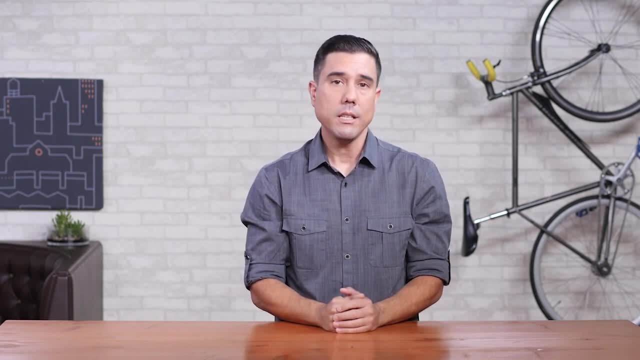 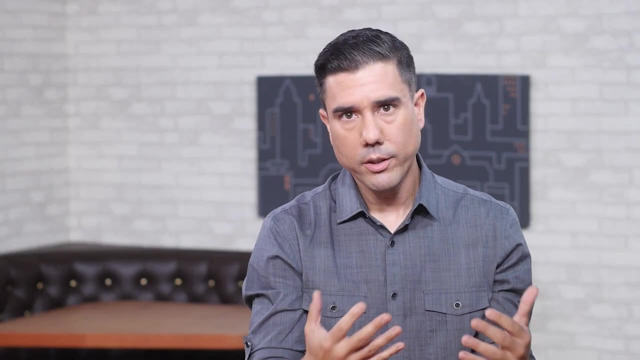 but you could also use the return value in other ways, like displaying it in an alert box or printing it to the console, In other words, creating a function that just does one thing: returns. the current time makes the function flexible enough that you. 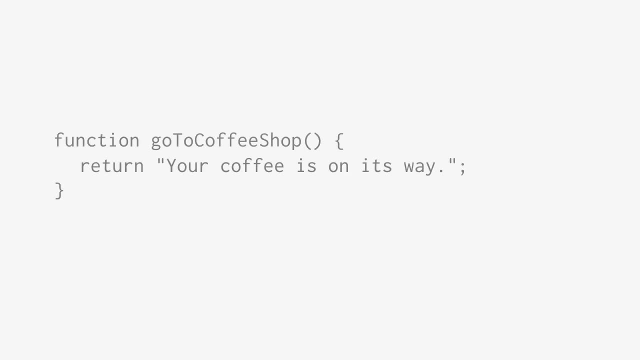 can use it in many different situations. To return a value from a function, you use the return keyword. This creates what's called a return statement. When the JavaScript engine or interpreter encounters the return keyword, it immediately jumps out of the current function. 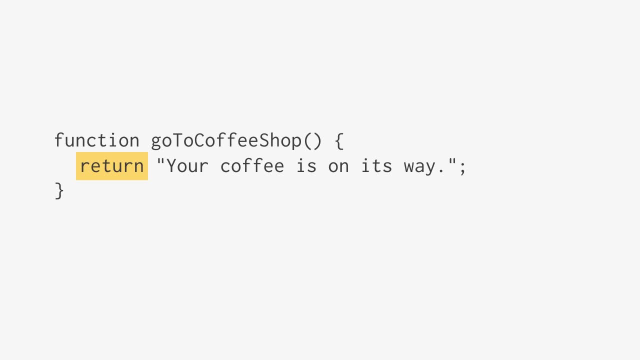 and provides the value to return. The value that's returned by the function can then be used in your program, For example, in this case, the return value is given to the alert function. So the message- your coffee- is on its way. 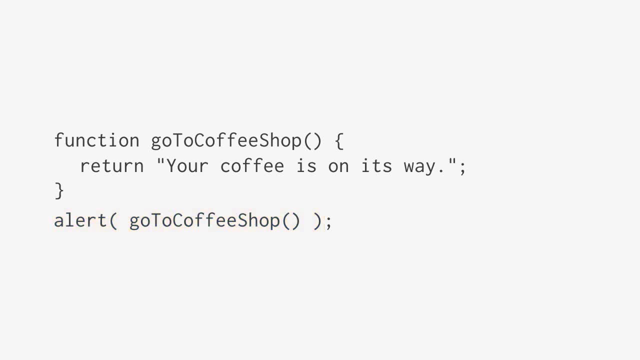 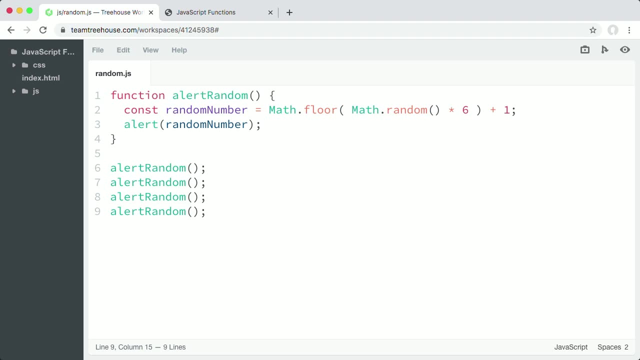 appears in an alert dialog box. But you could use this return value in many different ways: Print it to the console or even save it in a variable. Let's look at the alert random function we created earlier and see how we can improve it. 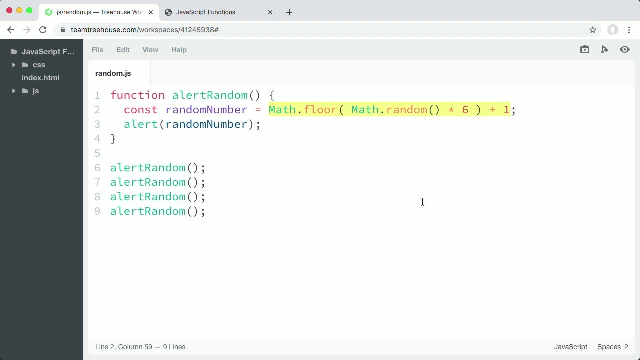 Generating a random number from one to six is useful. You can use it to build a dice rolling game, for example- But the function we created is limited. It generates a random number, but always displays it in an alert box. What if we wanted to show the random number on the page? 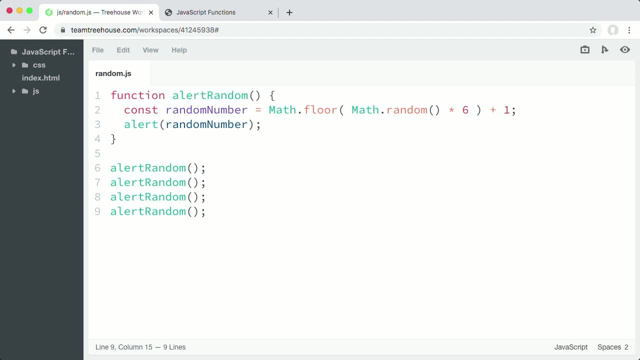 appear on the console or store it in a variable. We can make this function more useful by returning the random number. only That way we could use it any way we wanted to. I'll show you what I mean by first removing the alert method from the function. 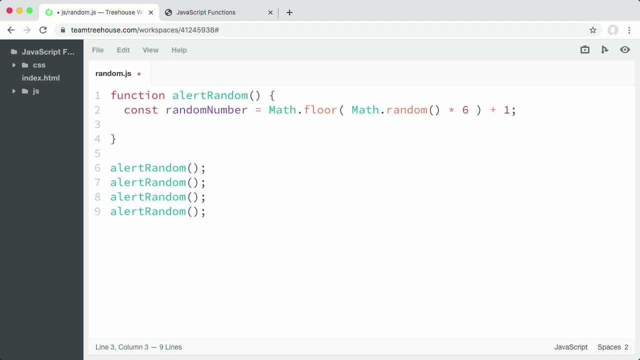 Next, I'll add a return statement to return a value from a function using the return keyword. And what do we want to return? Well, the value stored in random number. So now the function name alert- random- doesn't make a whole lot of sense. 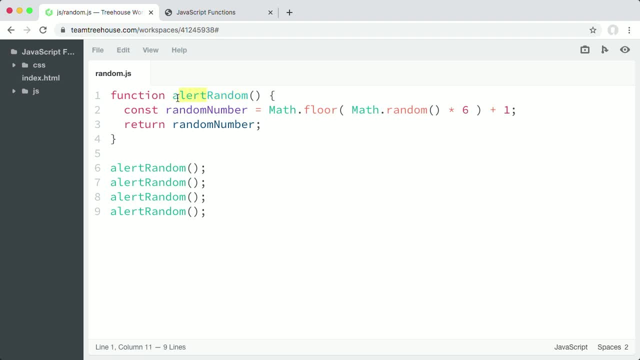 because the function no longer pops up an alert, So I'll change it to get random number, because that's what it's now doing. So now I can use this function anywhere. I want to get a number from one to six, For example in an alert dialog like this: 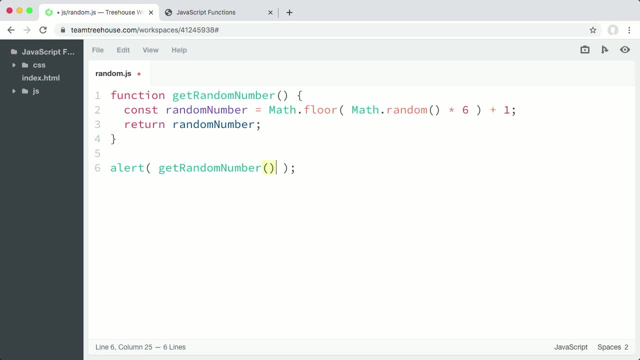 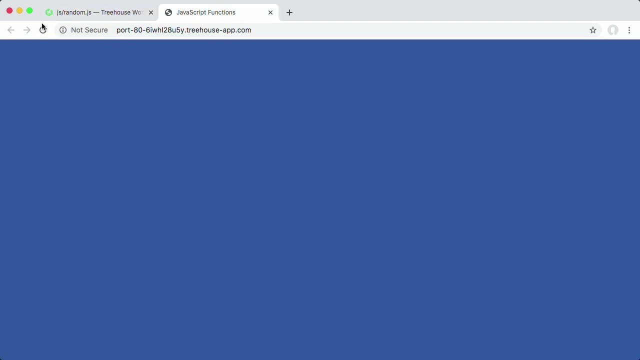 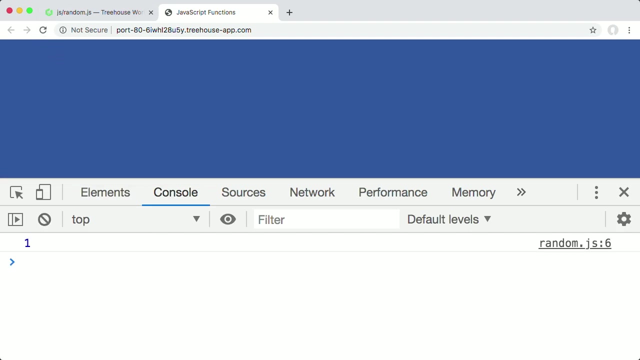 I can just print it to the console with the consolelog method. I can also print it to the console with the consolelog method. I can even store the function in a variable that I can use later, For example consolelog. So I'll copy that in here. 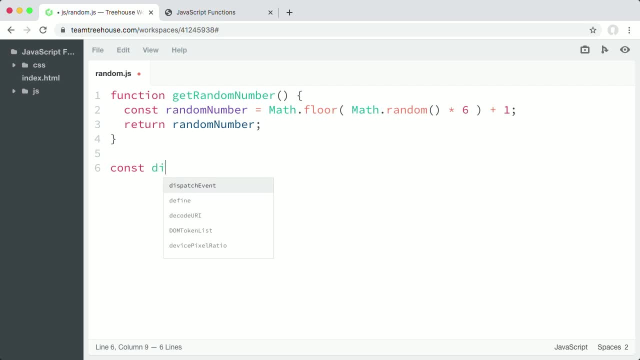 And now I can use it in a variable, And that's right. a function call itself can be a value that gets stored in a variable. Creating functions that only return a value is common in programming. For example, you might create a function that computes the total cost of an item, including tax and shipping. 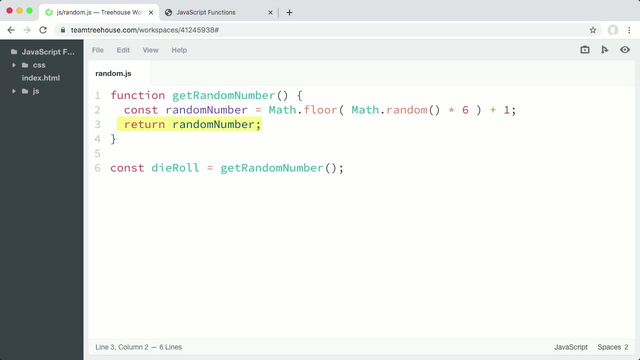 The function would return that total cost so that you can use it in other ways, like display it on the web page or use it for more calculations. Lastly, functions always return a value, even when they don't have a return statement. If you don't specify a return value, the function returns undefined. 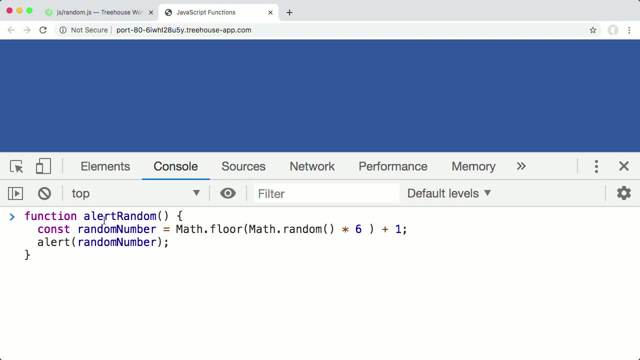 For example, in the console I'll paste the alert random function we first wrote, then call it. When I run this code, the browser pops up the alert and notice that undefined displays in the console. Undefined is one of JavaScript's built-in values. 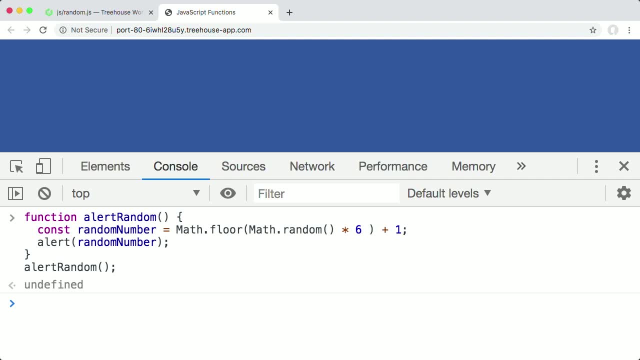 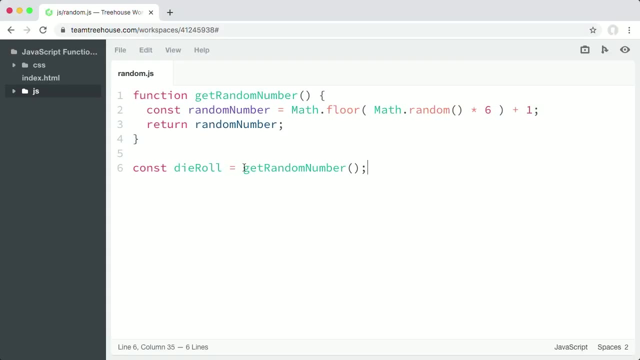 When returned by a function, it means that there's no return value specified. Now I'll call the getRandomNumber function here in the console And this time the console outputs a random number value. When you call a function, the JavaScript engine jumps into the function and goes through each of the steps defined inside its curly braces until it reaches the end or is instructed to stop with a return statement. 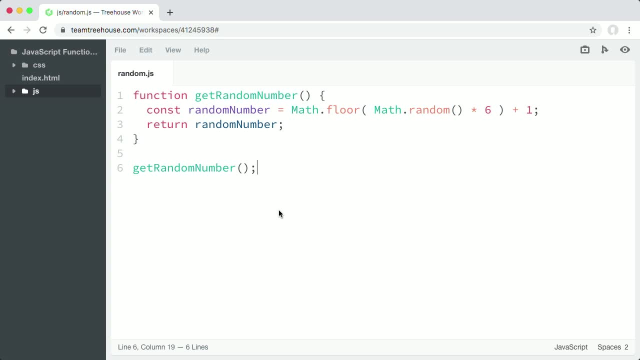 A function can have a return statement. For instance, you might create a function that checks if a form field is empty. In this case, the function could return either true or false. The function might check the field, then return just the value true if the form field hasn't been filled out by a user and is empty. 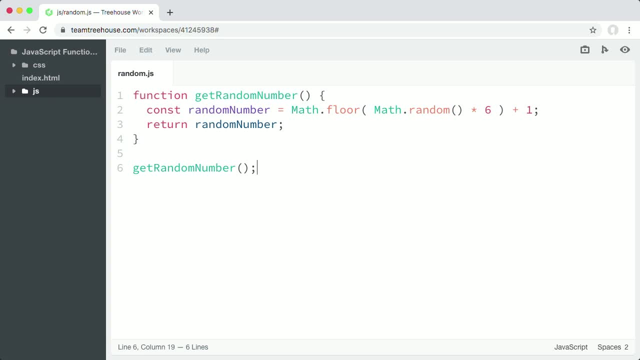 or it could return false. if the user did enter something, You can then use that return value to perform another action, like display an error message or prevent the form from being submitted. Let me show you one example. with code In your JS folder, open the file named multiple-returnsjs. 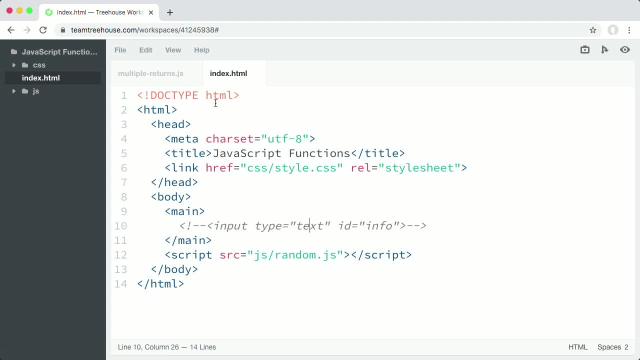 In indexhtml, update the script tag source attribute to js forward, slash multiple-returnsjs. In the JavaScript file, create a function named isFieldEmpty. This function will check if a form field for collecting a visitor's information is empty. In indexhtml there's an input element inside the main tags that's commented out. 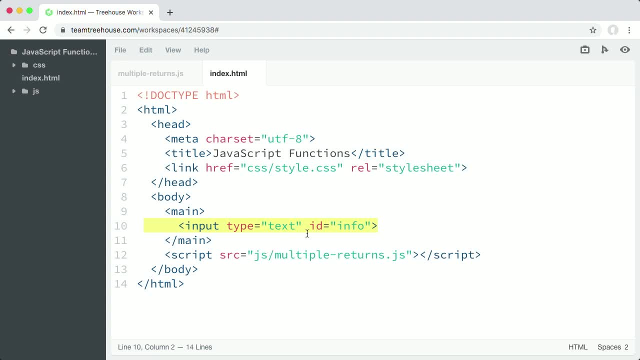 For this example. uncomment this code so that we're able to interact with it using JavaScript. The input element's ID attribute is set to info, so you can select this element with JavaScript using this ID. I'll save indexhtml and back in my JavaScript file. I'll first access the form field inside the function. 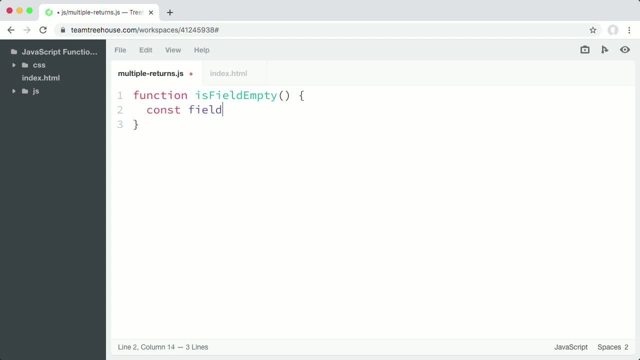 and store it in a variable named field With const field equals documentquerySelector And I'll pass documentquerySelector the string pound info. So this code accesses an element on the web page with an ID of info and stores a reference to that element in a variable named field. 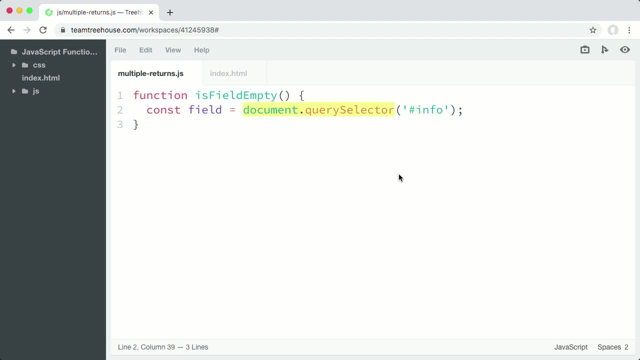 You've worked with documentquerySelector in a previous course, but don't worry too much about how this code works right now. You'll learn how to access elements in a web page like a form field in a later course. Once I have the field, I can test the value of it using a conditional statement. 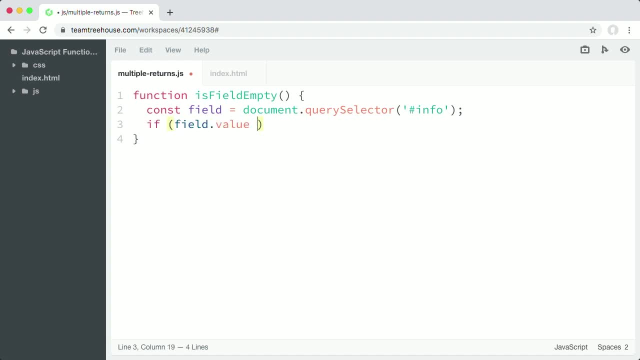 I'll start with. if fieldvalue strictly equals an empty string, return true. This tests the value of the field. In this case, I'm checking if the value is equal to an empty string. In other words, is the field empty? If the field is empty, then the function returns true. 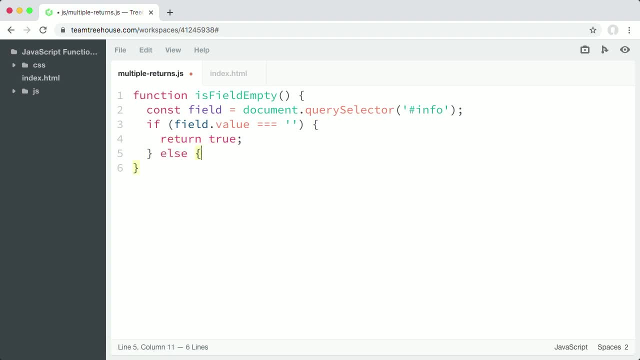 I can also use an else clause to return a different value. So now the function has two return statements, But remember that a conditional statement only follows one path. This function won't return both true and false. It will only ever run one of these return statements. 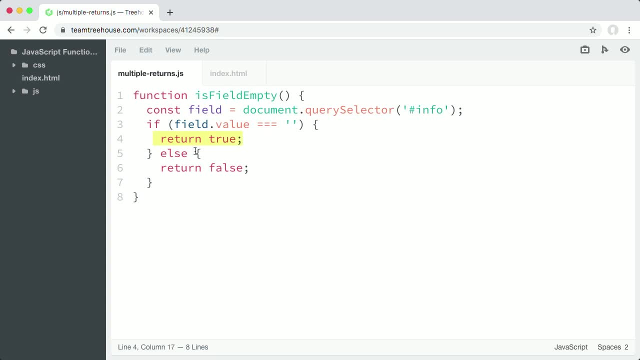 Either true if the field is empty, or false if it has something in it. I'll finish the programming for this by creating a variable named fieldTest to hold the return value from the function: Either true or false. Then use a conditional statement to see if the field is empty. 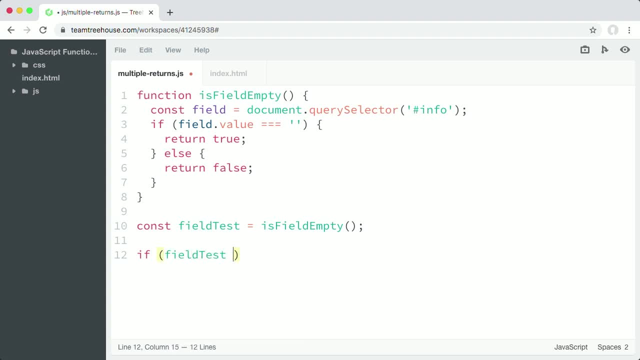 With if fieldTest strictly equals true. If it's empty, I can, for example, pop up an alert that says: please provide your information. I can test that this works by going back to my indexhtml file and adding a value attribute to the input element. 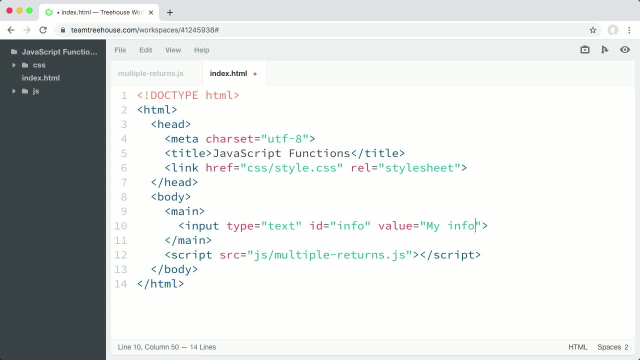 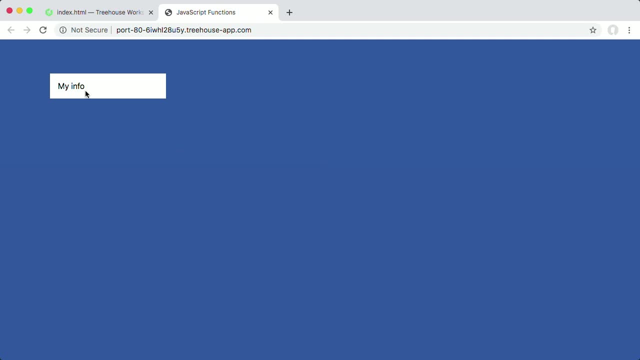 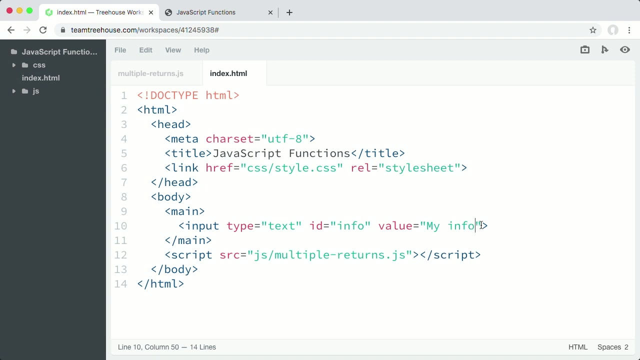 I'll set the value of the input field to minus MyInfo. I'll save indexhtml And over in the browser. since the input field is not empty, it has a value. nothing happens, However, if I remove the value attribute from the input element. now it's an empty field. 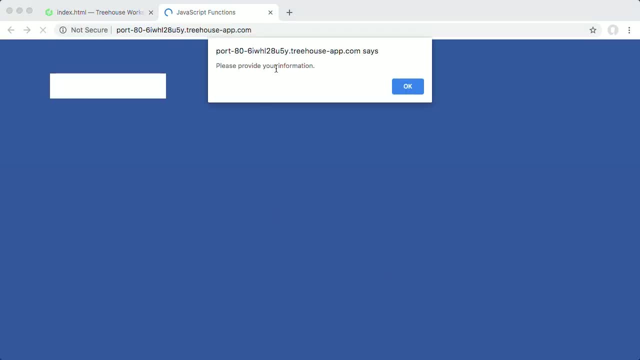 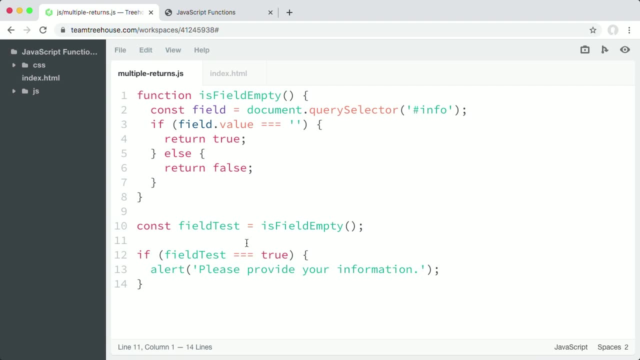 So an alert dialog pops up with a message. please provide your information. We can also simplify each condition. You know that all conditions evaluate to either true or false. true or false, the test condition produces a boolean value. So we don't need to use the strict equality operator in our conditions. For example, we can 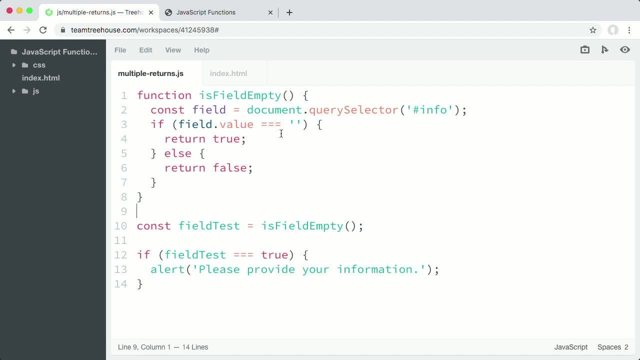 check if the value of the field is empty using the logical, not operator, like this: This checks if the field does not have a value. Also, since the value of field test is either true or false, we can check its value like: so: If field test is true. 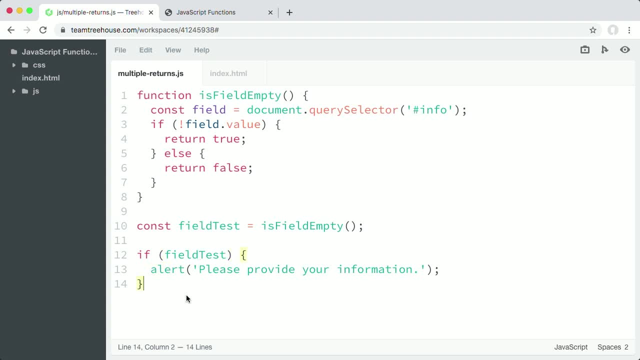 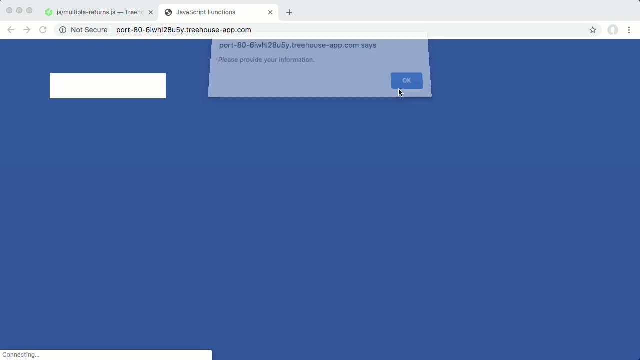 the alert will pop up. If it's false, nothing will happen. I'll save my file, refresh the page and everything should work just as before. Good, There are a few details to remember about the JavaScript return statement. When a return statement 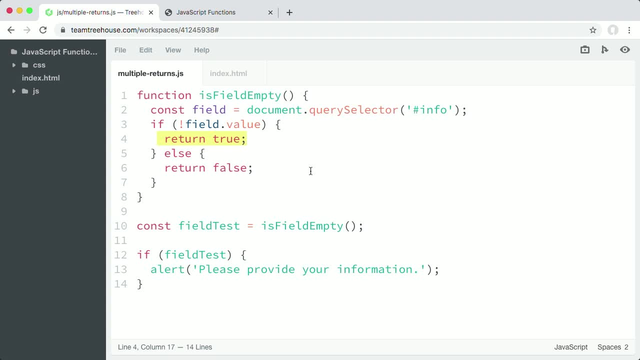 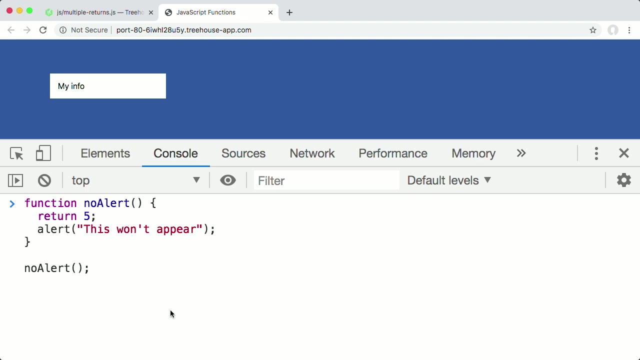 runs, it causes the JavaScript engine to exit the function immediately. In other words, the return statement should be the last line of code that you want to run in a function, For example over in the JavaScript console. let's follow the flow of some code. First, the JavaScript engine memorizes the steps in the no alert. 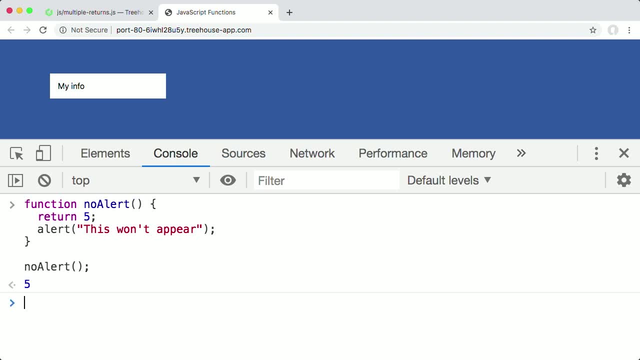 function. Then when we call the function, the program flow jumps into the function. When the return statement runs, it causes the JavaScript engine to exit the function immediately. In other words, the return statement is encountered, the function returns the number five. 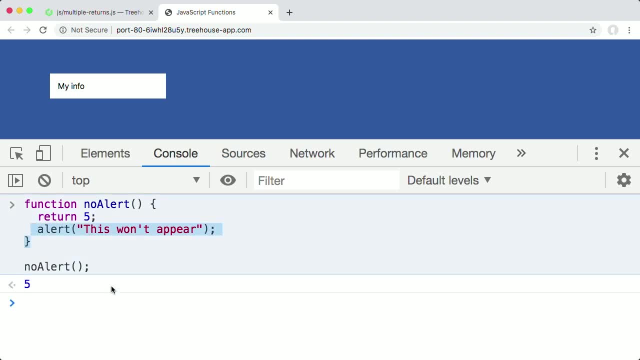 And the last line in the function never runs. Instead, control gets passed back to the main program. But notice that when I run the code again, this time adding an alert following the no alert function call, the alert outside of the function is the only one that runs. 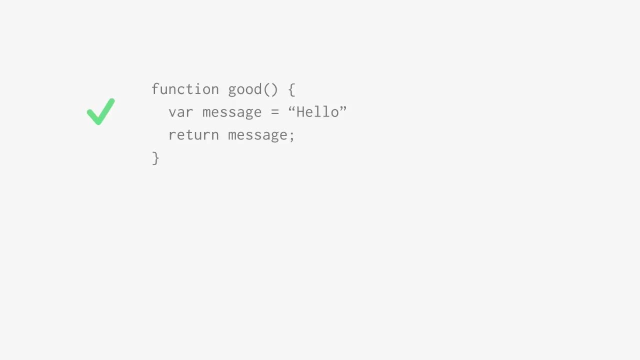 In addition, the return statement can only return a single value, That is, you can only return one thing: a string, a number, a Boolean value or the contents of a variable. Just keep in mind that you can't return multiple items at once. 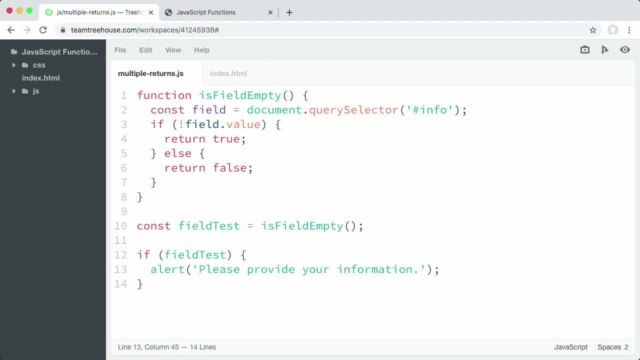 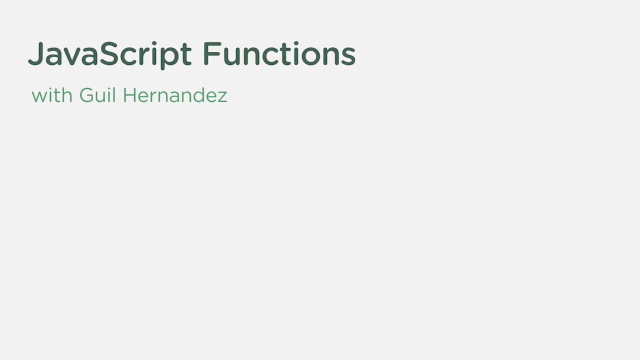 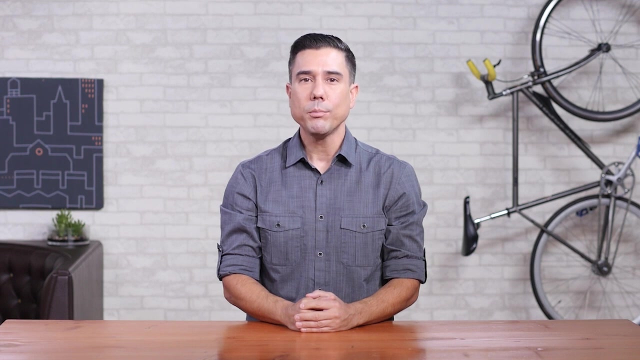 Just like you're able to get information back from a function, you can pass information into a function to change how that function works. I'll teach you how in the next stage. As you learned in the previous section, functions can return a value, But a function often needs. 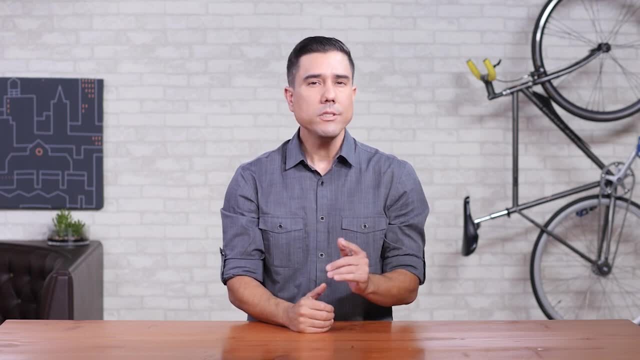 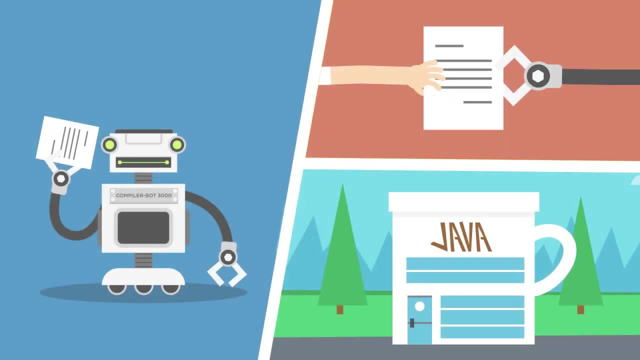 specific information to perform its task. In addition to getting information from a function, you can also send information to a function to change how that function works. Let's go back to the example of you and your magical assistant, Your go-to-the-coffee-shop. 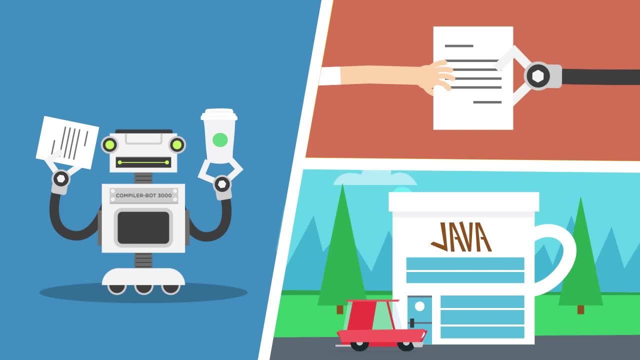 function is working well. You get your coffee each time you see it. Go to the coffee shop, to your assistant, But where's the variety? What if sometimes you want iced tea instead of coffee? Your current function only returns coffee. The function is limited. 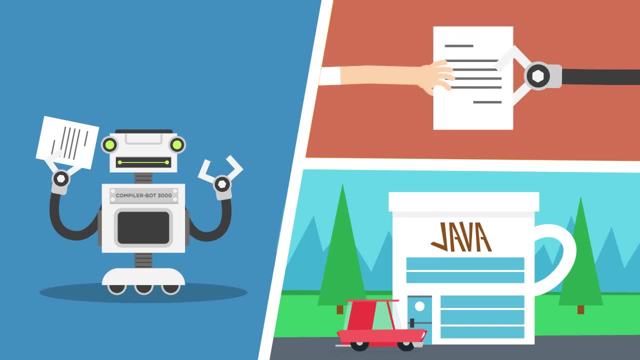 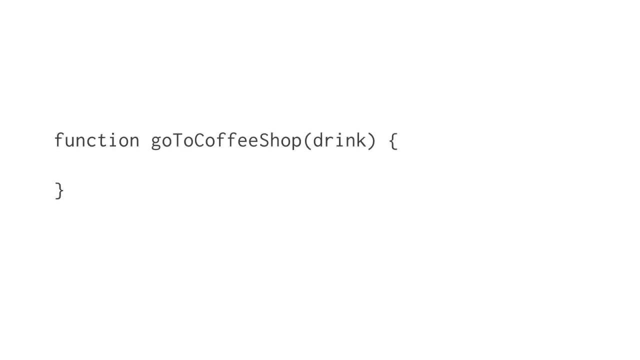 Instead, what if you can give your assistant information whenever you said go to the coffee shop, You can then ask them to get you something else. Now your go-to-the-coffee-shop function is really flexible. You can get an espresso, a hot chocolate or iced tea, for example. JavaScript functions can also accept information. 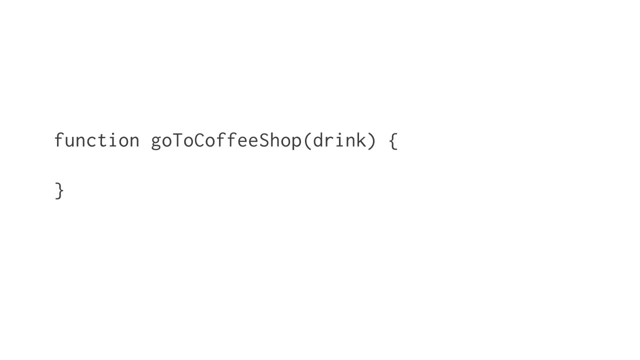 from a function to change how that function works. To have a function accept an argument, you add what's called a parameter inside the parentheses when creating a function. The parameter works just like a variable. You can name it anything you want, but you do need to follow the same rules when naming the parameter. 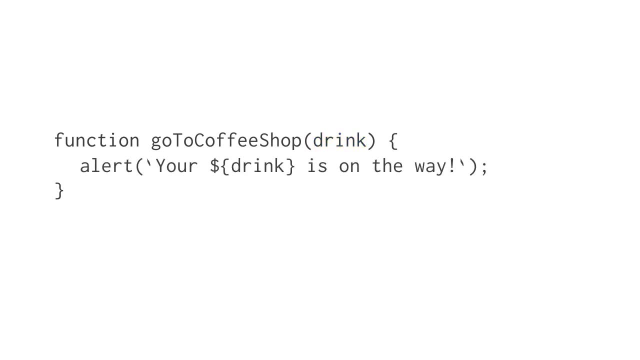 as you do when naming a variable Inside your function. you can use the parameter just like any variable. So now this function is expecting information. Each time you call the function, you need to pass it the information. Notice how much more flexible this function is. You can pass different values and get different. 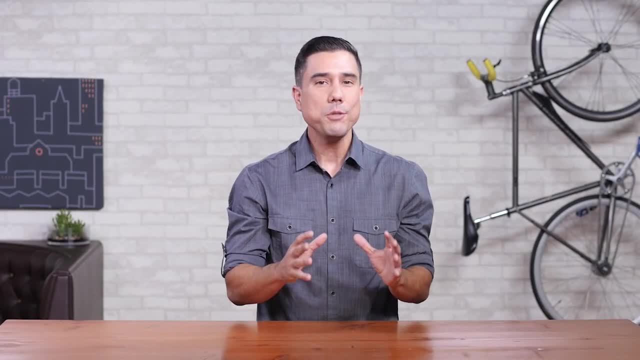 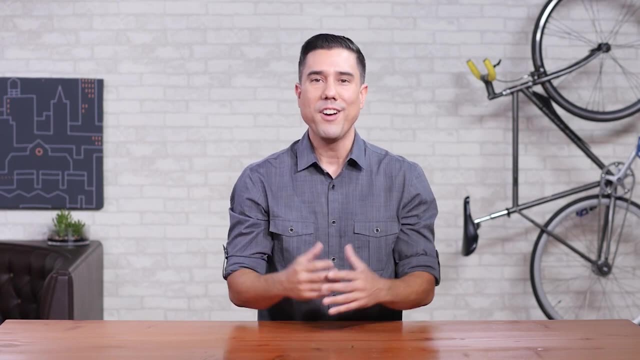 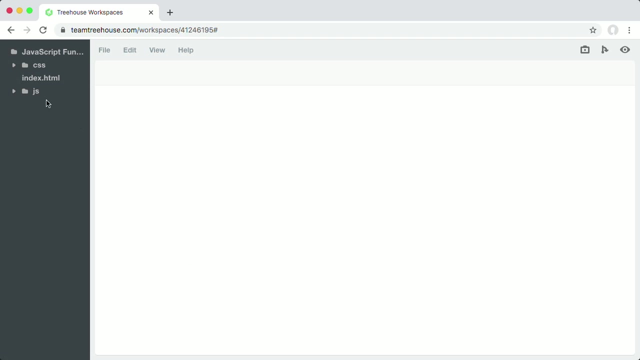 results. To summarize: a function parameter represents a value that you supply to the function via an argument so that the function can do something with that value. Let's look at how to use a function parameter as well as an argument in the getRandomNumber function we wrote in the previous stage. Open the file randomjs and make sure that you have. 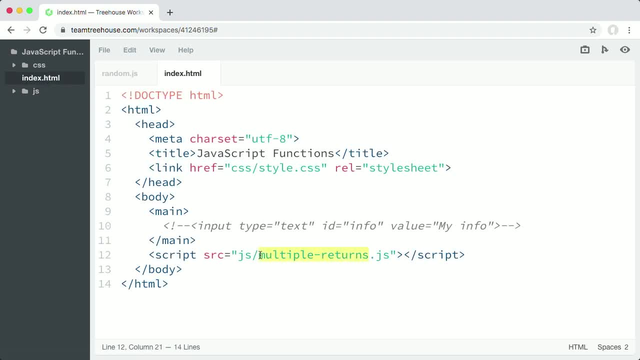 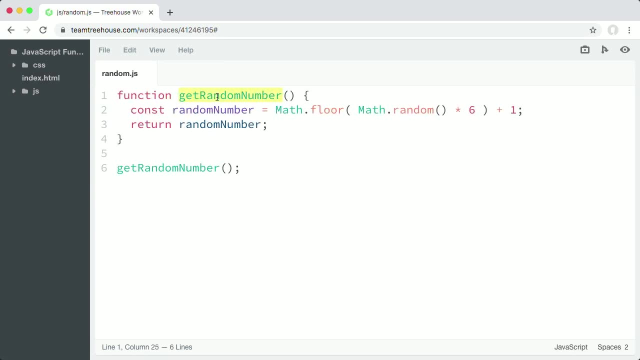 the script tag in indexhtml to point to randomjs. The getRandomNumber function only returns a value from 1 to 6, which works well for a die-rolling game, for example, but the function is limited. What if you want to create games? 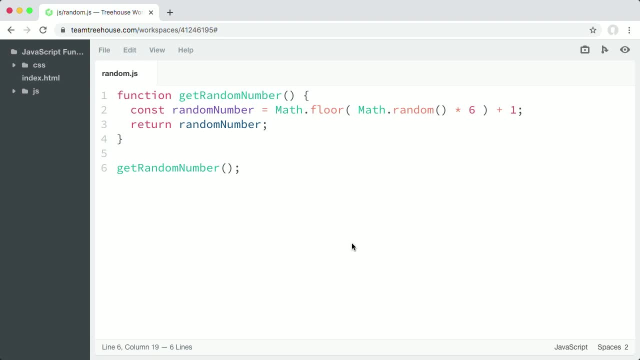 that use other types of dice, like 4-sided, 12-sided or 20-sided. Or what if you wanted to create a flexible random number generator that returned a number from 1 to 100,, 200, or 1,000? even You can make the random number function more flexible by accepting a value. 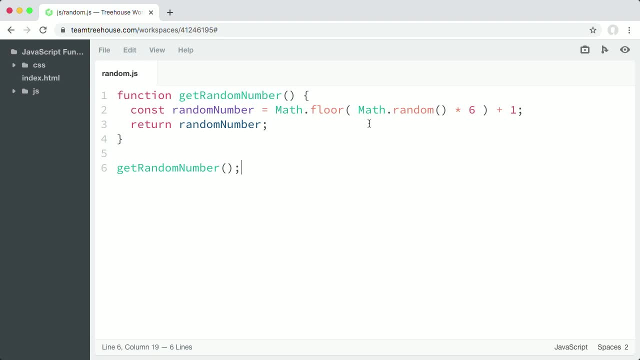 that sets the upper limit of each random number. First, let's add a parameter named upper inside the parentheses. Keep in mind that function parameters like the word upper have no particular meaning to JavaScript. Upper is just a parameter name that I came up with to represent the upper. 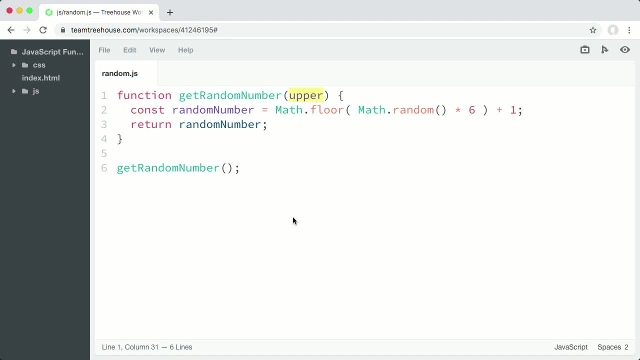 limit of the random number and it's going to hold a value that gets passed to the function when called. So currently the function returns a number from 1 to 6.. To use the value of the parameter, replace the number 6 with the parameter name upper. 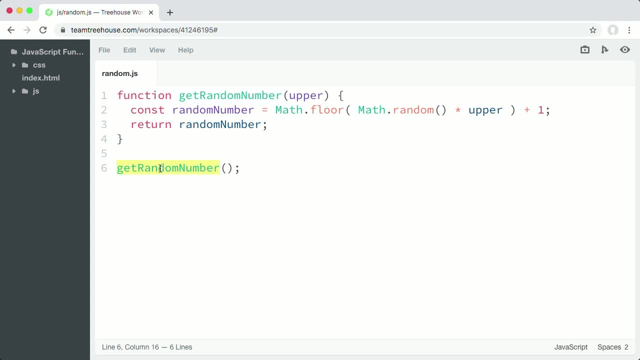 Now the getRandomNumber function is going to expect that you pass an information each time you call it. Again, when you pass information to a function, it's called passing an argument to the function. You can generate all kinds of random numbers now by calling this function. 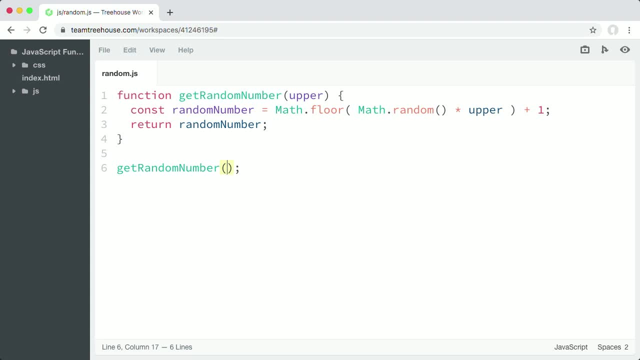 and passing it an argument. that's the upper limit of the function, So let's pass it 6.. I'll wrap this function call in a consolelog so that I can see the random number in the JavaScript console. Now take a look at this consolelog statement. You've actually been passing arguments for. 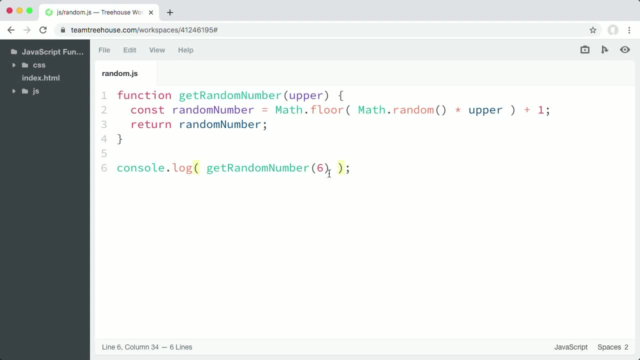 some time already. Notice how we're passing the value from the getRandomNumber function to consolelog. You've also passed values to other functions, like alert, for example. Those are all similar examples of passing an argument to a function to control the function. 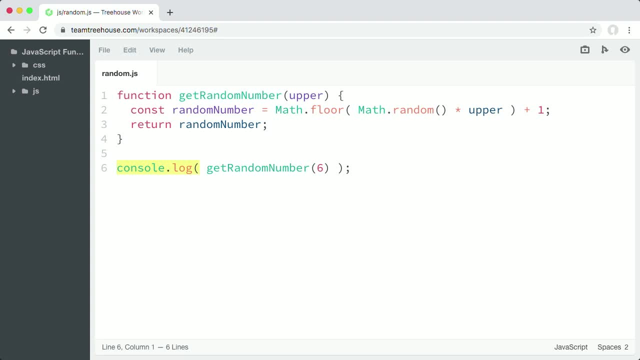 I'll wrap this function call in a consolelog so that I can see the random number in the JavaScript console. From here, let's assign the value of this function. to control how they work, Let's add a few more lines so we can see several different random numbers. 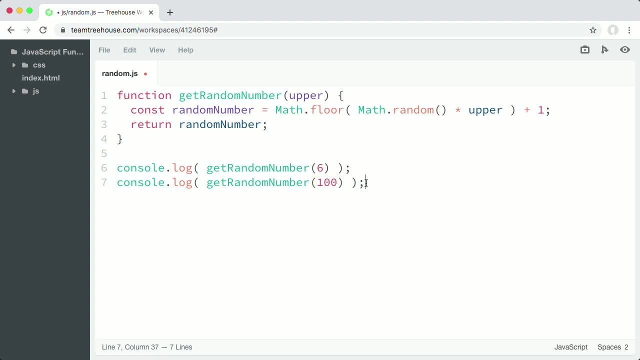 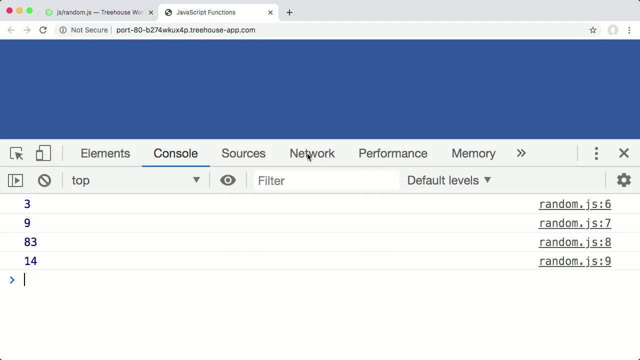 I'll pass this one, the number 100,, then 1000, and finally 20.. I'll save the file and preview the workspace in the browser. In the console we get 4 random numbers. Refresh the page and new random numbers display. 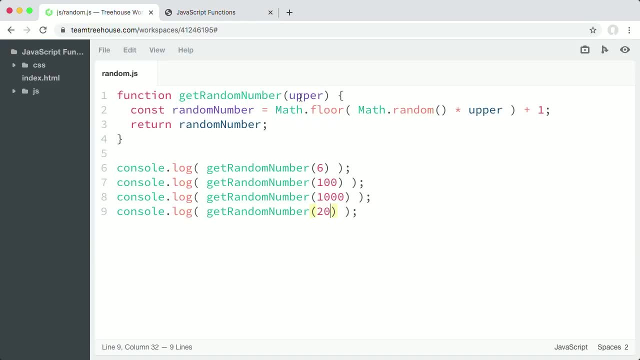 Great To recap. parameters are like variables that you define in the function, definition like upper, and arguments are the values you pass to the function when you call it, like the number six and 100.. Be sure to review the teacher's notes with this video. 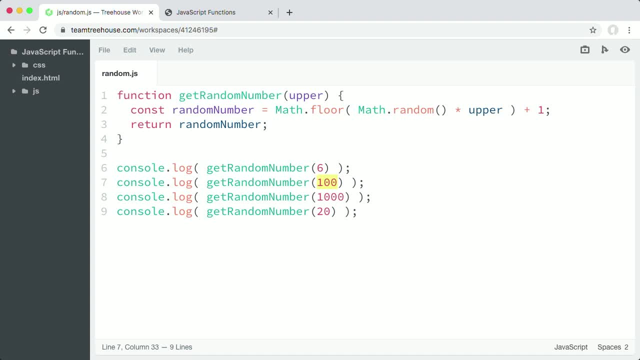 to learn more about the differences between parameters and arguments, You learn that you can pass information called an argument to a function. The function stores that value in a parameter and uses it within the function. Functions can accept more than one argument When calling a function. 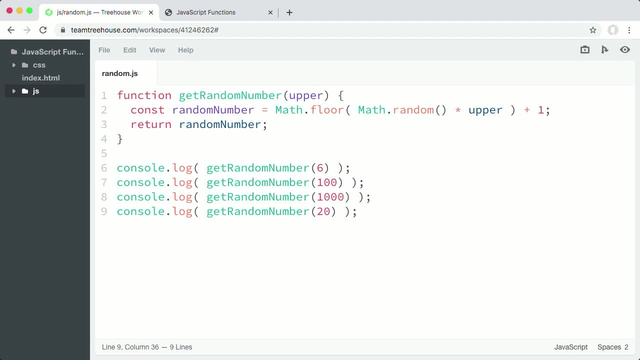 you're able to pass multiple arguments to the function. Each argument gets stored in a separate parameter and used as a separate variable within the function. Let's revisit the example of you and your assistant and the useful go to coffee shop function. Perhaps you want to not only order a drink. 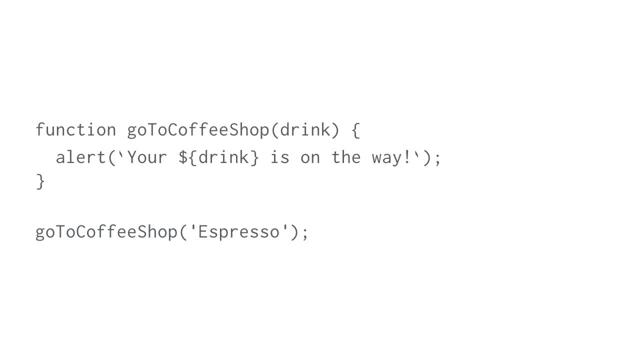 but also get something to eat when your assistant runs off to the coffee shop. Currently, the go to coffee shop function is limited to just one item. You can add another parameter in the function definition by typing a comma followed by the parameter name. Let's call it pastry. 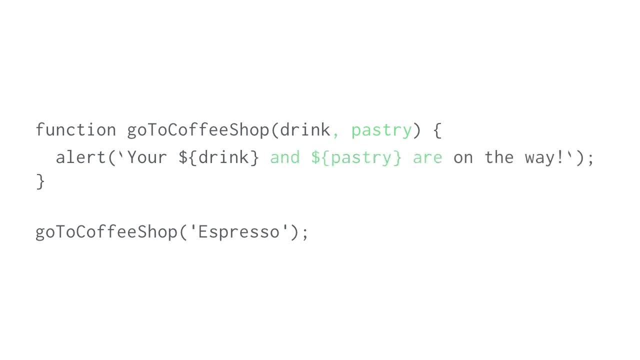 Then update the programming inside the function to use the new pastry parameter. Now this function expects two arguments. When you call the function, pass the second argument by typing a comma followed by a value- croissant, for instance. This function is now flexible enough. 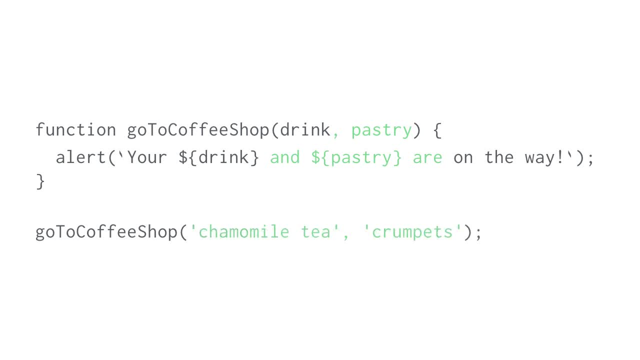 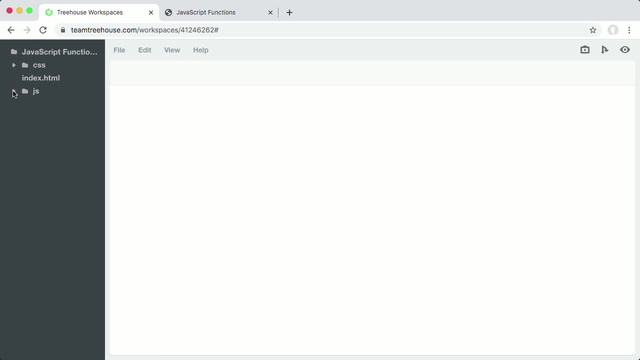 for you to order a different drink and pastry each time it's called. All right, Let's create a function that uses multiple parameters and arguments. This time open the file named multiple argsjs and, as usual, update the script tag and indexhtml. 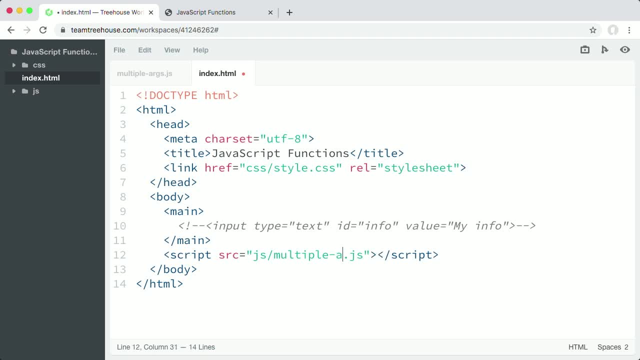 so that it points to multiple-argsjs. The function we'll create is going to calculate the area of a rectangle. Define a function named getArea, and the math for calculating the area is pretty straightforward. So let's create a function that says: 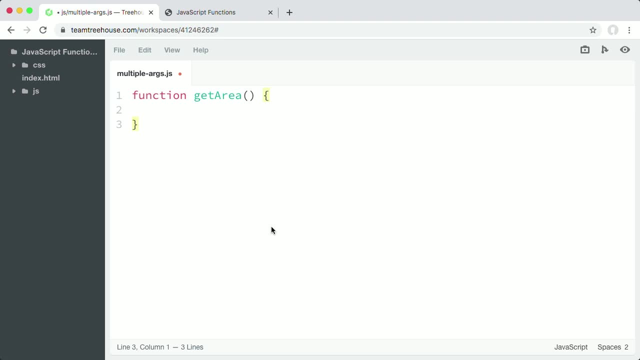 multiply the length of a rectangle by its width. Let's have this function accept a length value and a width value via the parameters width and length. Inside the function declare a variable named area. Its value is the result or product of width times length. 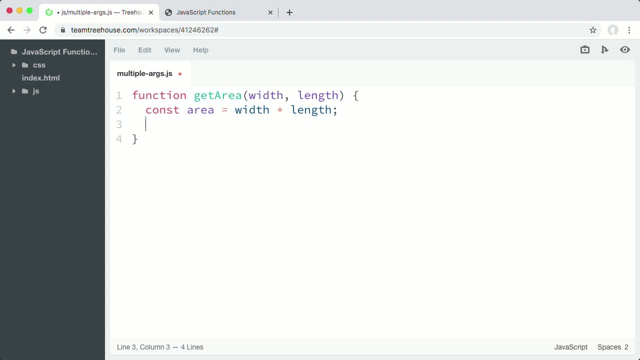 And let's have the function return the value of area using a return statement. Now to use this function, you call it and pass it a width and length value, Let's say 10 and 20.. Let's view the value in the console. 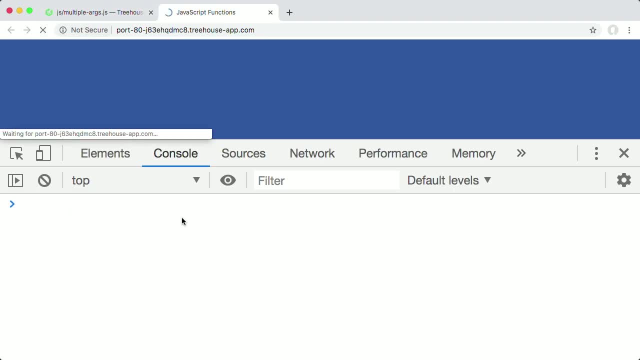 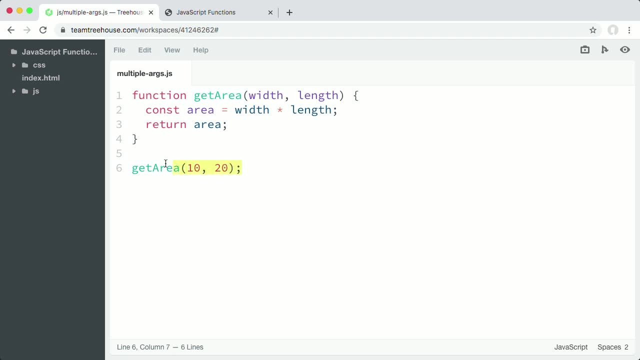 Once the browser loads JavaScript, you can call any functions in your JavaScript file directly from the console. For example, I'll test the getArea function by cutting the function call out of the file, saving the file and pasting it in the console. 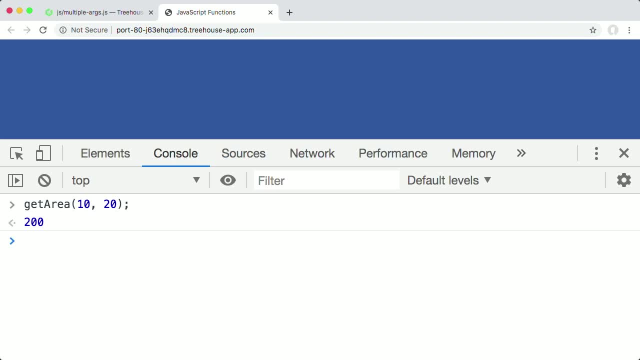 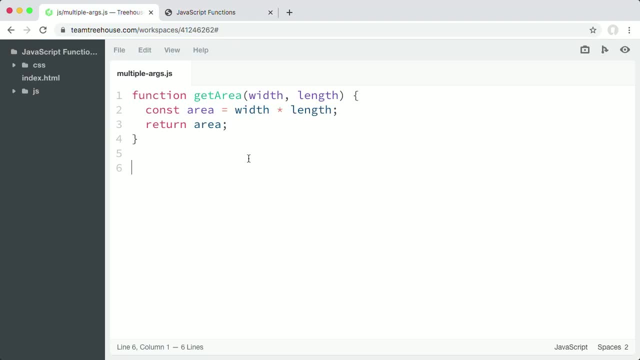 The function returns an area of 200.. But 200? what I want to return? a value that includes a unit of measurement like square feet and square meters, For example, a value like 200 square feet. To do that, I'll add a third parameter to the function, called unit. 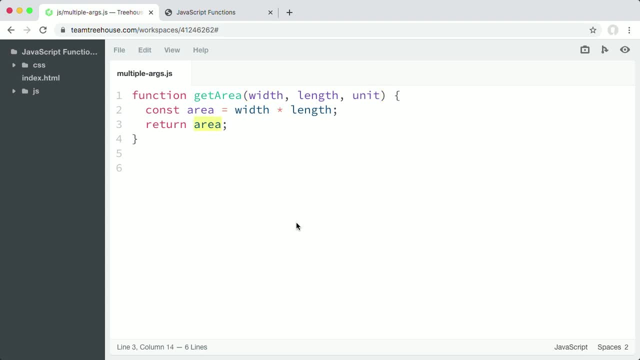 Remember a function can only return a single value, So I'll need to adjust the return statement to return a string holding the area and unit. I'll replace area with unit With a template literal that uses the dollar sign, curly braces syntax or string interpolation. 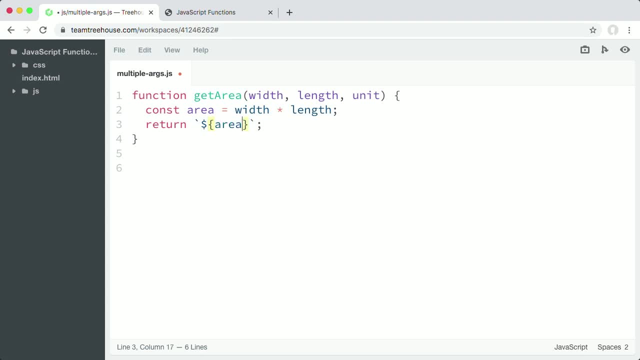 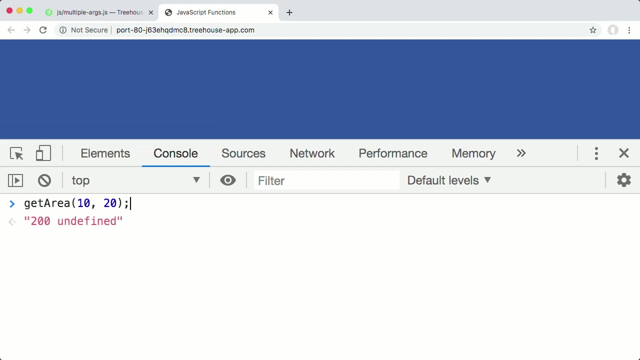 to insert the values of area and unit into the string. I'll save this file, refresh the page and back in the console. I'll press the up arrow key once to bring back the getArea function call. This time I'll pass the unit value as a string. 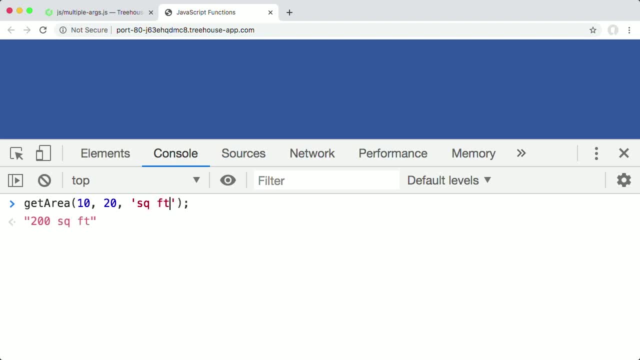 Now the console outputs 200 square feet. I'll try a different set of values, Let's say 5 and 17.5 square meters. That returns 87.5 square meters. Good, You're able to pass any number of arguments to a function. 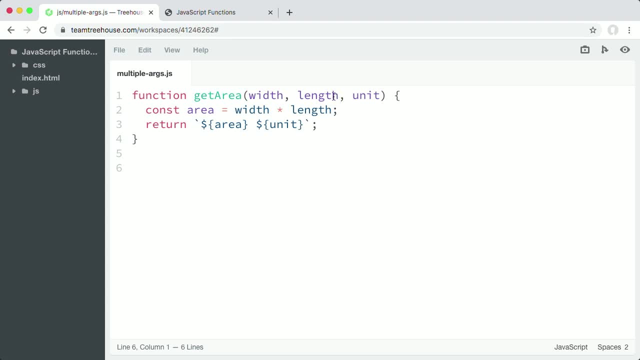 Too many arguments don't work. The functions, however, can make your functions difficult to manage. For instance, passing 12 arguments to a function and adding 12 parameters to a function definition makes it challenging to track each value. In a future course, you'll learn more efficient ways to pass lots of pieces of information. 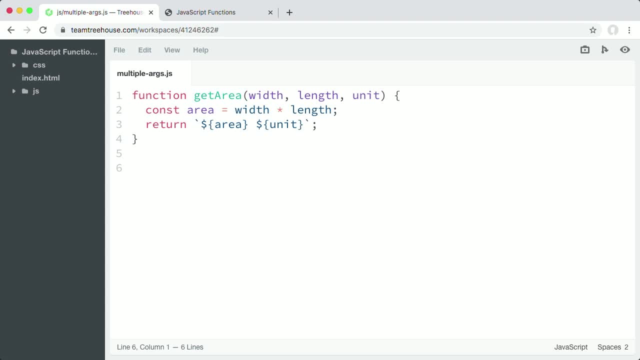 to a function with something called an array as well as an object literal that holds multiple values. For now, keep in mind that passing more than 4 or 5 arguments to a function can make your function tedious to use and harder to read. 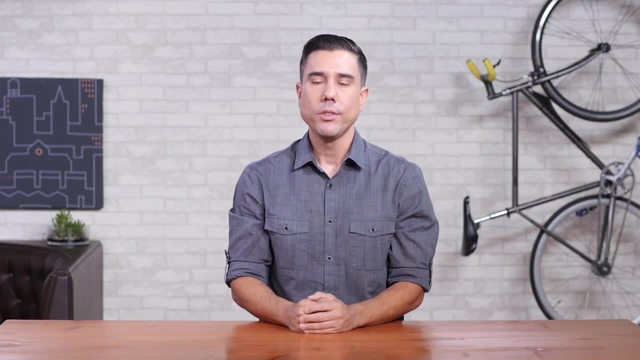 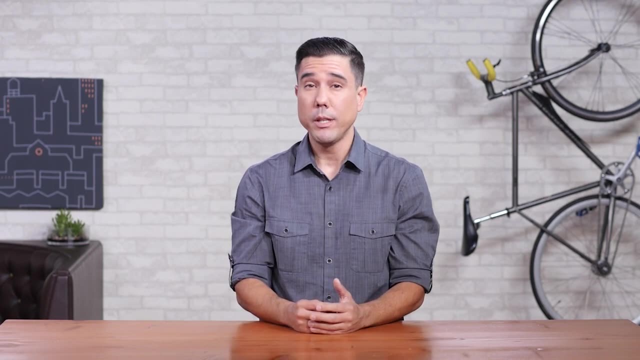 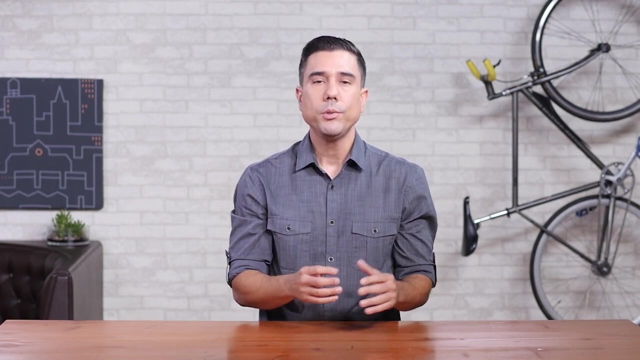 Let's try this, Let's see. With more and more complex programs, you'll likely end up writing multiple functions. You might also start using JavaScript libraries or utility functions that other developers wrote in your websites and apps. So it's possible, even likely, that within a function is a variable that uses the same. 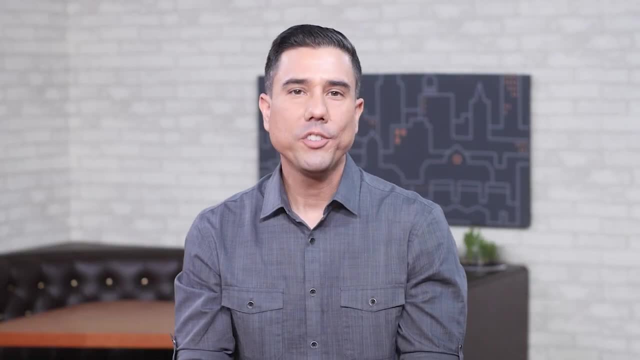 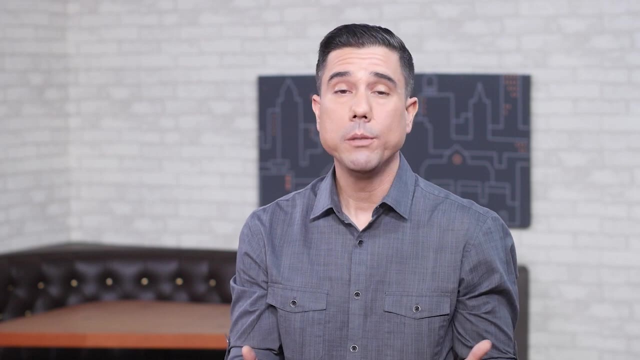 name as a variable used elsewhere in your script. For example, you might write a script with a variable named width, but also have a function called computeArea that has a width variable inside it- Two different variables with the same name. What does JavaScript do in this case? 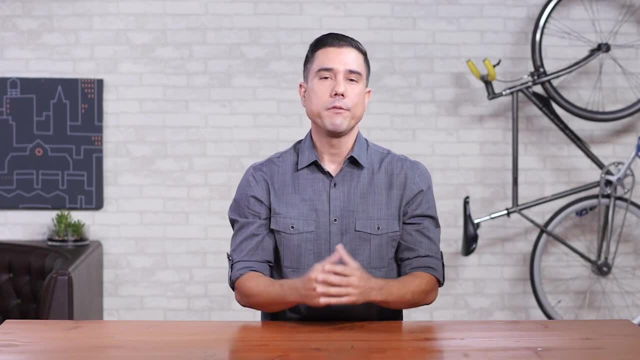 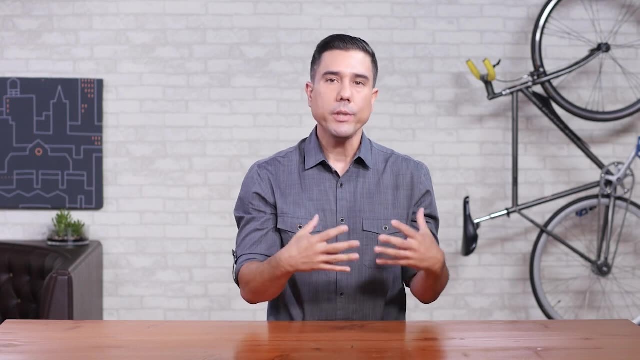 Fortunately, JavaScript provides separate scopes for each function. That is, each function acts like its own individual universe, if you will, And the variables that are created within that self-contained universe don't interact with the variables created in another universe or another function. 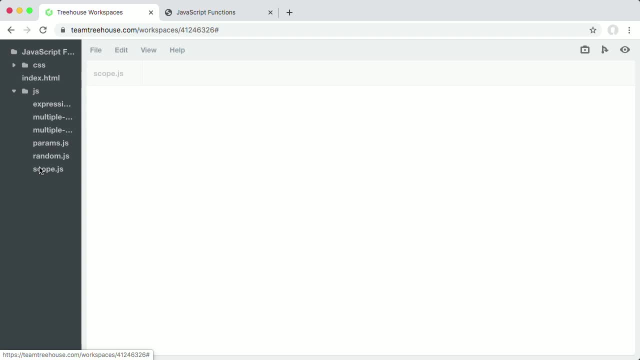 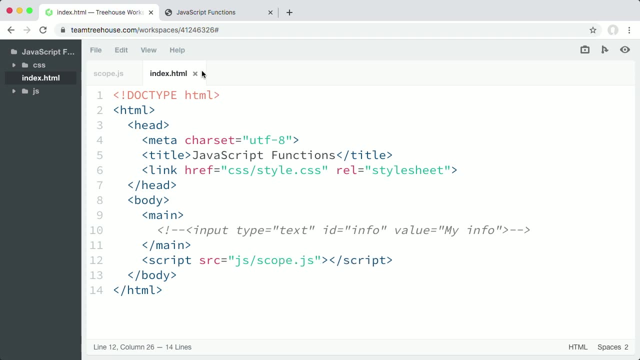 Let's look at an example. Open the file scopejs and update the script tag in indexhtml to point to it. Scopejs contains a small function named greeting. This function uses the value of the person variable to open an alert dialog displaying a greeting and a name. 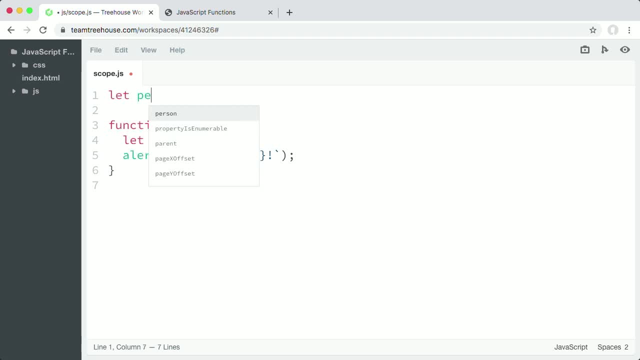 Now, outside of the function, I'll declare a variable, also called person, and store a different string in it. This time, leet, When you call the greeting function, the JavaScript engine jumps into the function, sets the person variable to meg, then opens the alert dialog displaying the message: hi meg. 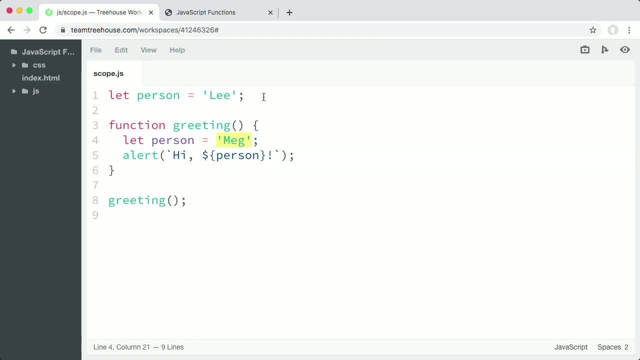 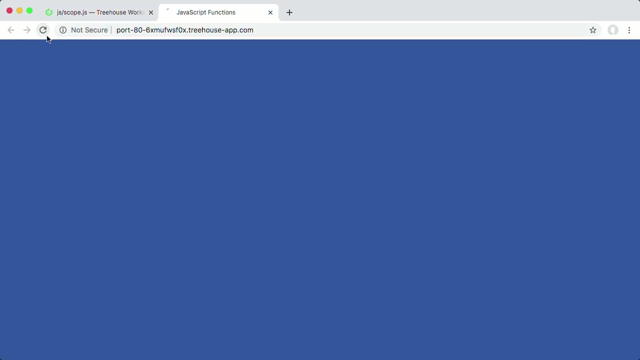 But what happened to the person variable declared earlier in the program, the person variable with the value of leet? If I add another alert method outside the function and pass it the same hi message with the person variable, notice how now we get one alert that displays hi meg and another. 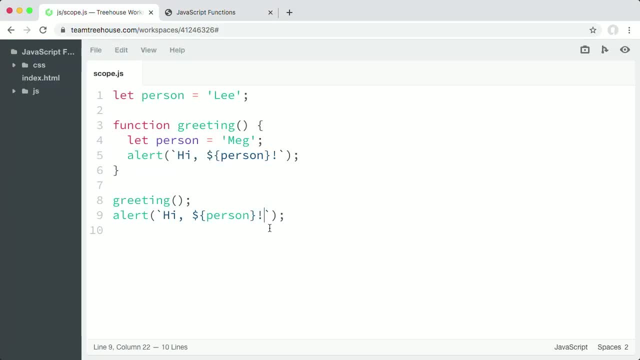 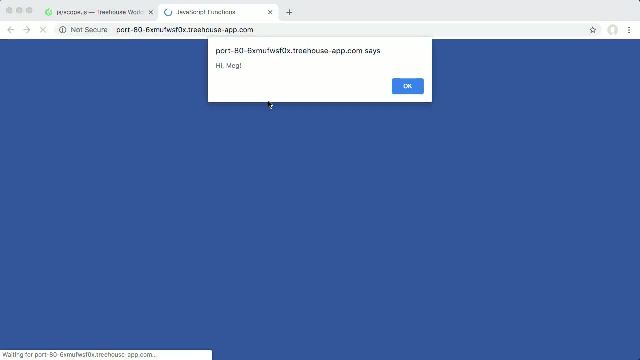 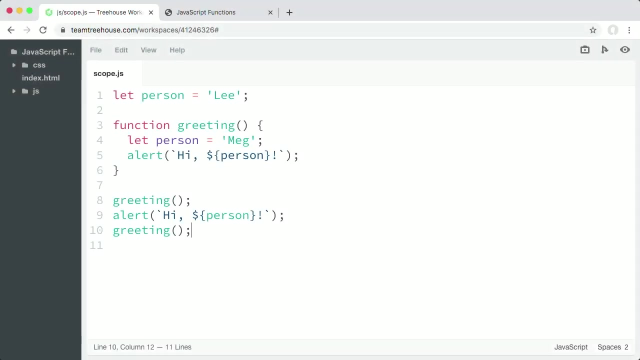 that displays hi leet. And if I call the greeting function one more time, just below this alert, we get the strings hi meg, hi leet and hi meg. In this script there are two variables: named person. Each has a different value. 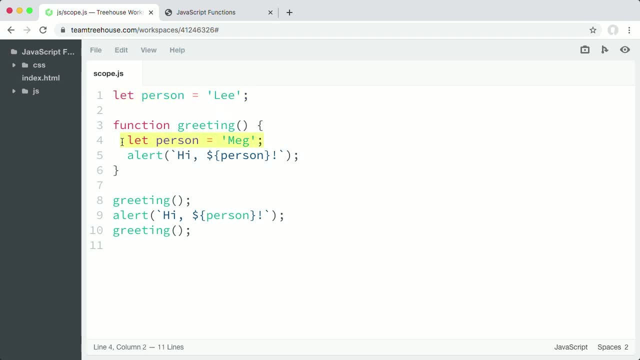 Each variable is declared within a different context or scope. In programming, scope is the context in which values are visible or can be referenced. Earlier I mentioned that each variable has a different value. Each variable is declared within a different context or scope. 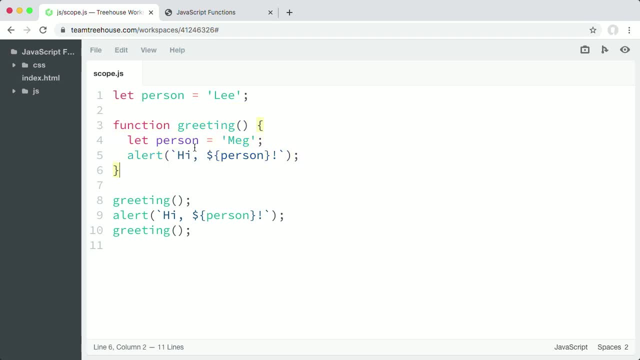 In programming, scope is the context in which values are visible or can be referenced. The function acts like its own individual universe and any variables created within that self-contained universe cannot interact with variables created outside of that so-called universe. When you declare a variable inside a function, for example, you can only use the variable. 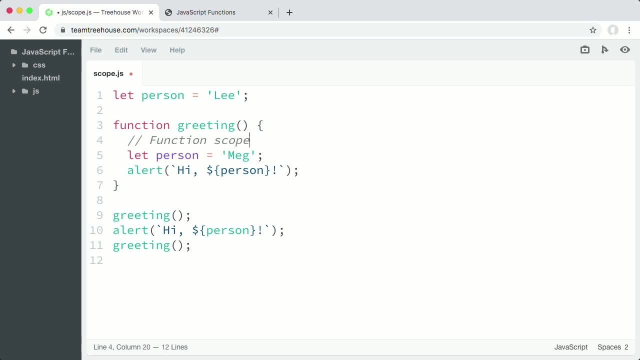 within that function. In this case there's the scope of the greeting function. The person variable declared inside the function lives inside this function only. You can't access or change the variable outside the function. This also means that functions do not have access to each other's scopes. 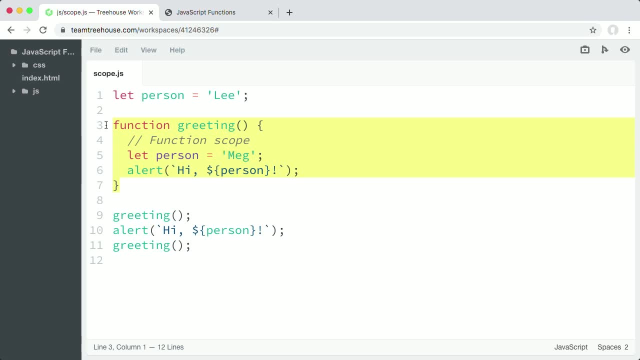 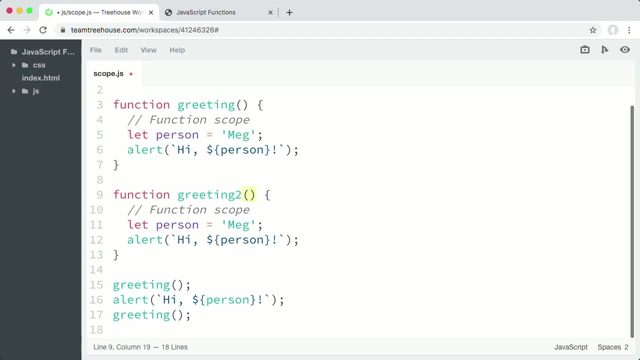 To better demonstrate, I'll create a second function by copying the greeting function, pasting a new function below it and changing the name to greeting2.. This time I'll set the value of the person variable to Robert and the alert message to good morning. 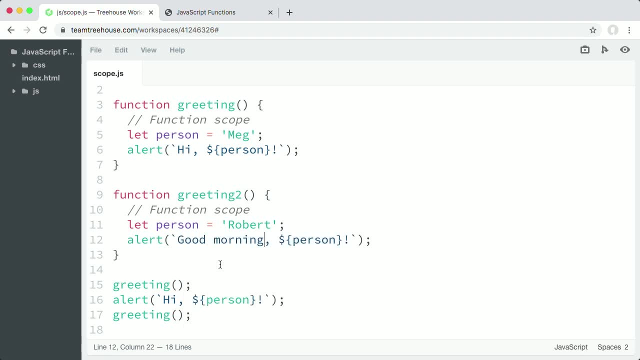 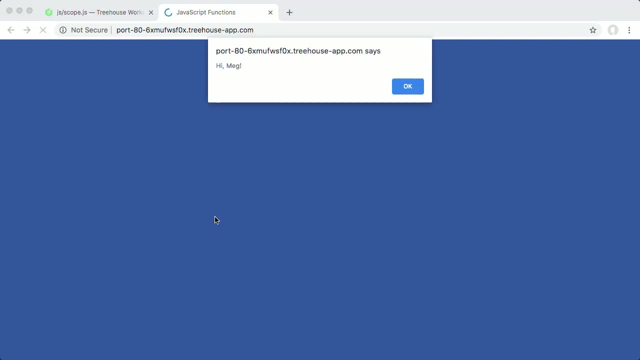 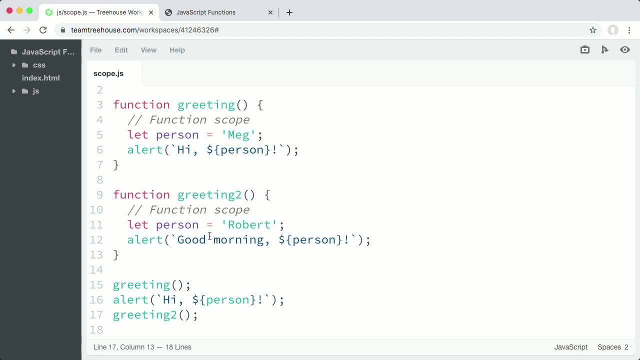 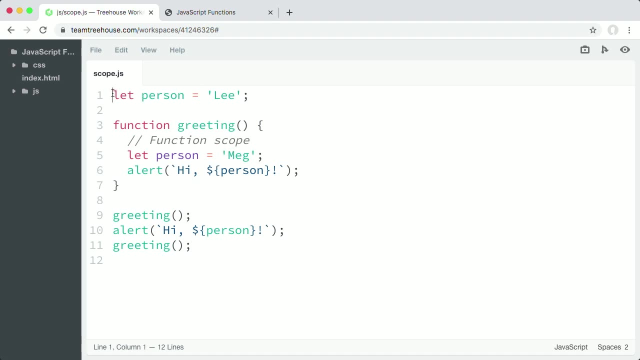 Function scope is one of the ways JavaScript protects variables from overriding each other. There's also a scope outside of a function. It's called the Global scope and it's the scope where the other person variable lives. variables you create that are not contained inside a function are accessible in this larger universe. 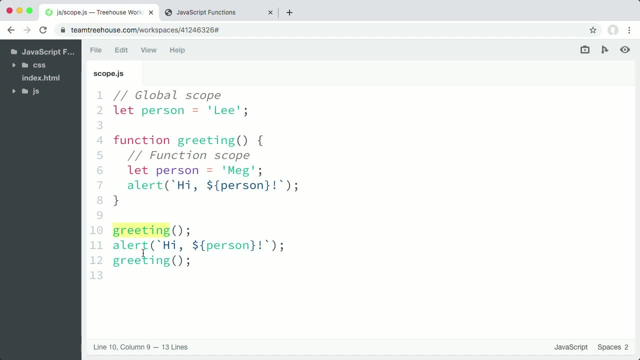 called the global scope In our script. wherever we call the greeting function, we're accessing the person variable that lives inside the function. So the alert displays hi meg. However, the alert method outside the function references the person variable in the global scope, which is: 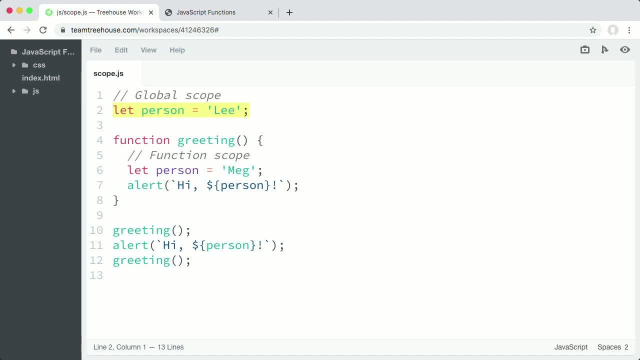 set to lead. The reason I mentioned that the global scope is a larger universe is because functions can access the global scope. In other words, you can change the value of a variable that's defined in the global scope from inside a function. This is usually not recommended. 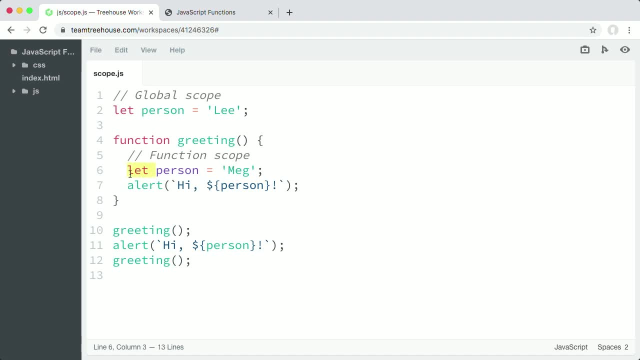 but I'll show you an example. If I remove the let keyword inside the greeting function, the program changes dramatically. Without a let or even a const keyword, the function now reaches out into the global scope to access a variable named person. Once it accesses the variable, 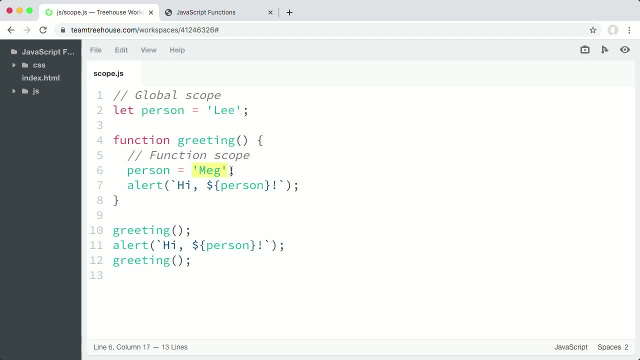 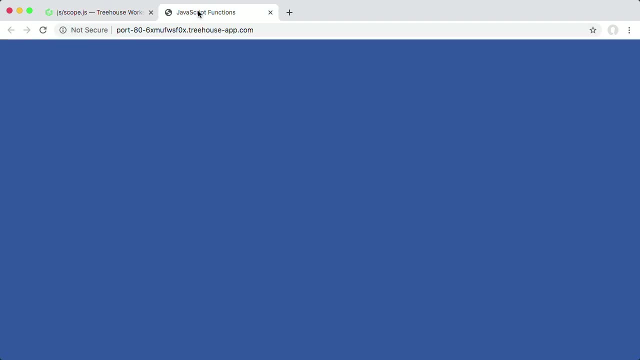 it changes or re-accesses the variable. So if I remove the let keyword inside the greeting function, it re-assigns its value to meg. Now the person variable in the global scope contains the string meg. The lead value is gone forever. Notice in the browser how all three alerts display: hi meg. 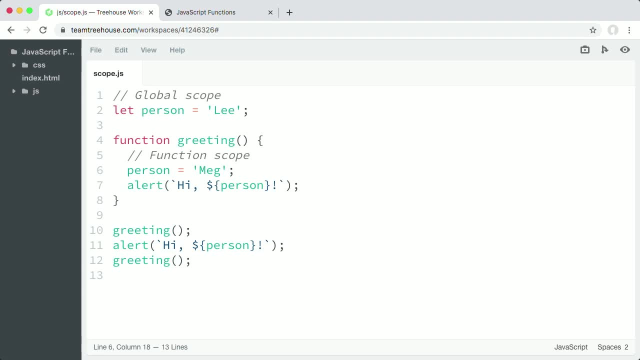 As you learned in an earlier course, the const keyword protects a variable from being changed to a different value. So one safeguard to prevent this from happening is to declare global variables that shouldn't change with the const keyword. Now the script does not change the value of the variable, So the const keyword is not changed. 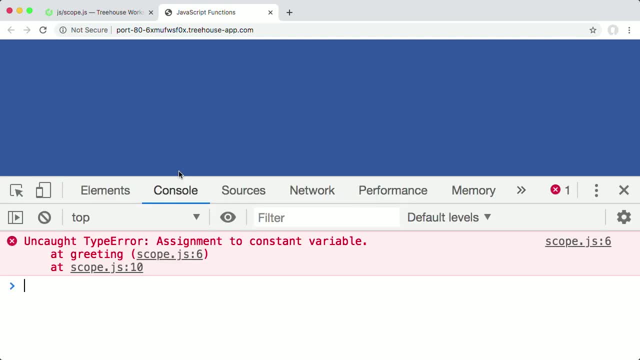 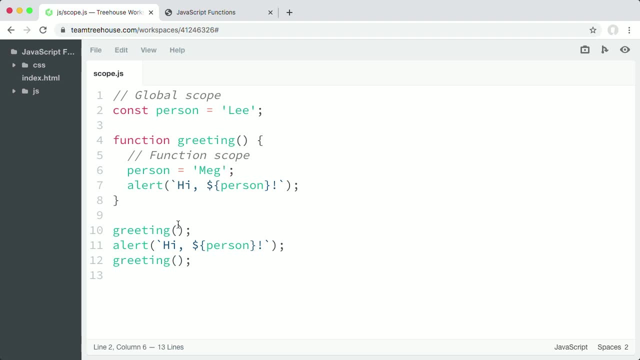 And the console outputs a type error. instead It says assignment to constant variable on line six. It's generally not recommended to access global variables from inside your functions. It makes keeping track of variables and debugging difficult. Also, one of the main benefits of functions is that 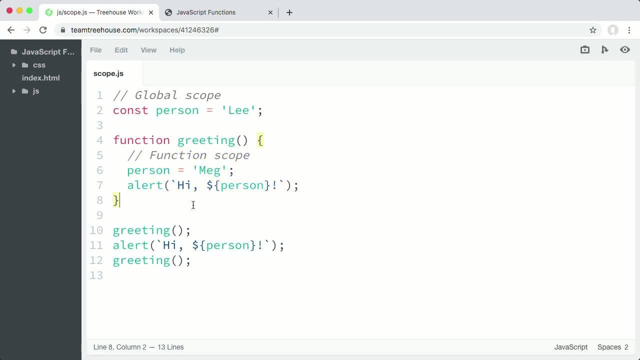 they are self-contained blocks of reusable functionality. So making a function dependent on global variables that live in other parts of a script can make the function harder to reuse and more likely to break. So if I remove the let keyword inside the greeting function, the function now. 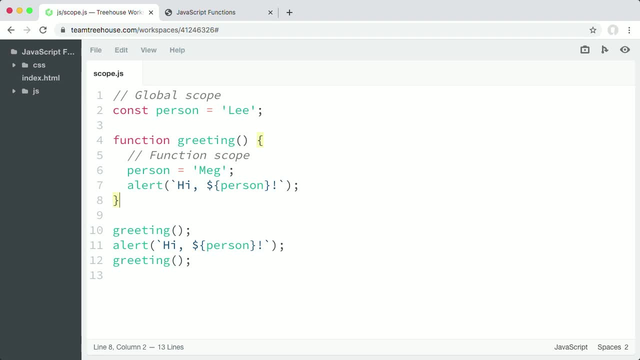 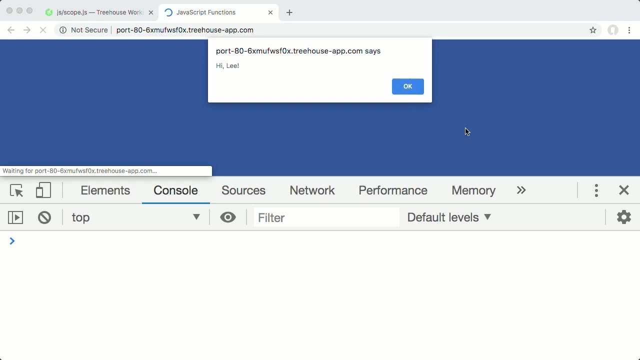 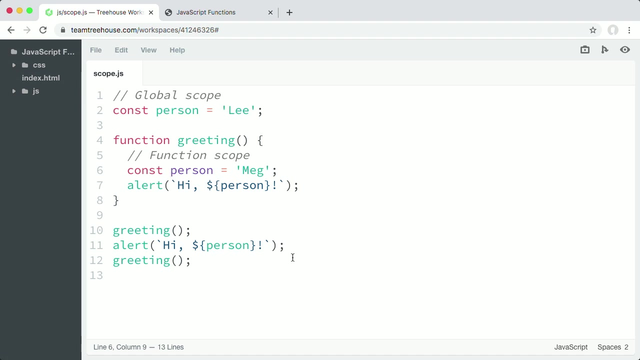 has to produce unexpected behavior. So it's acceptable to use the same variable name inside of different functions. as long as you use the let or const keyword to declare the variable, The variable will only exist inside that function. You might be wondering: why not just use different? 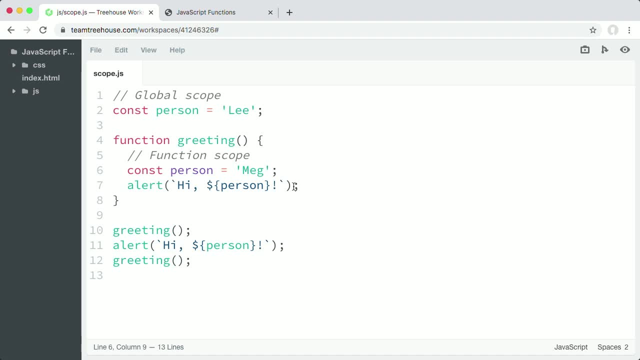 variable names everywhere and avoid any issues in the first place. Well, you always want to make sure your variables are in the right place, So you can use the let or const keyword to declare the variable. variable names are meaningful and accurate for the context in which they live. Because of the way 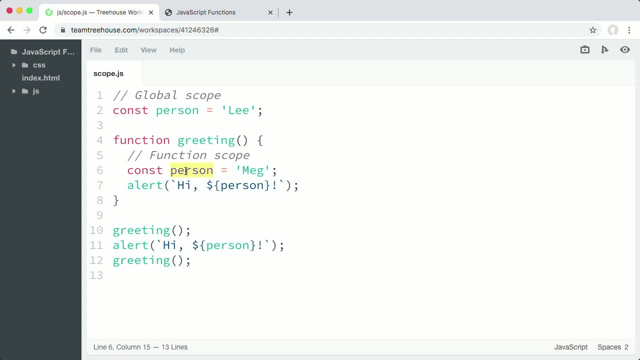 scope works, you don't need to worry about using the same names as long as they live in separate functions or scopes, And sometimes you might not have a choice for variable names, For example, if you're using a JavaScript library or helpful utility functions that other developers wrote. 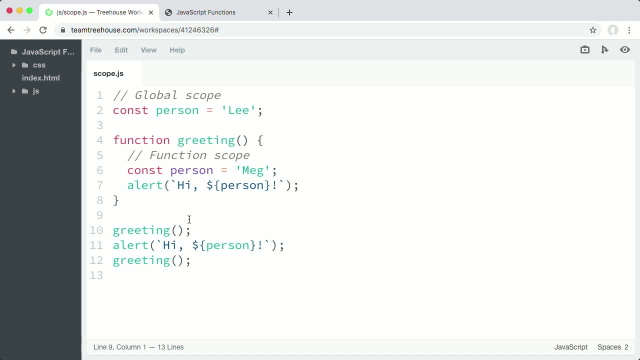 you might run into variables with the same name and you don't want to change those because the library expects those exact variable names. However, because those variables live within different scopes, they won't collide with any variables you might create. So far, you've written. 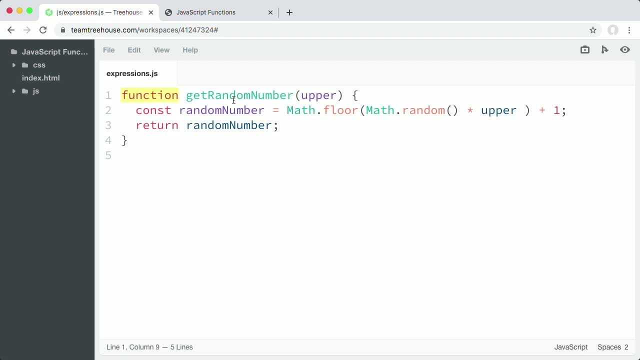 functions that look like this: The function keyword followed by the name of the function. This is what's called a function declaration. There's another syntax for creating a function, that's called a function expression. Open the file expressionsjs and in indexhtml. 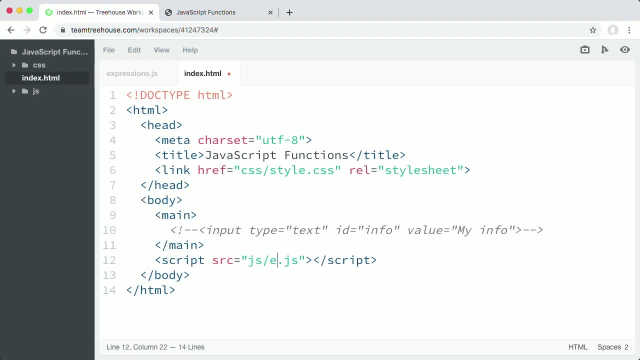 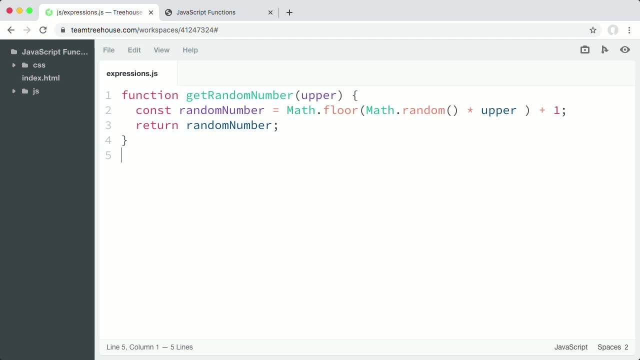 update the source attribute in the script tag to js forward slash expressionsjs. A function expression lets you assign a function to a variable. For example, you could rewrite the get random number function to look like this: Notice that there's no name after the function keyword: A function without a name after the? 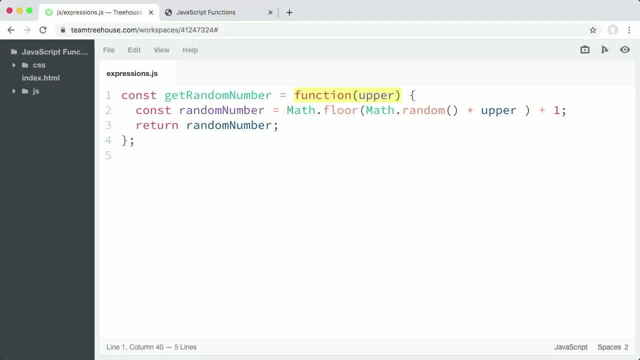 function keyword is called an anonymous function. Instead, the name comes from the variable. In other words, I'm storing a function as a value in a variable name. get random number. Also, in this case, you're creating a statement by assigning a value to a. 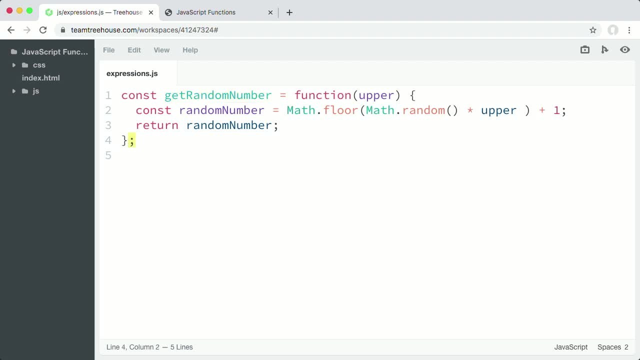 variable. Because of this, you add a semicolon after the closing curly brace. You call this type of function the same as you would a function with a name or a function declaration. Use the name of the variable, followed by parentheses. So now, anytime you come across a function that's assigned, 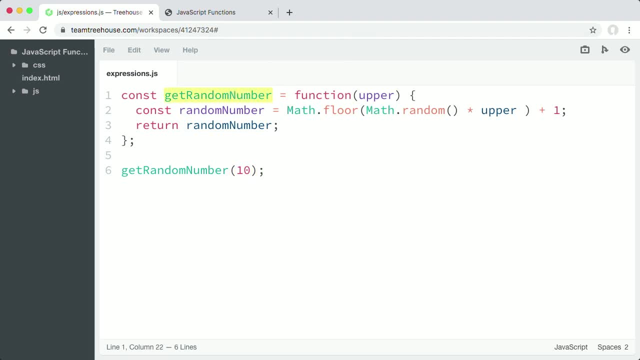 to a variable, you'll know that it's a function expression. You're also going to explore function expressions further in the next stage on arrow functions. Finally, function declarations and function expressions work in much the same way, except for one subtle but important difference: You can call a function declaration before it's. 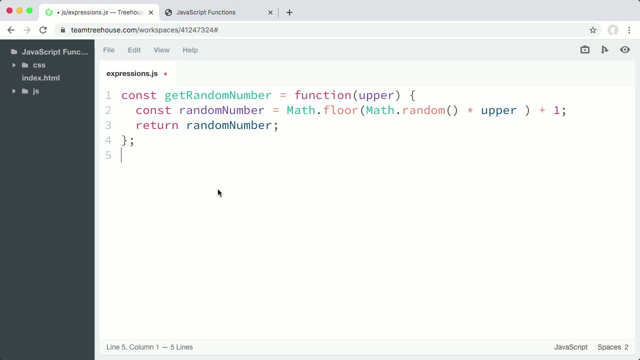 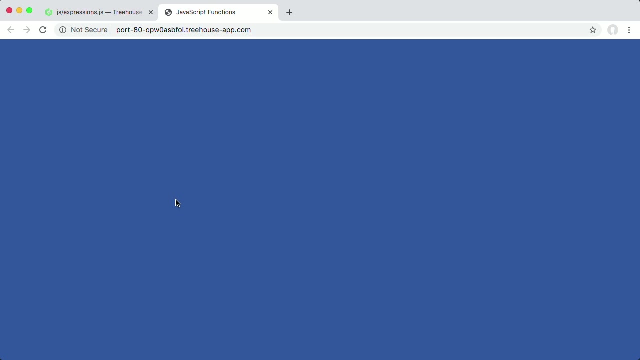 defined. For example, I'll convert this function back to a function declaration. Then call: get random number above the function and print its return value to the console with consolelog. Notice how the function still works as expected. We get a random number. That's because function. 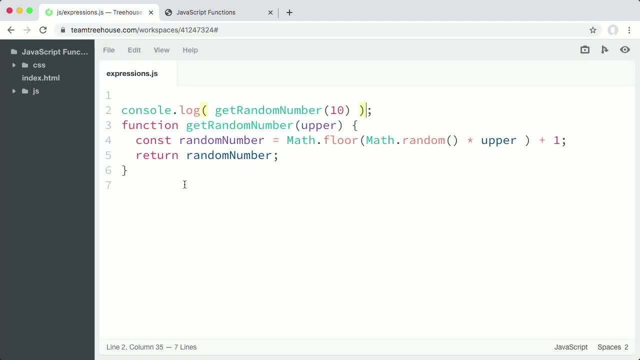 declarations load before any code is executed. When the JavaScript file loads, the JavaScript engine behind the scenes moves all function declarations to the top of their current scope, in this case the global scope. Since the JavaScript engine immediately knows about any function declarations, you're able to call a function before it's declared in the file. 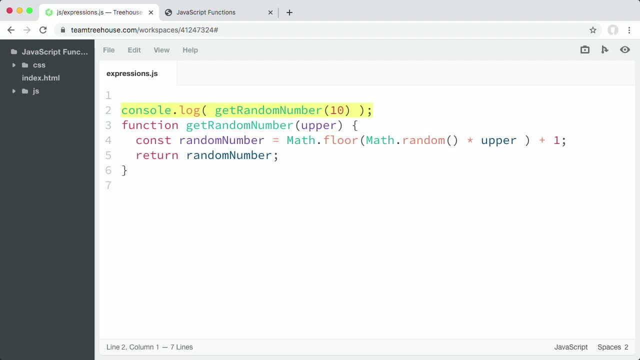 This behavior is called hoisting. Function expressions, on the other hand, are not hoisted or lifted up to the top of their scope. A function expression loads only when the JavaScript engine reaches the line of code it's on. For instance, I'll again convert the get random number function into a function expression. 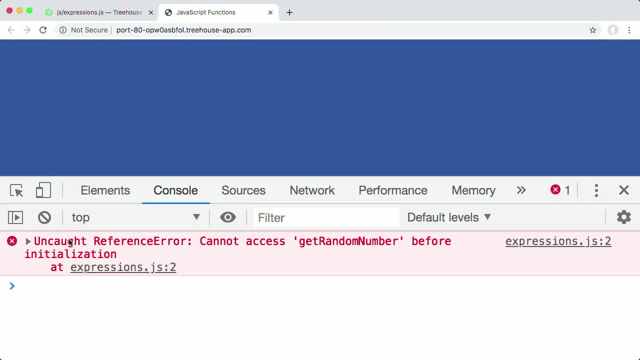 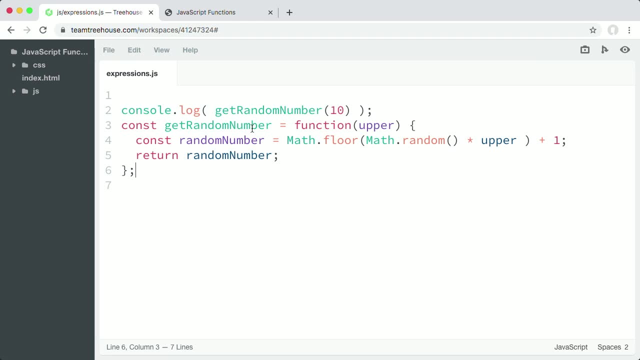 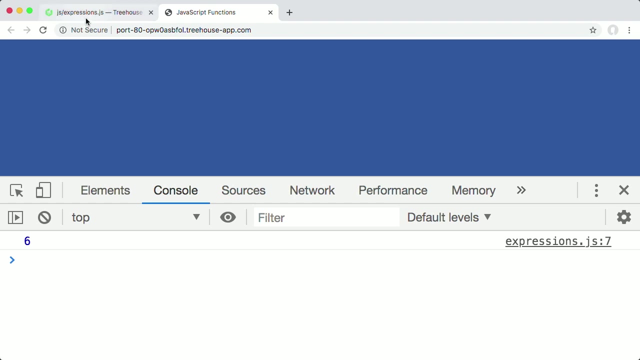 Now the console outputs an error. It says: uncot reference error. Cannot access get random number before initialization. So remember, if you call a function expression before it's defined, you'll get an error. The approach you use to writing functions is a matter of personal preference. Choose one. 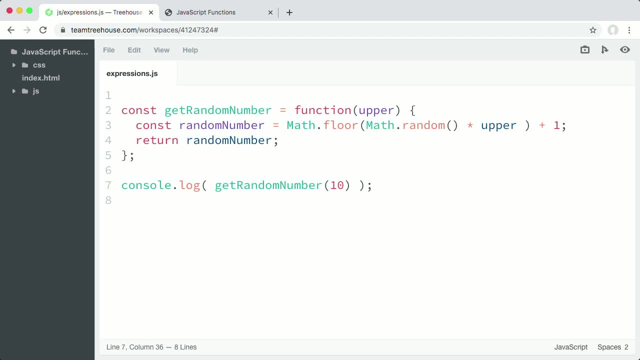 style and try to stick with it throughout your script. If your program at some point might need to call a function before it's declared, then use function declarations Now. some developers also prefer the structure that function expressions provide to their code. 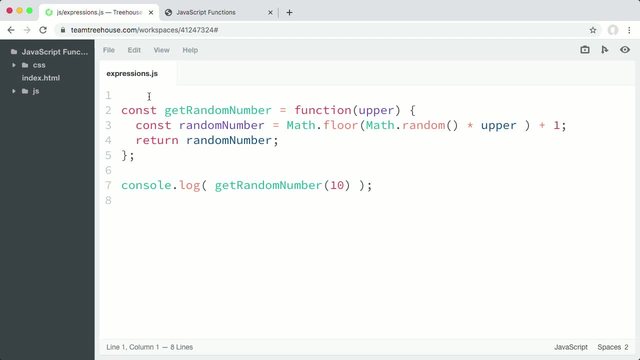 Since you're not able to call a function expression before it's declared, it requires that you write your functions up top in a specific order, otherwise they won't work. Then any code that calls and runs functions get placed toward the bottom of the program or file. 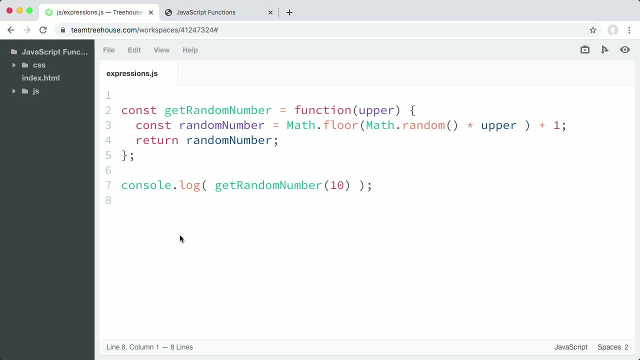 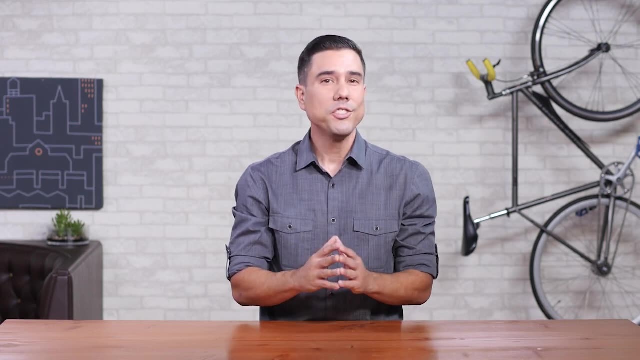 which can make your code more readable and predictable. But again, the style is mostly up to you and your team. Understanding the basics of functions is a big deal. Just about every program you'll write will use one or several functions As you become more experienced with JavaScript. 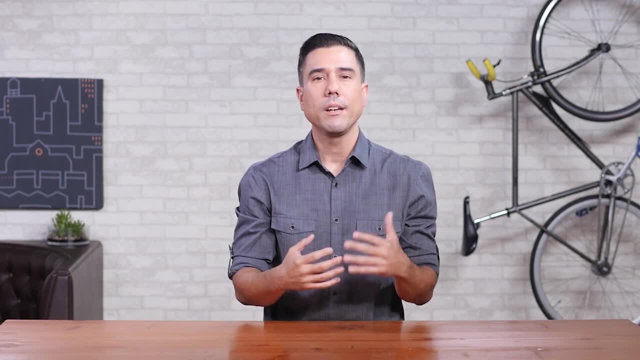 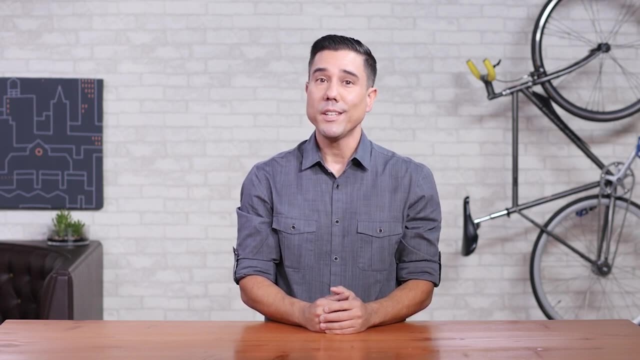 you'll start to notice that parts of your code are repetitive and do the same thing over and over. So if you find yourself writing the same exact code more than once, it's a symptom that something is likely wrong. That's where a function can help you avoid duplicating code. 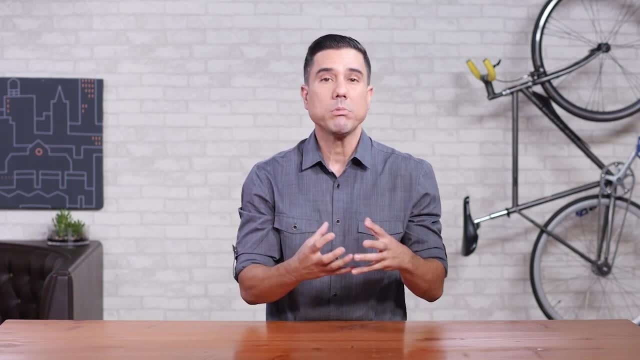 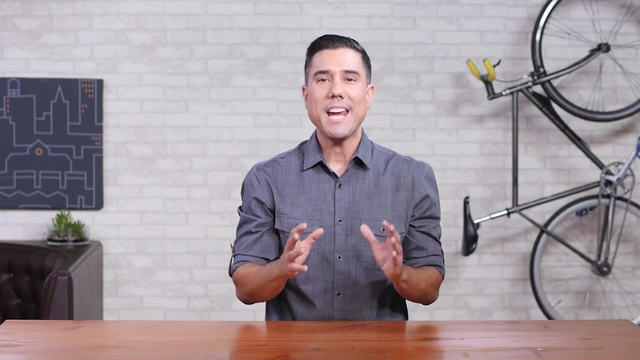 and provide a way to group reusable code together to use or call later at any point in the program. In the next stage you'll build on your knowledge of functions by learning about arrow functions, which offer a more concise syntax for writing functions. See you soon. 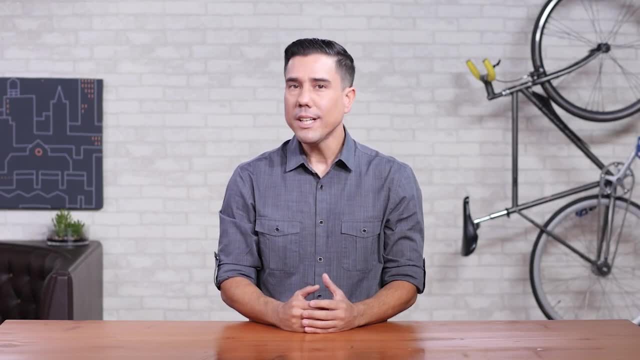 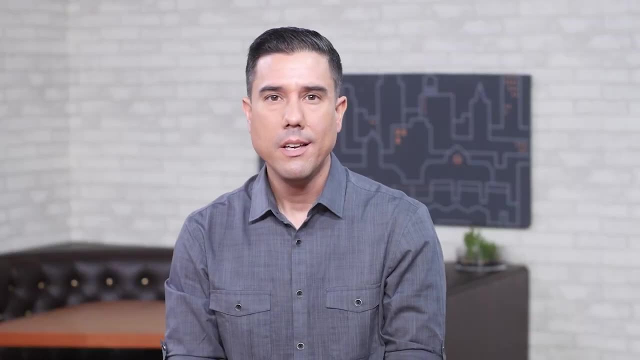 As you learn more about JavaScript and how the language evolves, you'll realize that it provides different and perhaps more efficient ways to do similar things. Working with functions is one of those things. So far, you've learned how to write a function as a declaration and as an expression. 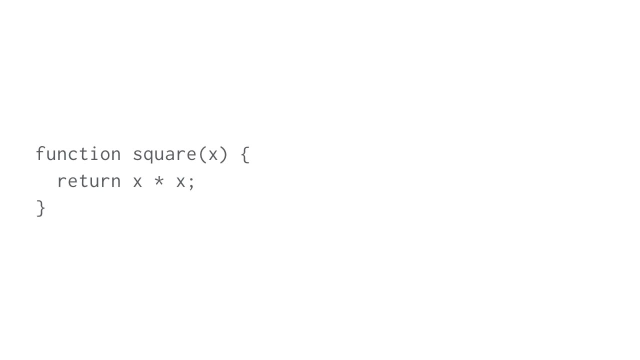 A function declaration, for example, defines a function using the function keyword followed by the name of the function, And a function expression is an anonymous function or a function without a name that's assigned to a variable. In this stage, I'll teach you another method. 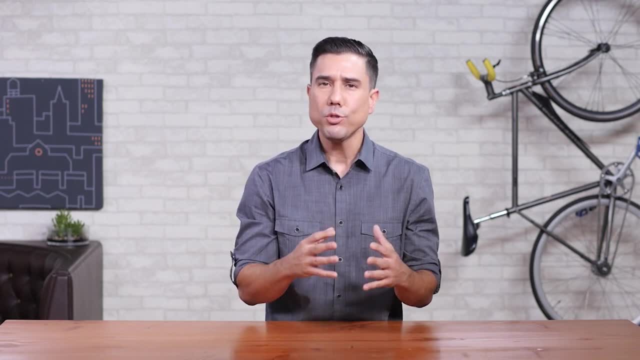 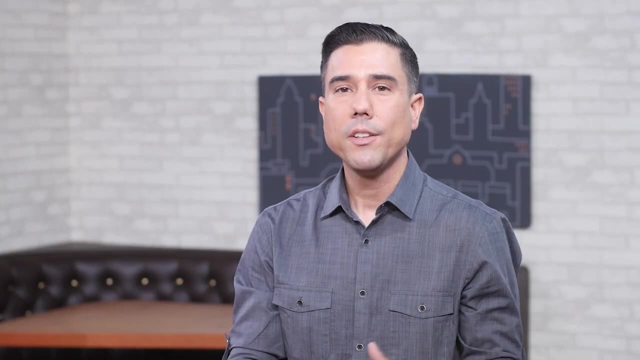 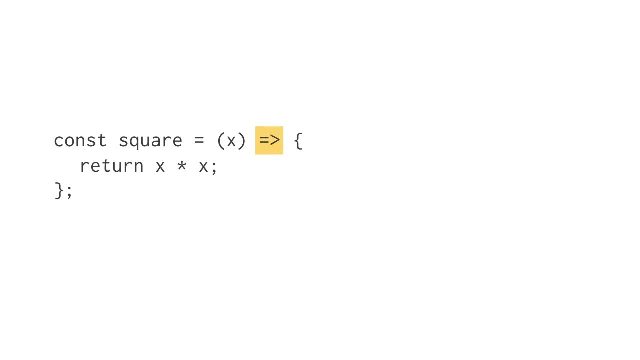 You omit the function keyword and after the parentheses you'll see an arrow function. You omit the function keyword and after the parentheses you'll see an arrow token, which is just an equal sign, immediately followed by the greater-than sign. The body of the function can remain the same. 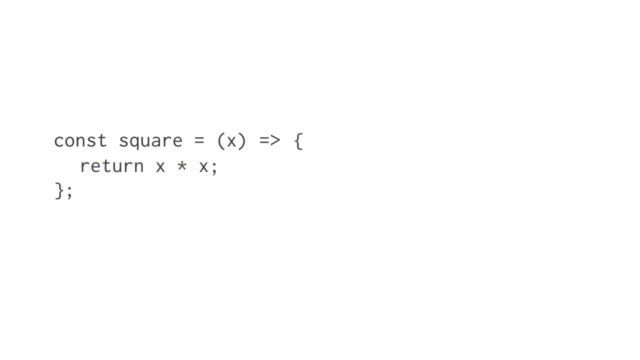 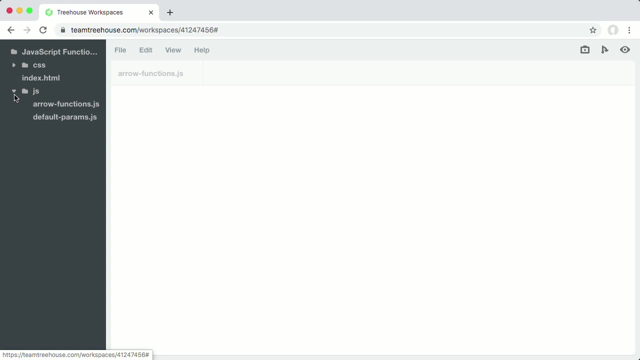 but, as you'll soon learn, there are ways to make arrow functions even more compact. You can access the new set of files by launching the workspace with this video Open to the file arrowfunctionsjs located inside the jazz folder. The files are already linked to indexhtml. 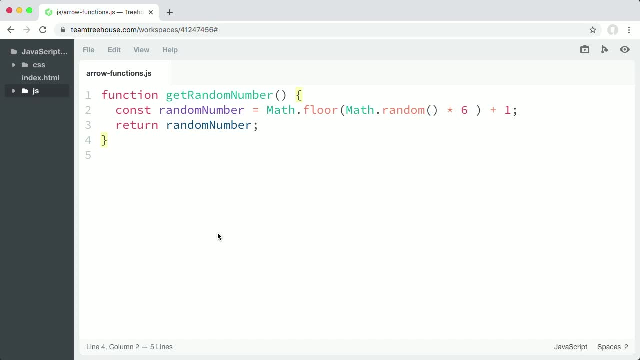 The get random number function in this file is written as a function declaration. That is a function that begins with arrow. That is a function that begins with arrow, with the function keyword followed by the name of the function and a pair of parentheses. 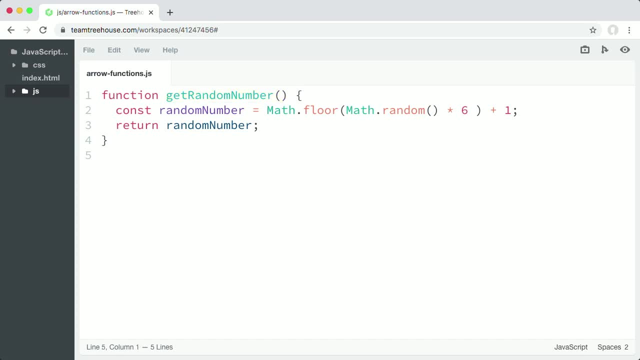 We're going to convert this function to an arrow function Now. arrow functions are similar to the function expressions you learned about earlier, so let's first change the getRandomNumber function declaration to a function expression and then to an arrow function, Create a variable named getRandomNumber and assign an anonymous function to it. 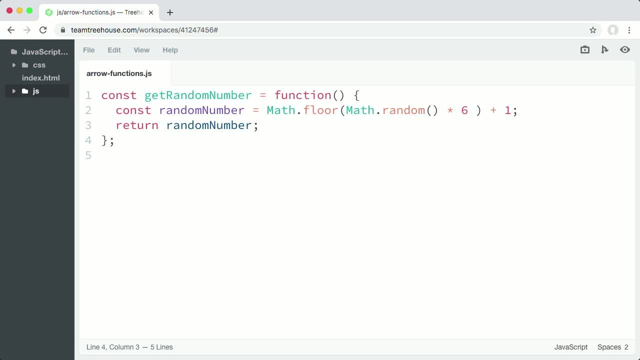 You can make this function even more concise using the arrow function syntax. To convert the getRandomNumber function expression to an arrow function, remove the function keyword and after the parentheses, add an arrow which is an equal sign, immediately followed by a greater than sign. 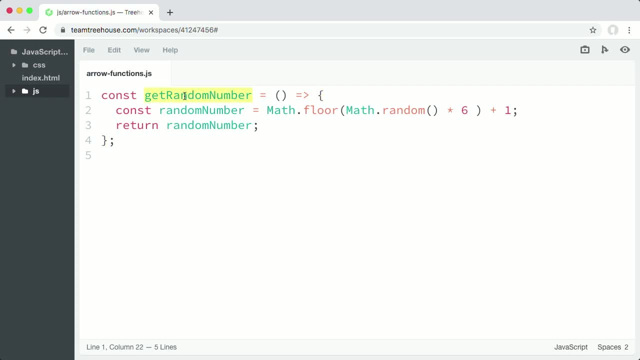 Alright. so now we've rewritten the function assigned to the getRandomNumber variable as an arrow function And notice how arrow functions themselves are anonymous functions because they don't have a name and you call or reference the function using the variable name. 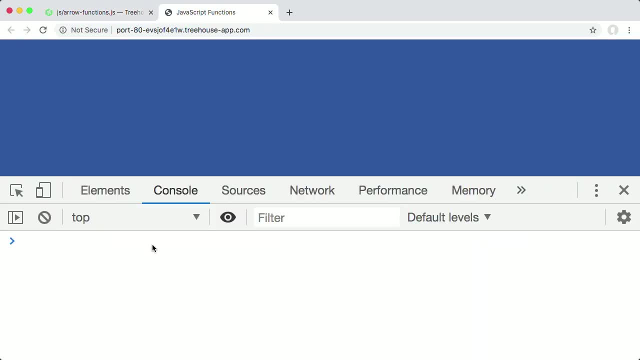 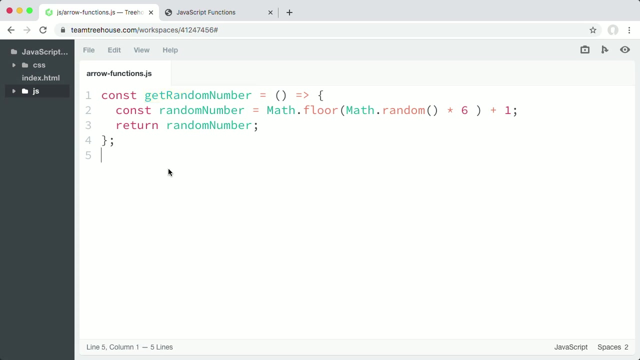 Let's test the function by calling it in the JavaScript console, And it works. We get a random number between 1 and 6.. Keep in mind that arrow functions mostly behave like function expressions. For example, arrow function expressions are not hoisted or lifted up to the top of their 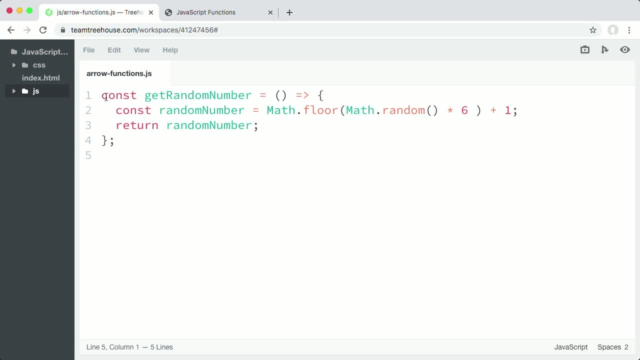 scope by the JavaScript engine. They load only when the JavaScript engine reaches the line of code they're on. So if you try to call an arrow function expression before it's defined, you'll get an error. Now, currently, this arrow function has no parameters. 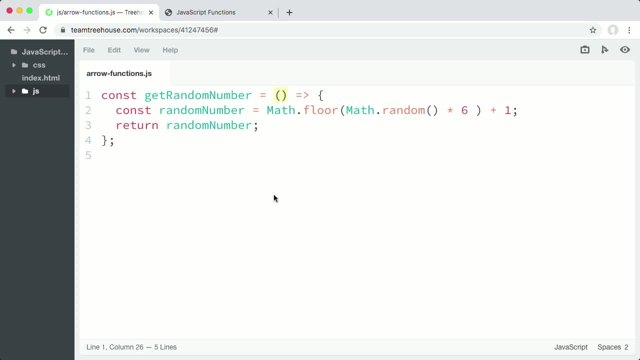 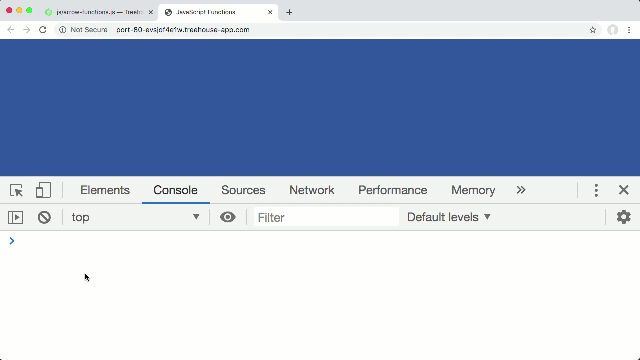 When you need to add parameters to the function definition, you include them, just as you do in function declarations and expressions. For example, add an upper parameter inside the parentheses, then use the value of the upper parameter inside the function. I'll save my file and test it in the console by calling getRandomNumber and passing it. 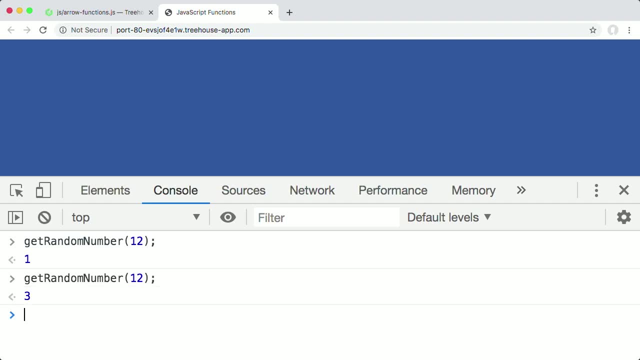 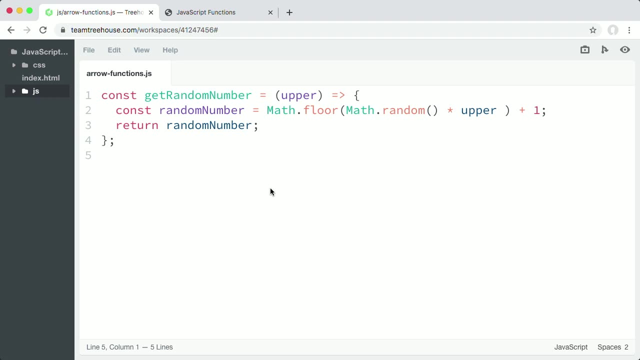 the argument 12, and there's my random number. Besides being concise, the arrow syntax has other benefits and helps solve common JavaScript problems and gotchas. Like other features, they have advantages and disadvantages which are beyond the scope of this course, but you'll get to know about them later, as you learn more and more about. 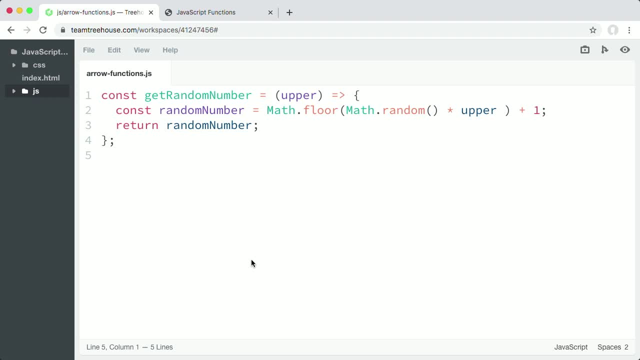 the details of JavaScript And keep in mind that arrow functions are not meant to replace regular function declarations or function expressions. It's just a newer syntax for writing functions. Function declarations, for example, are still widely used by developers. They're useful because they work in a slightly different way than arrow functions. 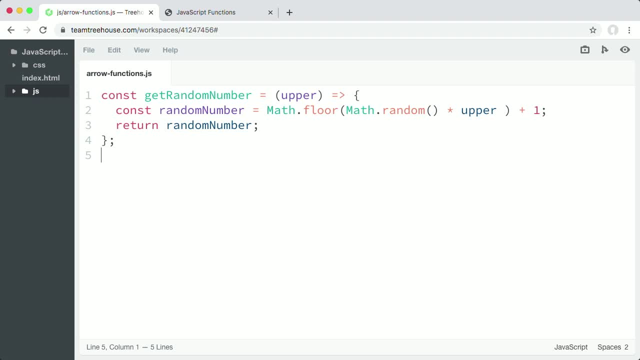 For instance, function declarations are hoisted, while arrow functions are not. There are specific places where arrow functions can improve your code too. For example, in future lessons you'll experience the advantages of the short arrow function syntax when you learn to pass functions as arguments to other functions with what are. 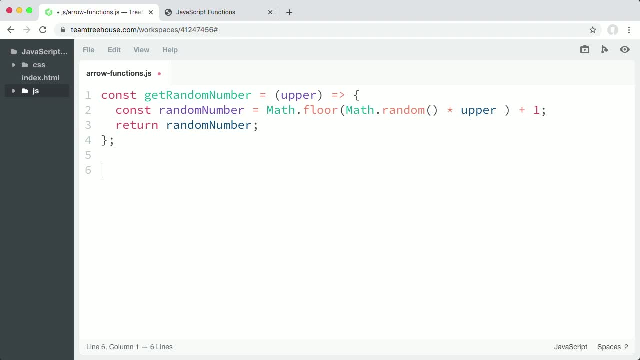 called callbacks. Alright, now to get additional practice writing arrow functions. I'll show you how to do that in just a few minutes. Why don't you rewrite this getAreaFunction declaration you wrote earlier as an arrow function expression? You can check out the solution in the teacher's notes with this video. 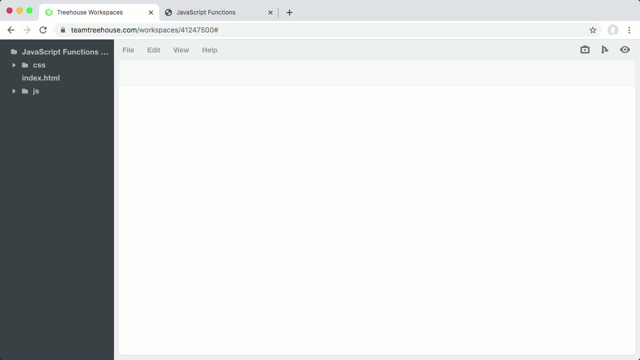 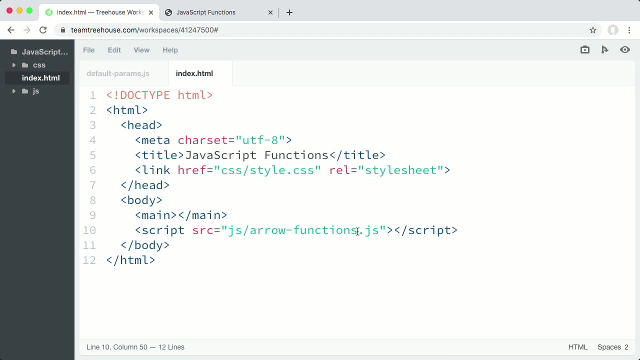 JavaScript lets you assign default values to your function parameters. That way, if, for any reason, you do not pass a certain argument to a function, the function uses or falls back to the default value. Open the file defaultParamsjs. Then update the script tag and indexhtml to point to default-paramsjs. 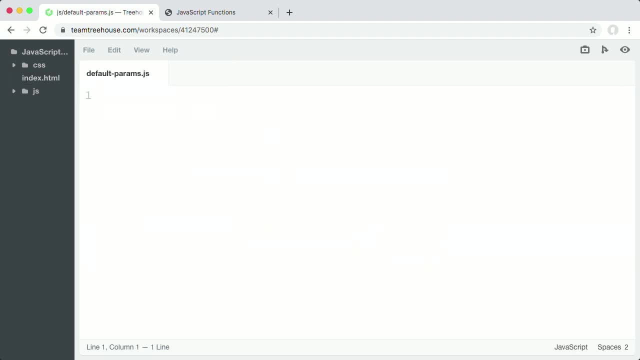 Let's first take a look at what happens when you don't pass an argument to a function that requires one. I'll define a function named sayGreeting that takes the parameter name. I'm writing this as a function declaration, but you can also write this as an arrow function. 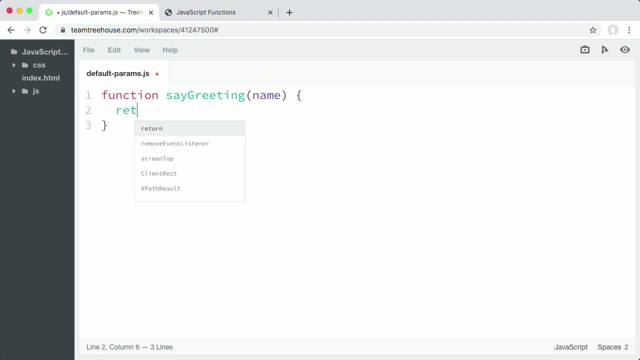 expression, if you'd like. The function should return a greeting using the value of the name parameter. I'm writing this as a function declaration, but you can also write this as an arrow function expression, if you'd like. I'll set it to return a string using a template literal with the message goodMorning followed. 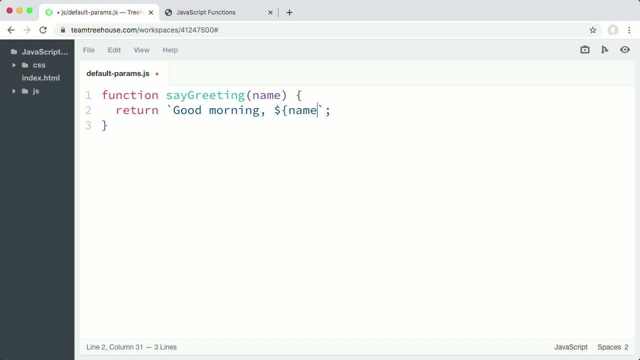 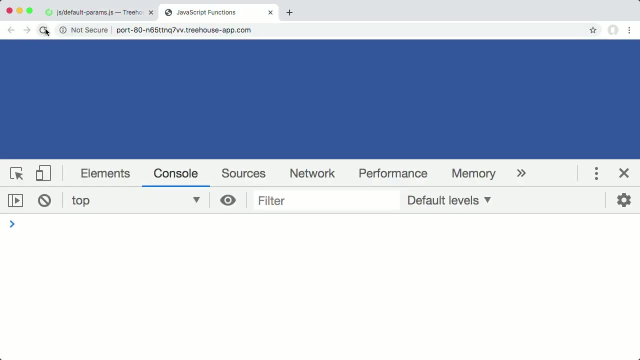 by the value of name. The function now expects a name value passed to it as an argument Over in the JavaScript console. let's see what happens. if you call the sayGreeting function without passing it a name argument, The console prints: goodMorning, undefined. 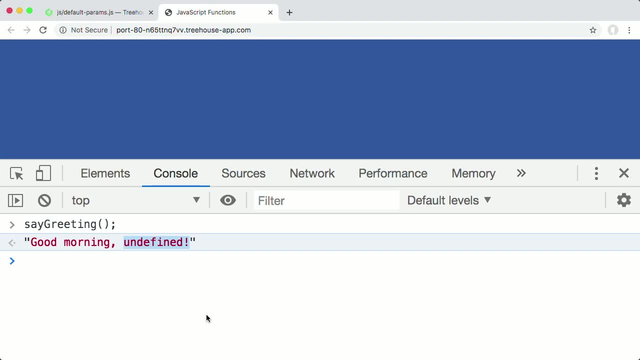 Undefined is one of JavaScript's built-in arguments. In this case, it means that there's no value assigned to the name parameter. It's undefined. In some cases, missing a function argument can break your entire program. To prevent any of that from happening, you can assign a default value to your parameters. 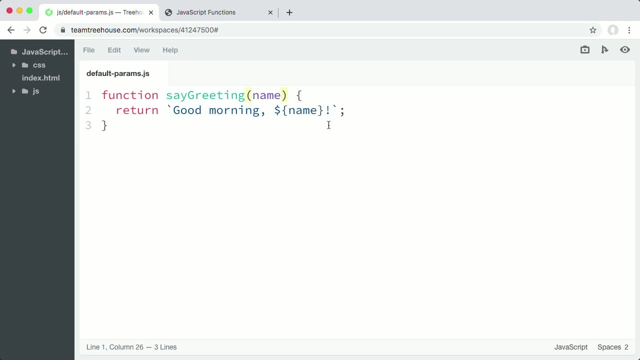 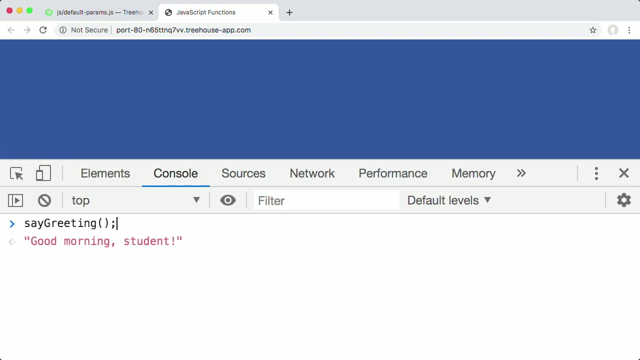 right inside the function definition. Let's assign the name parameter a default value using the equal sign or the assignment operator, and set it to the string student. I'll save the file And back in the console I'll once again call the sayGreeting function without passing it a name argument. 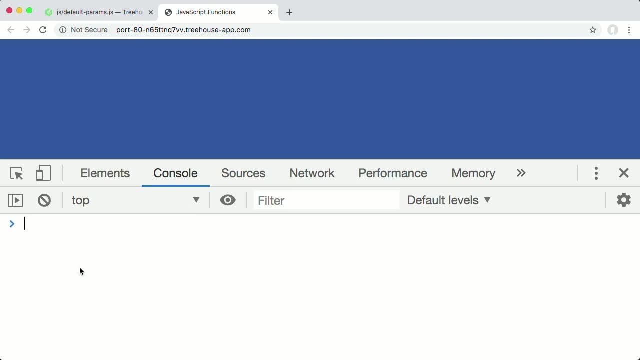 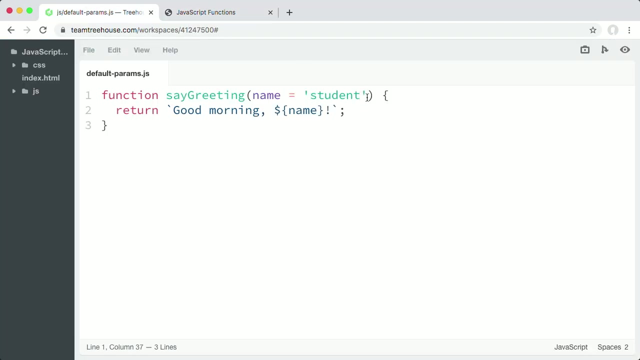 This time the console prints: goodMorning student. If you pass the function an argument Like the string Maria, Now the value Maria gets assigned to the name parameter And the function returns the greeting goodMorning Maria. Good, The default parameter acts as a fallback and safeguards your program from breaking or returning. 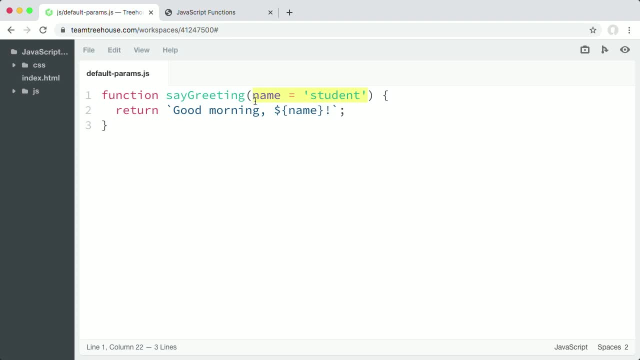 undefined. These work when you have multiple parameters in your function. I want to pass a custom greeting to the function instead of always displaying goodMorning, So I'll add a greeting parameter to the function definition, Then in the return statement replace goodMorning with the value that gets assigned to the greeting. 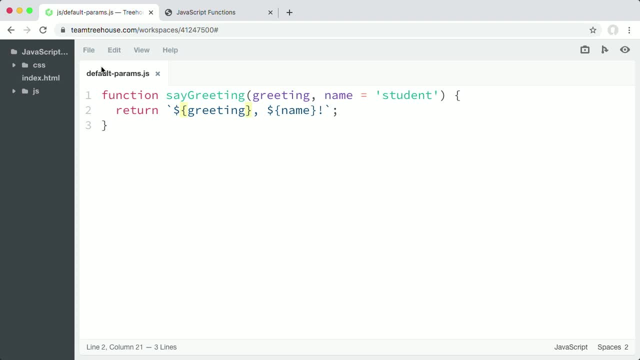 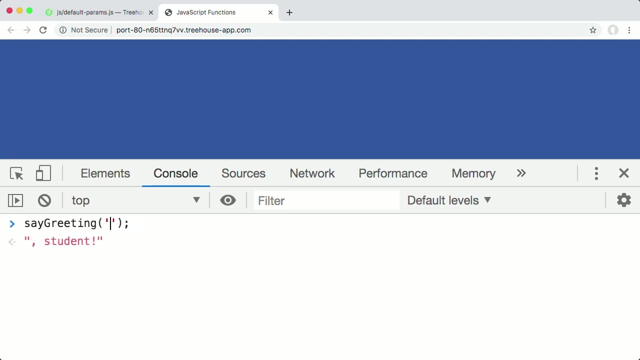 parameter. I'll save my file And over in the console I'll call the sayGreeting function, passing it a greeting argument only Good, Like hi there. The function returns hi there, student. Alright, now I'll assign a default value to the greeting parameter. 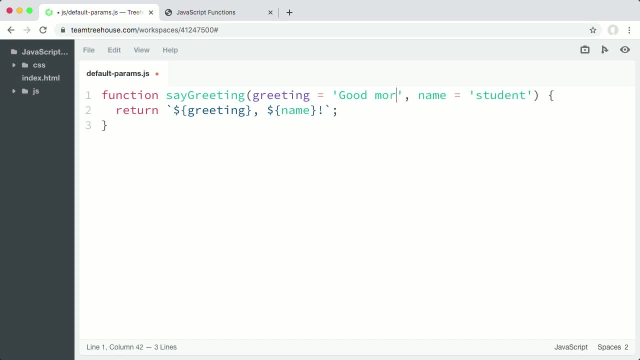 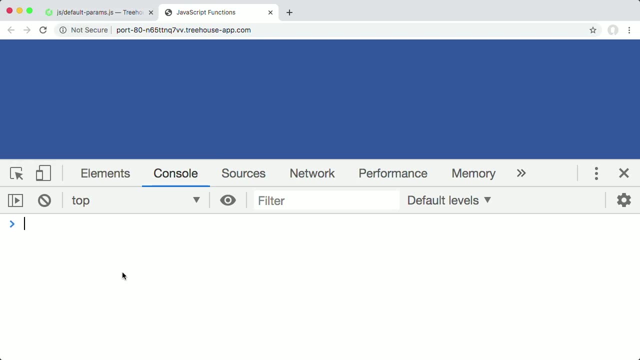 I'll set it to goodMorning. I'll test that this works by calling the sayGreeting function without passing it arguments, And it returns goodMorning student, The default greeting and name. But what if you want to pass the function a name argument only? 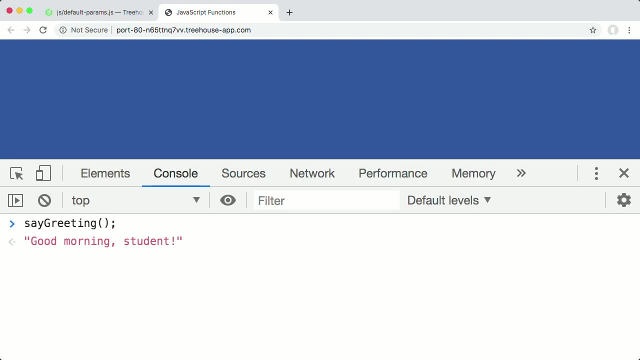 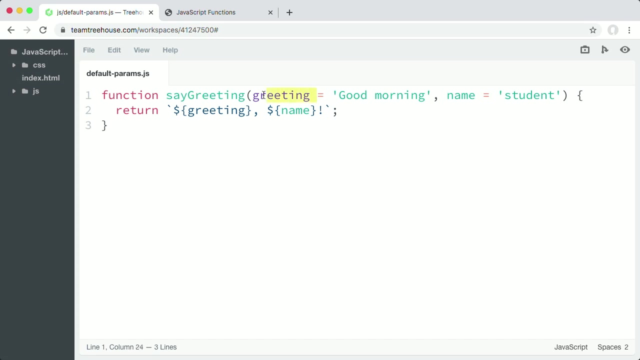 In other words, skip the greeting argument to use the default greeting and pass it just the name you want to display. Well, if you pass the function a name only, for example gil, it's going to return gil student. Since the function's first parameter is greeting, it's assigning the string gil to that parameter. 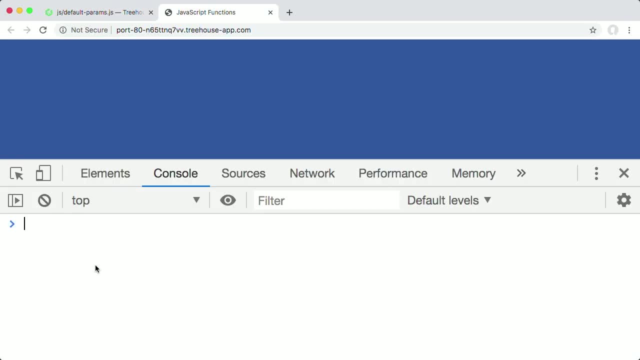 Now what if I just omit the argument? Well, if I just omit the function gil, it's going to return gil to that parameter. Well, if I just omit the function gil, it's going to return gil to that parameter. 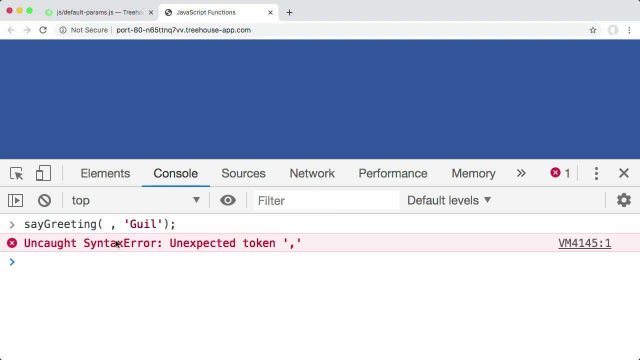 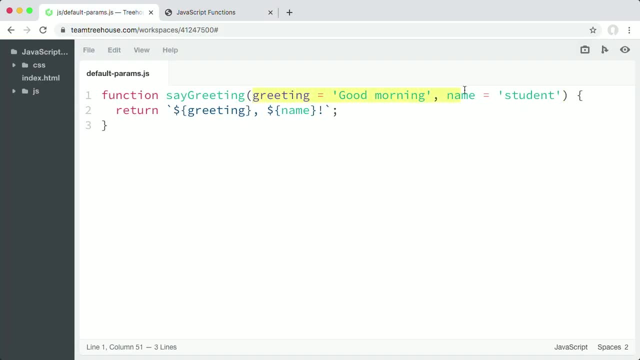 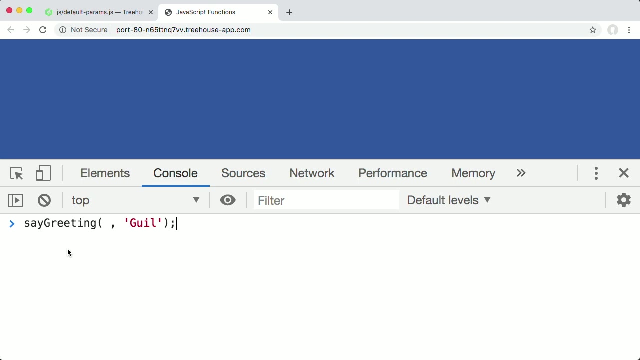 This breaks the function. JavaScript throws a syntax error. It says unexpectedToken comma. Even if you've assigned a default value to that first parameter, the function expects you to pass it a value. In this case, you need to pass the function undefined as the value for the greeting argument. 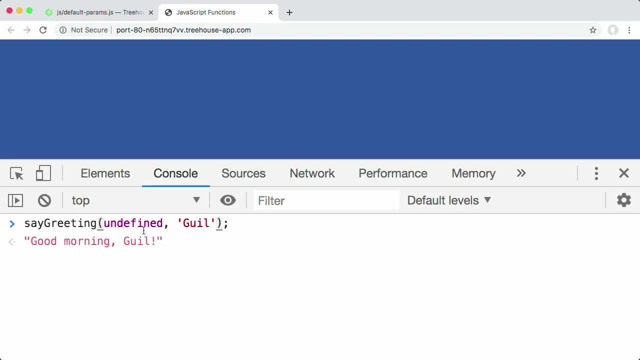 This instructs the JavaScript engine to use the default value assigned to the first parameter. It acts as a placeholder for the argument you want to skip Calling. the function now returns. good morning, gil. Perfect, And keep in mind that you only need to pass undefined for all but the last argument. 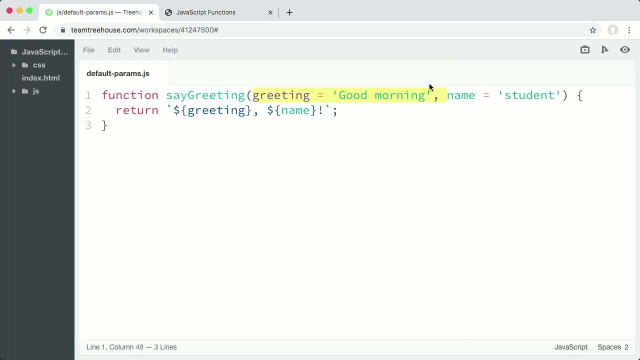 If the last argument is missing, the function will use the default value you set. Alright, now that you've learned how to work with default parameters, why don't you revisit the getArea function? You can copy this function snippet from the teacher's notes with this video. 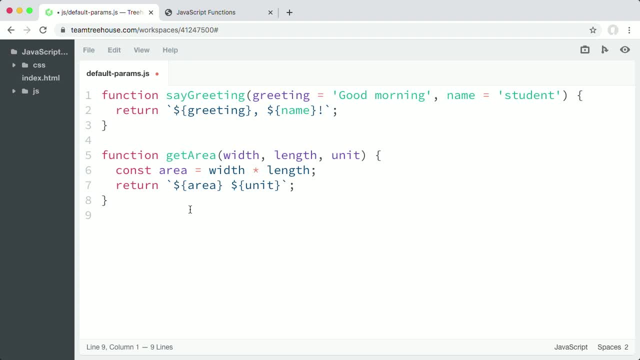 Let's say that, based on where your site visitors live, you'll want your function to display square feet or square meters. If most of your visitors are from the US, you will likely set the default to square feet. On the other hand, if most of your visitors are from Canada or Europe, for example, you'd 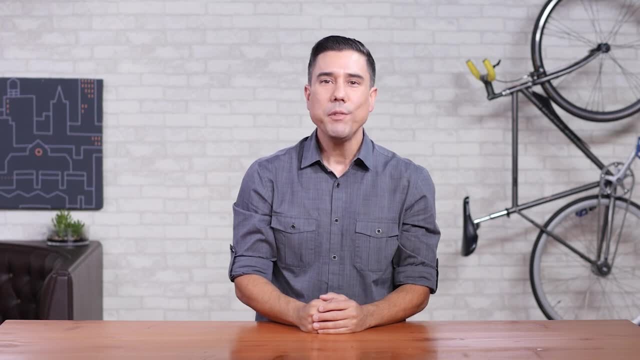 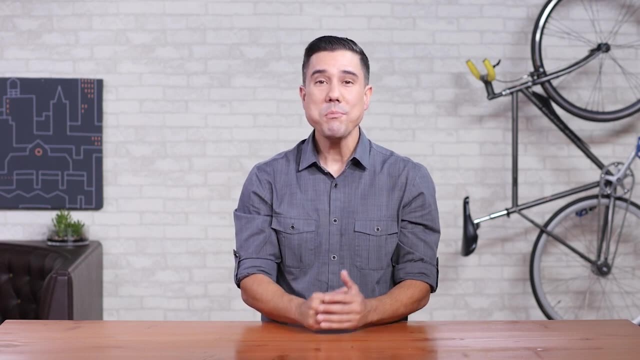 set it to square meters. Now that you've learned how to define and use functions, let's move on to the next part. I have a practice challenge for you. I'd like you to make the random number function you created earlier even more flexible. 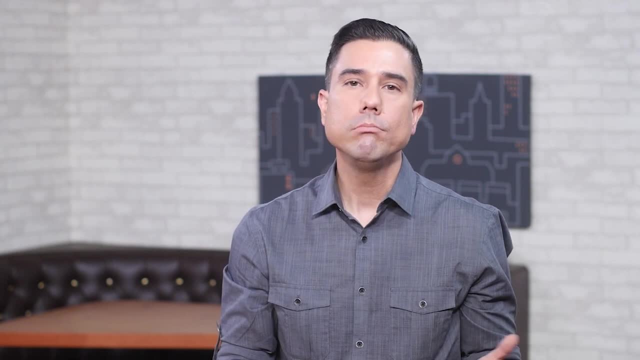 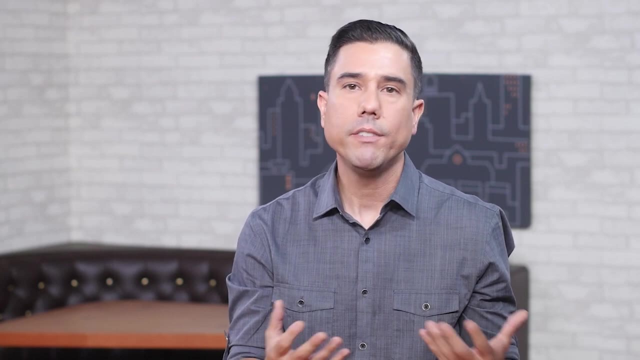 This time, the function needs to accept two values: a lower value and an upper value. In other words, the function should be able to produce random values between, say, 10 and 100, or 9 and 78, as well as between 1 and 6, or even 0 and 6.. 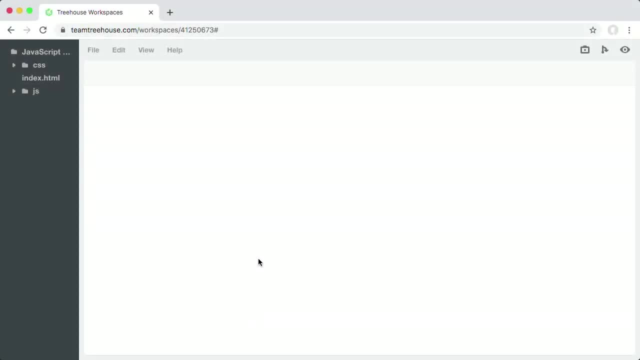 Let's go over the steps for this challenge. To get started with this challenge, launch the workspace with this video and open the file randomjs. In the file, I've included a comment that provides a high-level overview of the components of the function you'll need to create. 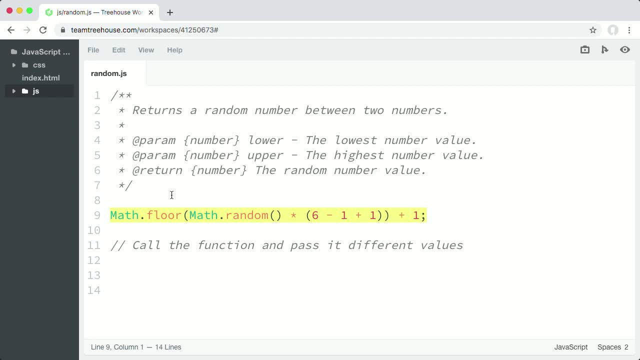 I also provided the formula or logic for creating a random value between two numbers, 1 and 6.. This should look familiar. You used this in a previous course on JavaScript numbers. Now you're going to use this as the basis for creating the function for this challenge. 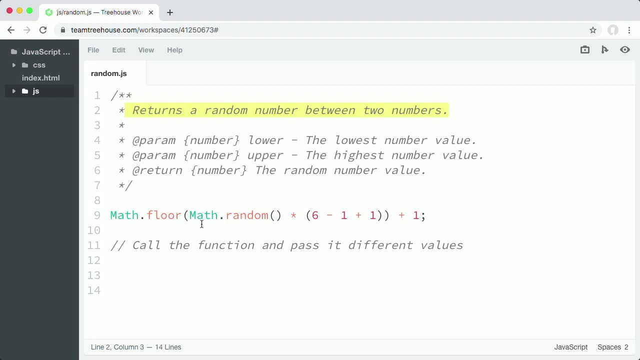 Your function should be able to produce random values between, say, 10 and 100, or 9 and 78. As well as between 1 and 6, or even 0 and 6.. Once you're done writing the function, make sure you test it by calling it and passing. 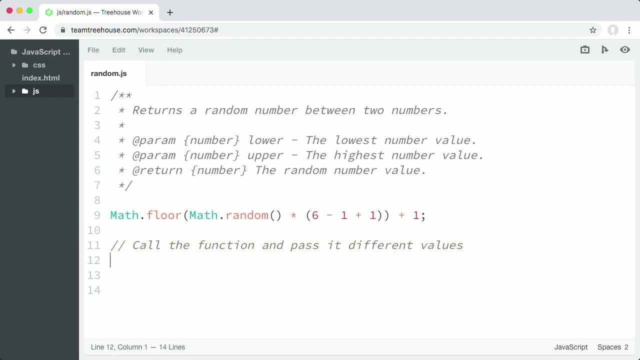 it different values. You can display the values in any way you choose, for example in a console with consolelog, in an alert dialog or on the page, using some of the techniques you've learned so far. So good luck, and in the next video I'll show you my solution. 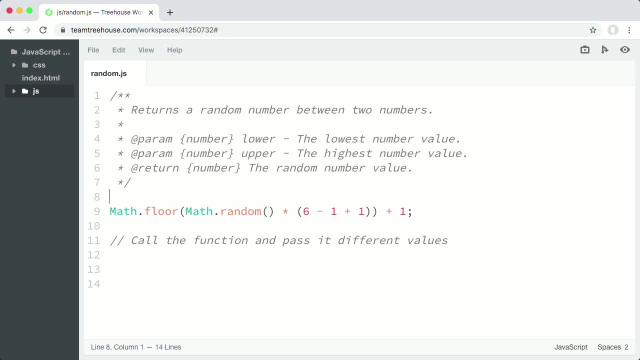 Alright, now I'll walk you through how I would write the random number function. You learned how to create a random number between two values in a previous course. The difference is that now you're using a function that accepts arguments. For starters, I'll create a function named getRandomNumber. 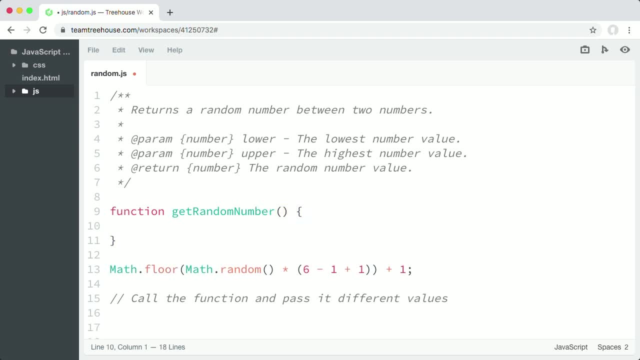 I'm using a function declaration, but you could have written this as a function expression or as an arrow function. The function should produce a random number value between two numbers. so I need to add two parameters to the function. I'll call them lower and upper. 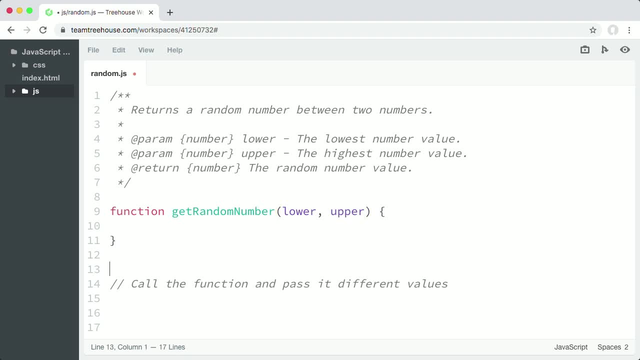 Next I'll move the randomNumber function to getRandomNumber. I'll put the randomNumber code into the function and place the parameters where they need to go. The upper value goes here and the lower value should go here and here. I'll assign the result to a variable named randomNumber, then return the value of randomNumber. 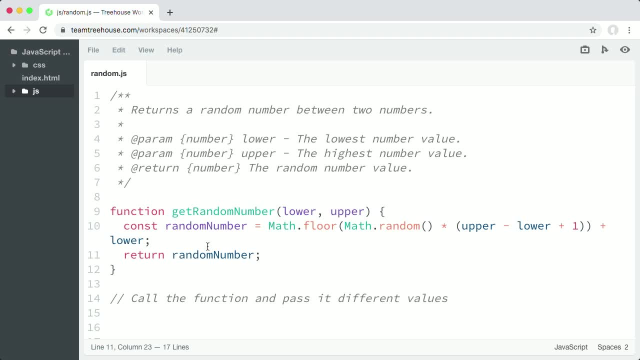 You could make this code even more compact. You don't need to assign the formula to a variable and then return the variable, Because the randomNumber generating code produces a value. you can return its result like this. Let's look at why we can do this. 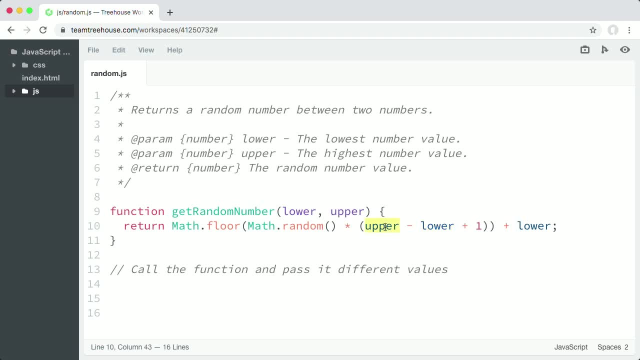 This code accepts information, the lower and upper values, and runs it through a couple of JavaScript methods. It does some math. All of this code evaluates, as programmers say, to a single value, a random number. All a return statement does is return a value. 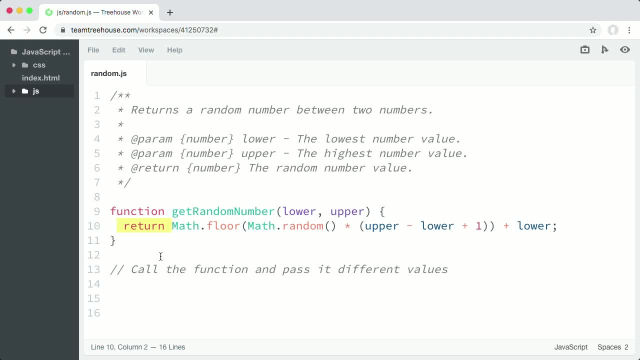 It doesn't matter where that value comes from. It can be stored in a variable, or it can be the result of another function or a mathematical operation, as it is in this case. Alright, now to test this, I'll call the function a few times and print the results to the console. 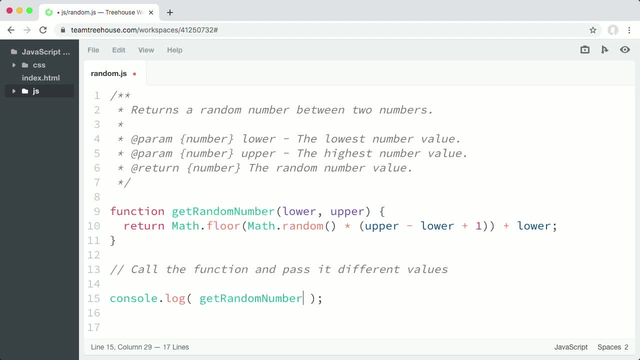 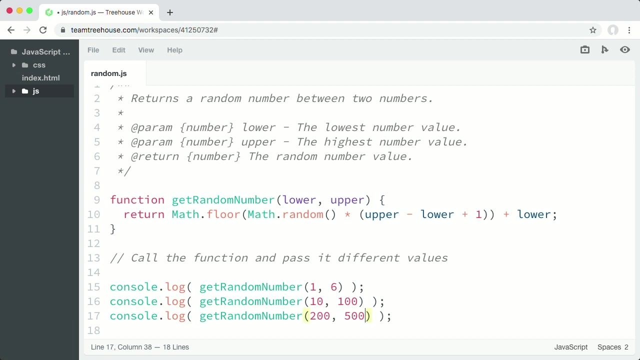 First I'll call getRandomNumber, passing it the values 1 and 6.. Below that, I'll call getRandomNumber again, this time passing it 10 and 100.. And I'll call getRandomNumber a third time, passing it the values 200 and 500. 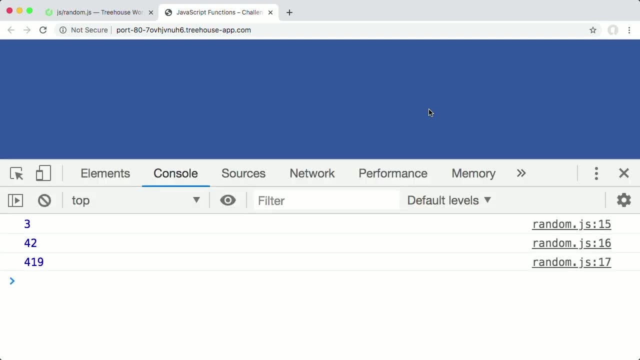 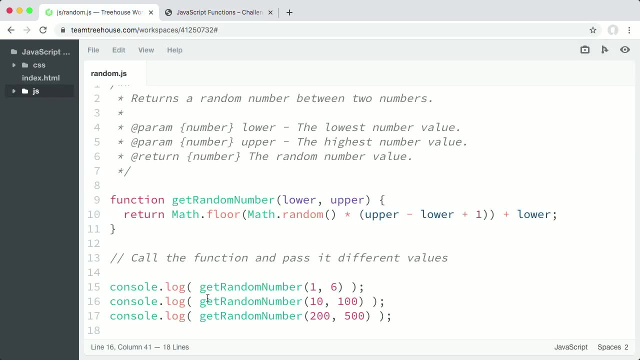 I'll save my file and over in the console I get 3.5.. Three random numbers: good. So now I can use my random number function in all sorts of ways, For example display it in a message like this: 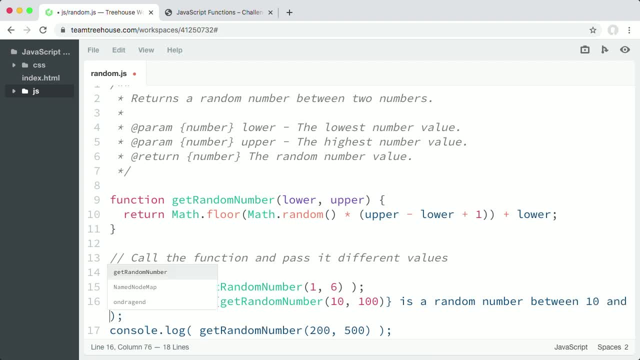 Remember, in a template literal, you can include any JavaScript expression between the dollar sign and curly braces And its value will be inserted into the string. By expression I mean any code that evaluates to a single value, like a variable math operation. 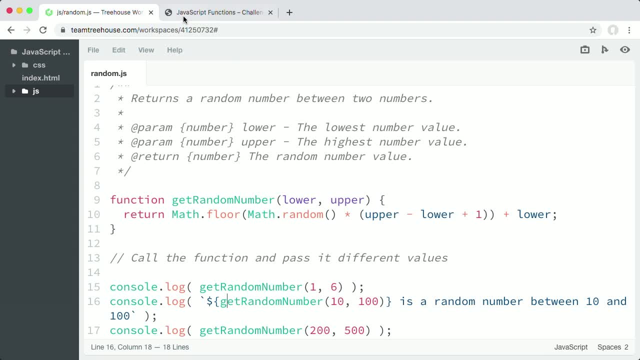 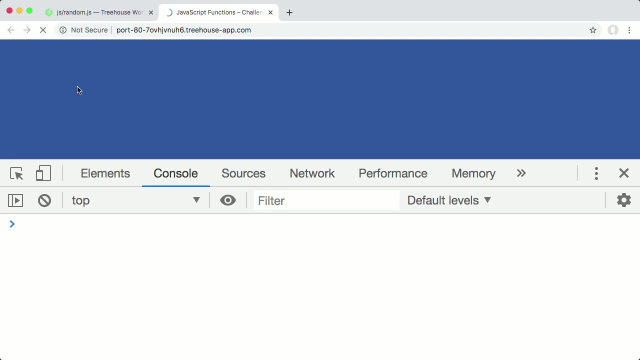 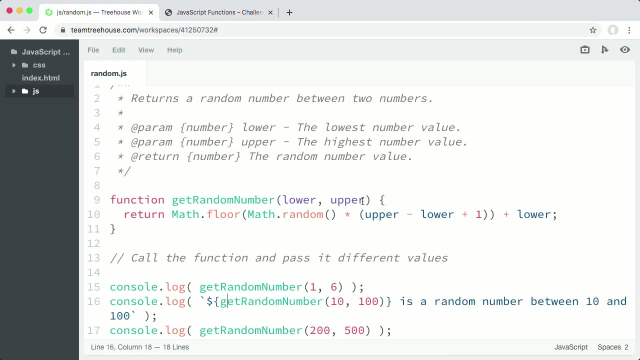 or in this case, a call to a function. In the console we see the message. 41 is a random number between 10 and 100.. You might have added a default parameter to your function too. For example, set the upper parameter to a default value of 100.. 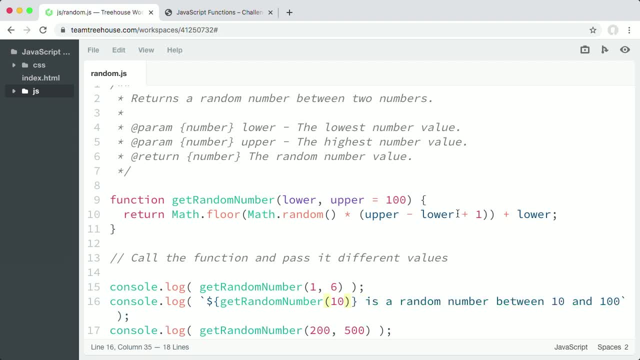 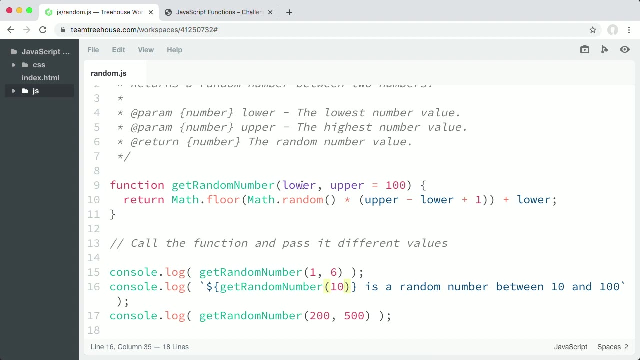 The function will change such that the number that it is going to call by is the same as the one you entered earlier. The function will probably need some more data, but if you want some more data, you can use the function instead, And that's it. 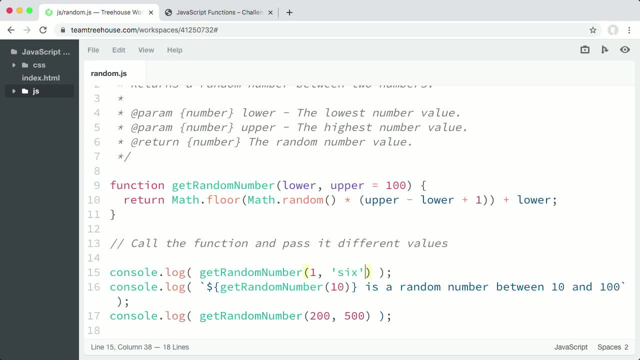 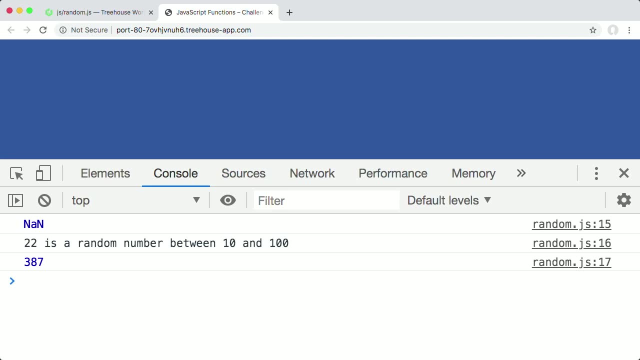 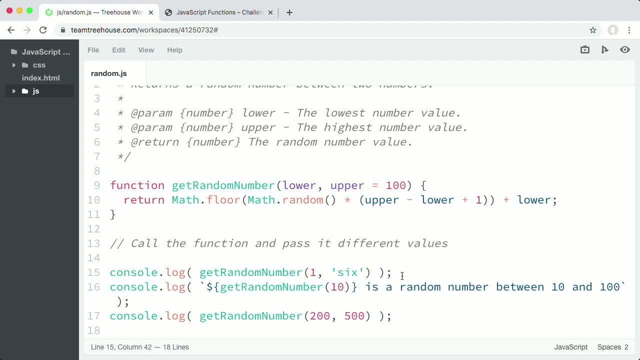 then coming up with a plan to handle those problems. To fix this, we can use an if statement to make sure that both arguments are numbers and then display an error if one or both of the values are not numbers. In the next video we'll implement the solution. 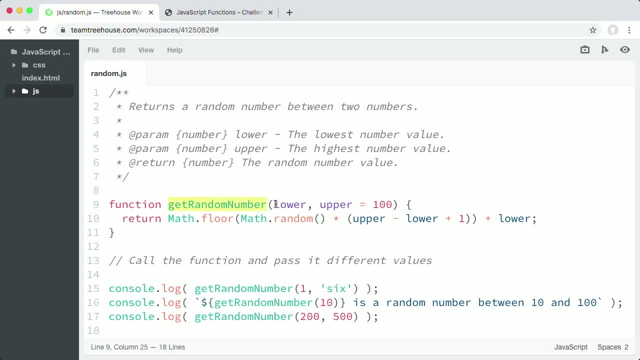 Now we need to make sure that the getRandomNumber function receives two numeric values as arguments and no other type of values. If the function is called with a string, for example, then the program should display a custom error message Inside the function. add an if statement just above the return statement. 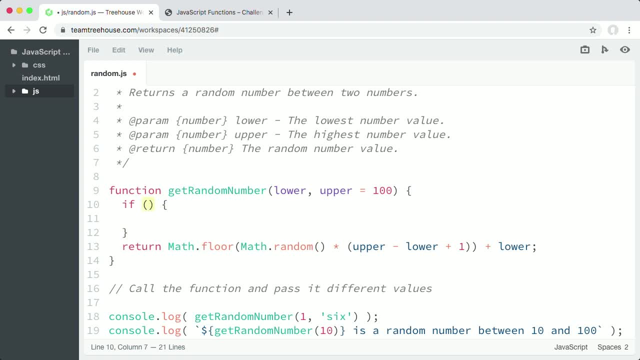 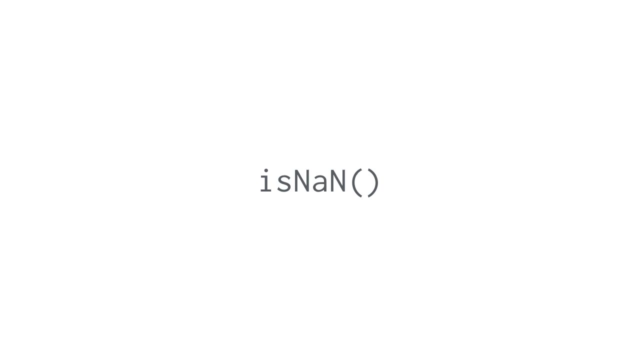 But what should we test here? Well, we need to make sure that the two arguments passed to the function are numbers. There's a few ways we might do this. I'll teach you a new method for testing number values. JavaScript provides a special function called isNan or isNotANumber. that takes one argument. 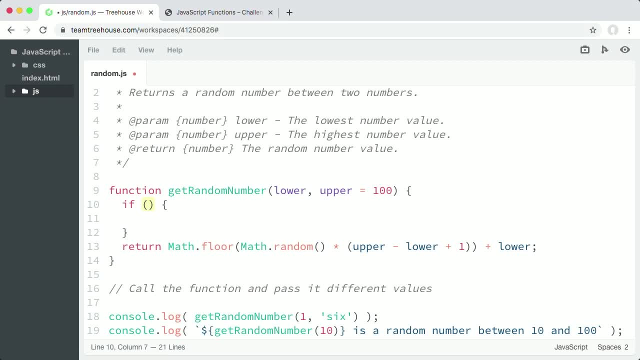 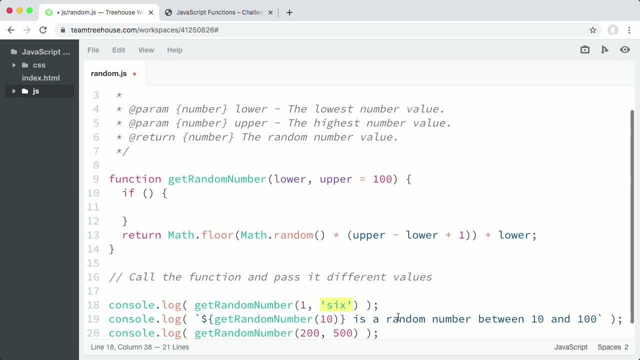 and returns a boolean value. It returns true if the value is not a number and false if it is. For example, if you pass the string 6 to the function, you get the value true. However, if you pass a number like 6 to the function, you get false. 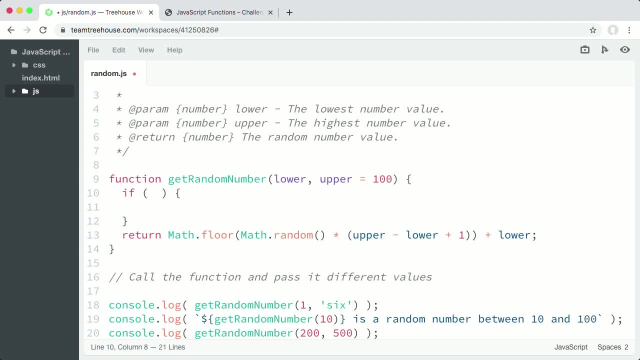 So in the if statement I'll first test that the lower argument passed to the function is a number like 6.. In other words, if the lower value is not a number, then the code block with this if statement will run. But we want to test both arguments. 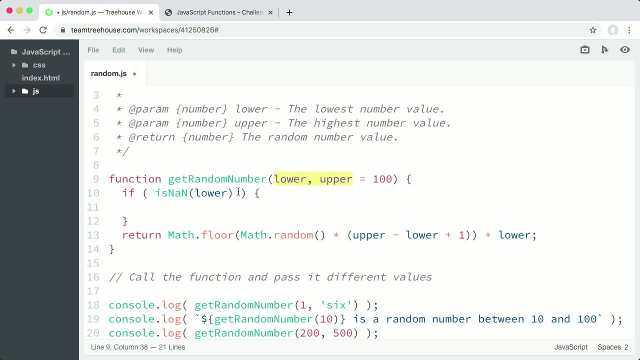 If either is not a number, then we'll display an error. To test both, you can use the logical or operator by typing two pipe characters. then add a test for the upper argument like this: Now, if either argument is not a number, we can display a custom error. 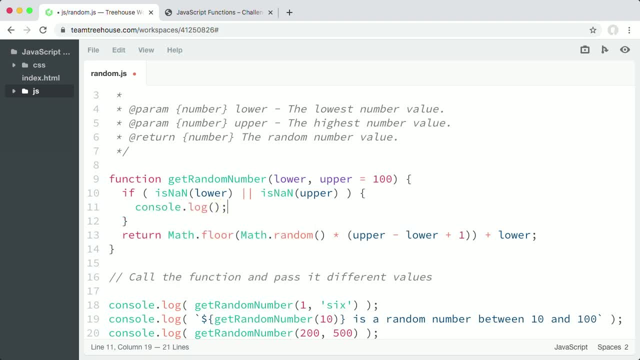 We could maybe use consolelog to display a message in the console. like both arguments must be numbers In this case, it's probably best to throw a custom error so the programmer can immediately see that they've used the function incorrectly. JavaScript lets you create your own errors. 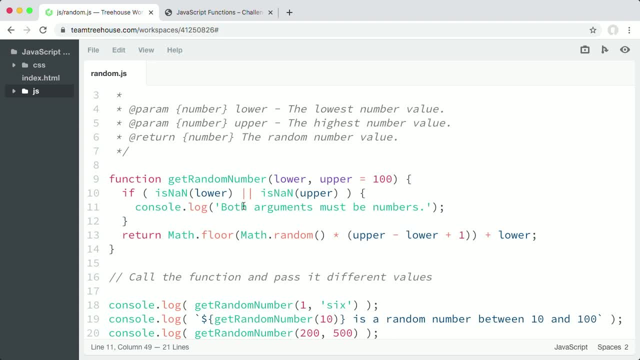 Which print directly to the JavaScript console, just like regular syntax errors do. It looks like this: The throw keyword followed by JavaScript's error object. This is a built-in keyword and object. JavaScript provides to create a custom error or, as developers say, throw an exception. 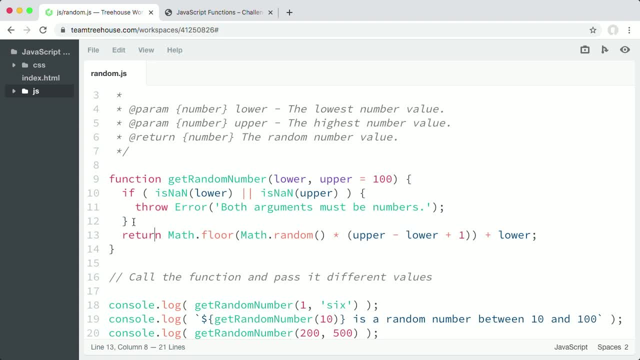 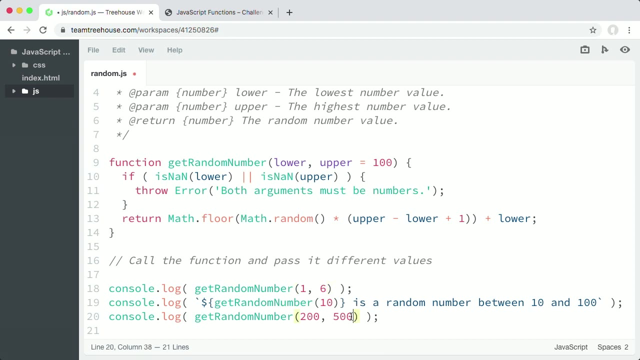 Since it's inside the if statement, the error is thrown only when the function receives anything but a number for either argument. Alright, Now I'll test the latest changes by calling the function correctly with numbers a couple of times, then call it with a string value like 300. 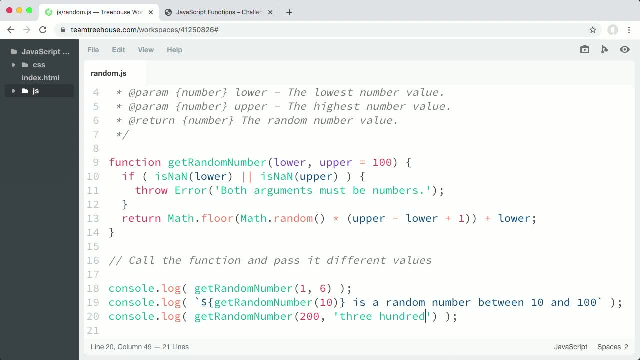 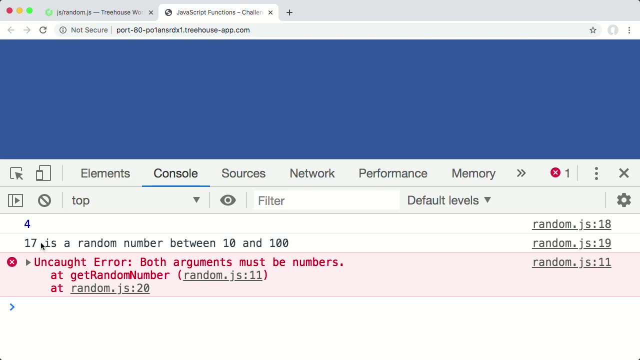 I'll save the file And over in the console I get two random numbers, 4 and 17.. And below them is the uncaught error displaying my custom error message. both arguments must be numbers. Notice how it looks just like a regular error thrown by the JavaScript engine.